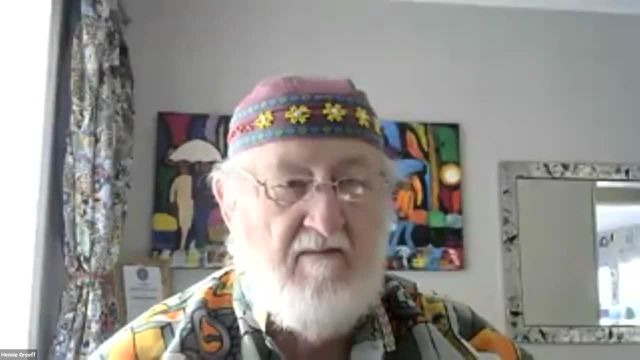 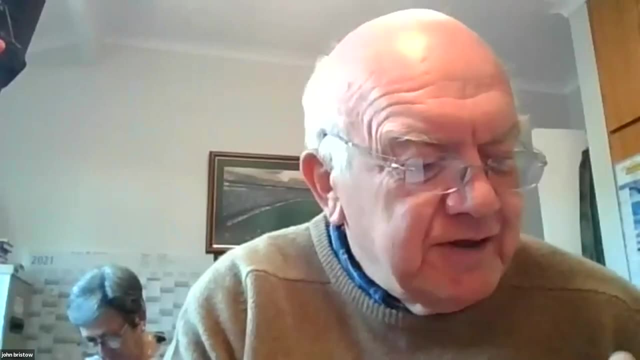 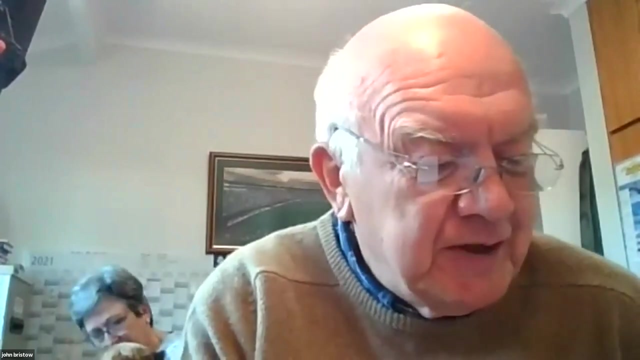 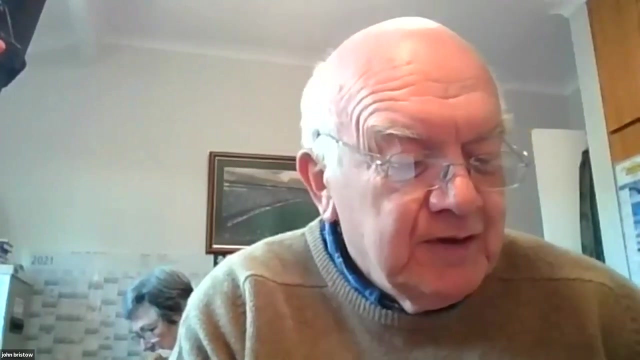 Thanks, Henny and good morning everyone, and thanks again for the very good turnout. I'd like to introduce Stephen Davey. Stephen graduated with the BSc Geology and a BSc Honours here at UCT in the Cape and started his career in the old rocks, Barberton, Greenstone Belt, with Anglo-Vile exploration and then gradually moved through geological time, he says, to the Bushfeld Complex with a. 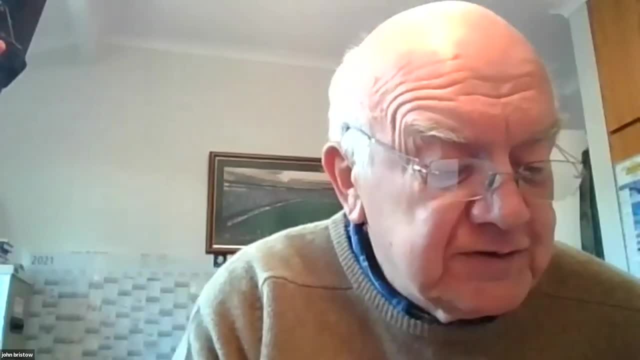 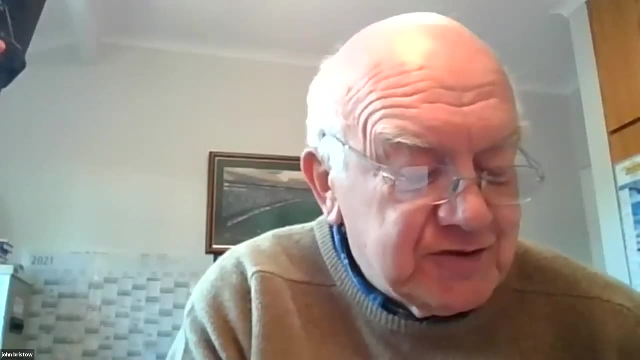 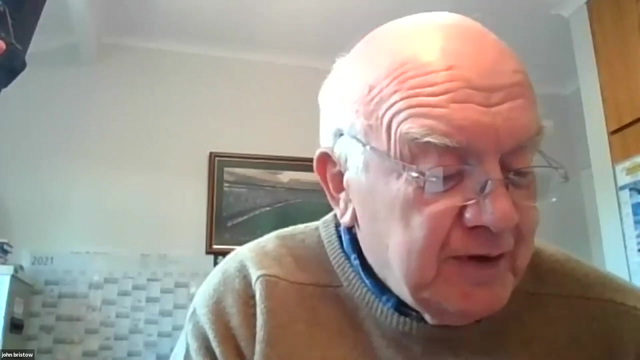 parlor and then Mises, Oak and Tertiary Rocks in Argentina and Ecuador with Gencor and Billiton. He then ran out of geological time in 1999 when the Gagu Pinchecha volcano that overlooks Quito and Ecuador erupted, and he sent me a gorgeous picture looking out of his 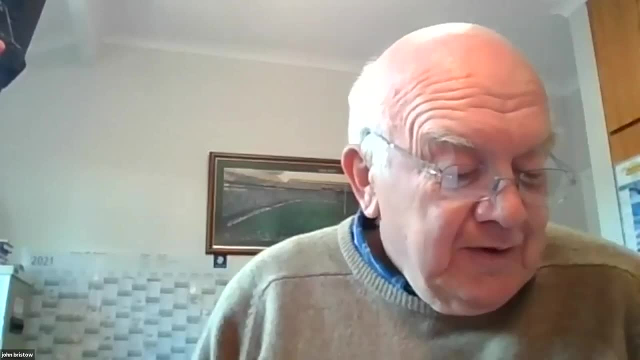 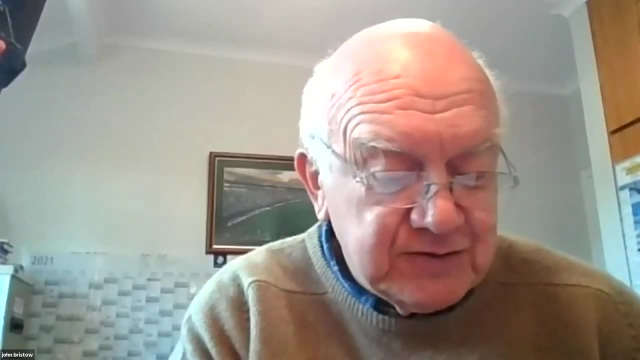 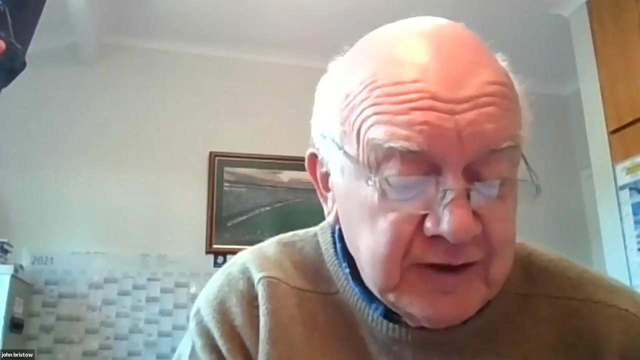 front balcony at this erupting volcano. Like many of us, he also had a mid-career crisis, or transition, as he calls it, and came back to Cape Town to do the Masters of Environmental Management from there, worked for the City of Cape Town and the Bananvoto. 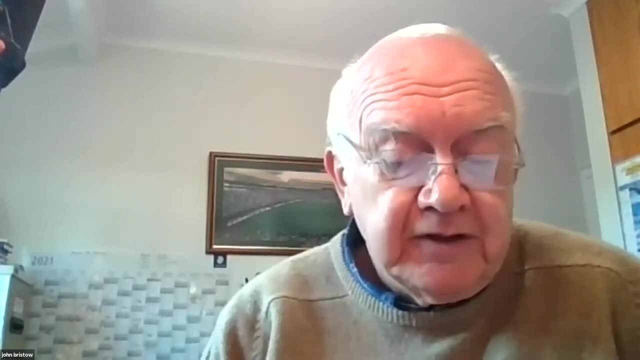 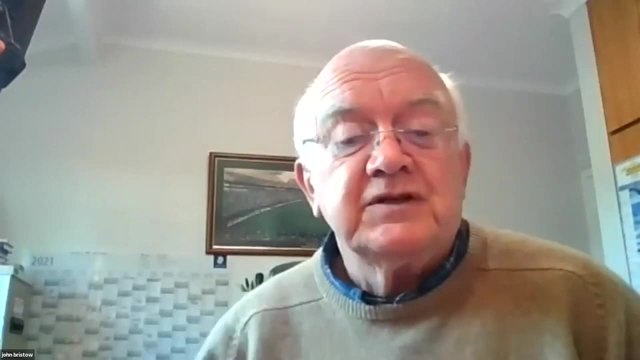 and then discovered that there are actually quite a few mines- mostly industrial mineral deposits- being mined here in the Western Cape, and he's going to talk to us about that today and he's also very up to speed with a lot of our legislation and can tell us, you know, how and why. 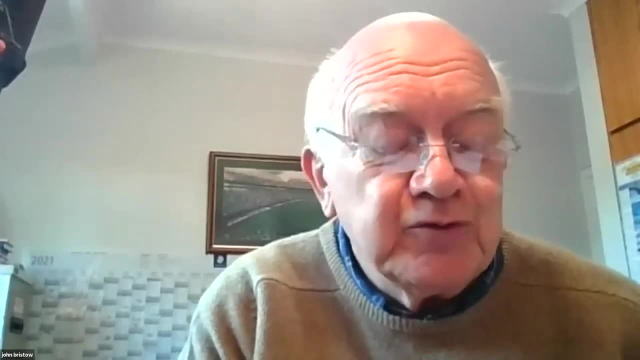 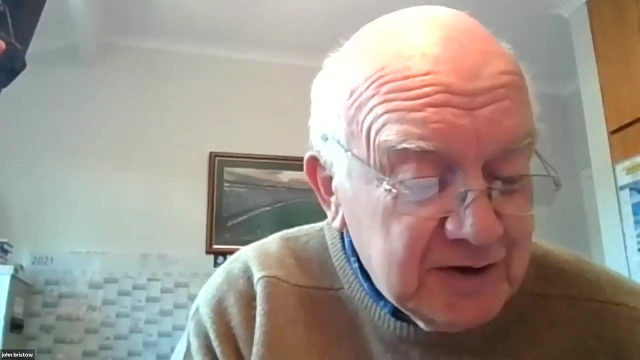 certain permitting processes and other processes don't work, and I think Henny and Peter, for NECIRC, are both on the talk today, very interested to hear about that, given their challenges with cutting reeds and the onrush estuary. Thanks, Stephen, look forward to your talk. 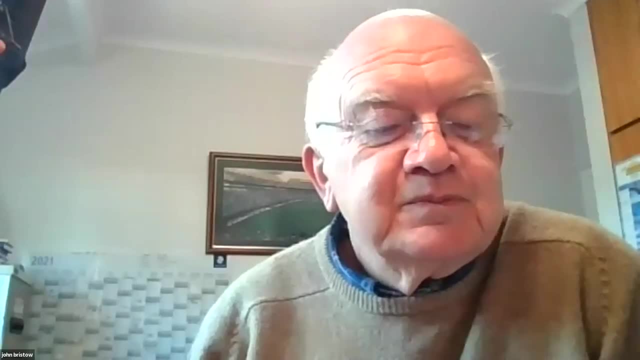 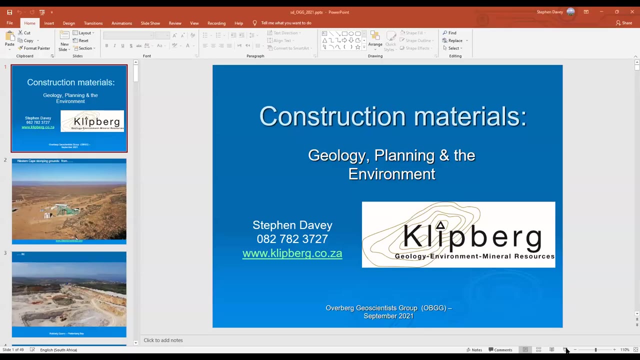 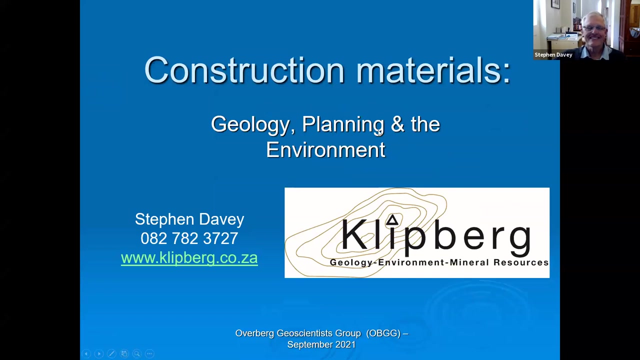 Okay, let me just try and share my screen first. Right, is that fine? can everybody see that now? Yeah, you're good to go. Okay, thank you very much everybody for attending this talk, Maybe just as a follow-up from last week's talk about the usefulness of the old material when I got back into mining, which 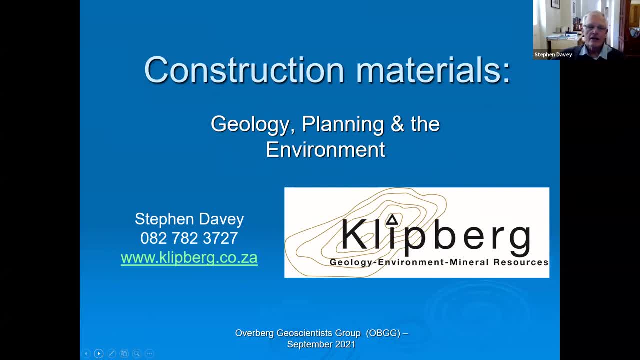 I never actually expected. in the Western Cape the first thing you do is you go to your local geological survey or council for geoscience and there I was really very well helped by Dr Doug Cole. Every question that I asked he was always very helpful, provided me information, access to reports and so on. So I 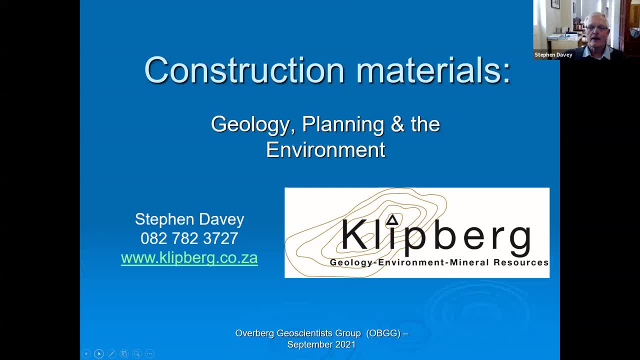 sort of went on a bit of a rediscovery of my own province, and thanks to the council for geoscience for all the information that they gave me, I also learned a lot more about mining than I ever expected, being involved with mining permit applications, mining right applications, 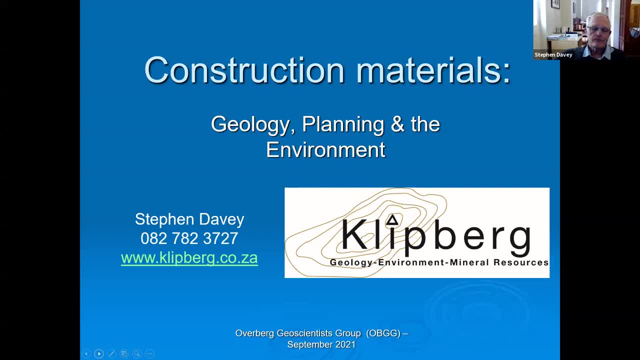 section 102 applications: prospecting applications, assisting people to object to mining applications- all these things that I never actually expected When I came back to the Western Cape I thought I might not ever see a mine again, but it's very interesting actually in the Western Cape. 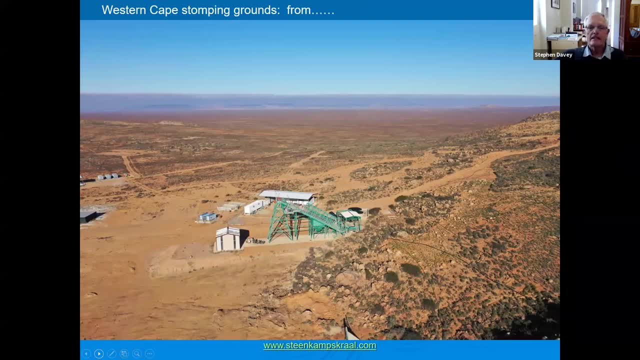 So my new stomping grounds stretch from right up the West Coast almost in the Northern Cape. This is not construction material. this is the Steenkampskral Monazite mine- rare earths mine, and people have been asking a few questions, I think in the previous two weeks, about Steenkampskral. 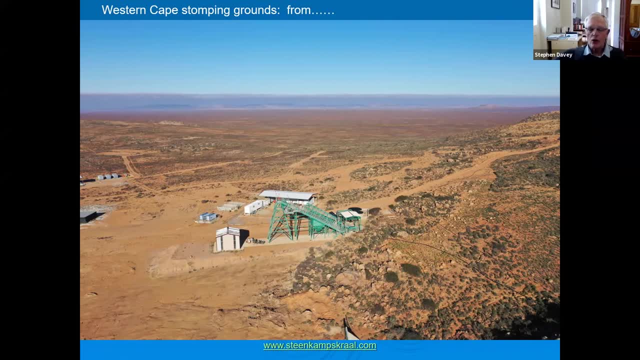 They've got a very up-to-date website. so you know I'm not going to talk about it, but I'll just advise people. just look at the website. I think there's a YouTube video on it, if you know of anybody that wants to invest in rare earth minerals. 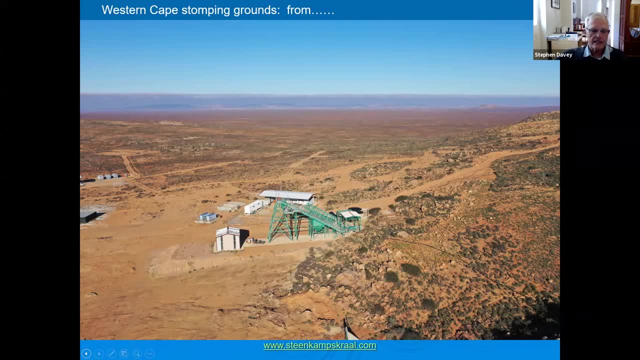 I think they are looking for investors. so that's Steenkampskral. Then I go as far east, almost to the Eastern Cape. this is the Robber Quarry in Blettonburg Bay, and in fact it's very close to the turnover of the. 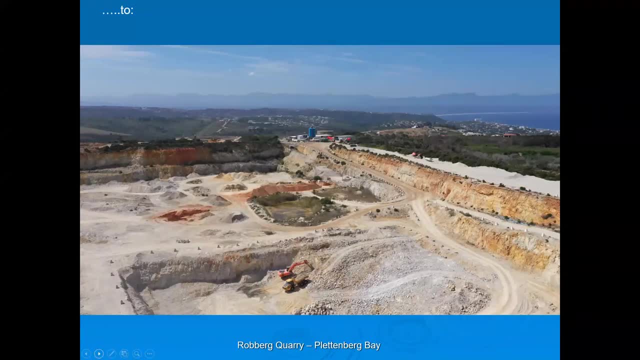 Amundsen Mine. This is the Robber Quarry in Blettonburg Bay and in fact it's very close to the turnover of the Amundsen Mine. This is the Robber Quarry in Blettonburg Bay and in fact it's very close to the turnover of the. 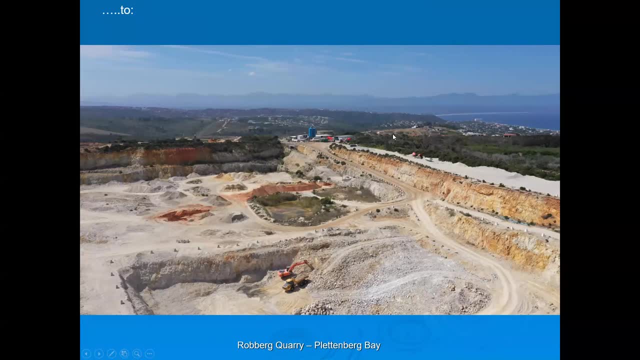 the turn off to the Robberg Peninsula Nature Reserve, But people don't really notice it because it's got very well constructed berms. It's tucked away on top of the hill. The quarry is mining table, mountain group sandstone and quartzite. 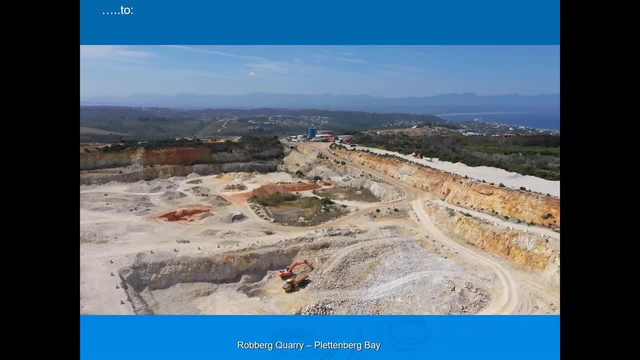 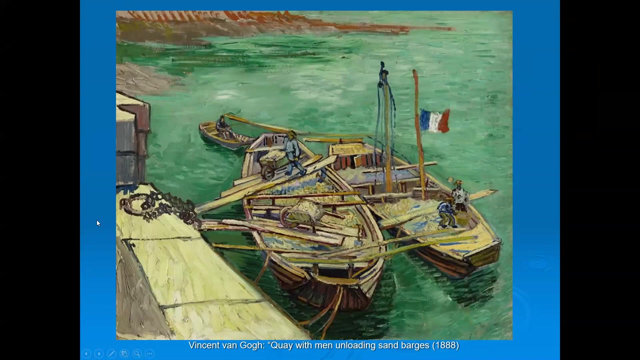 and it's probably the best aggregate anywhere along the garden route. So this is just a picture, just to illustrate that when you build something, the building material is not always right where you expect it. And here's a picture from Vincent van Gogh. 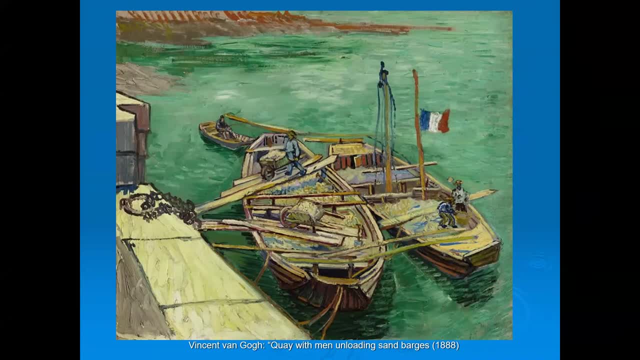 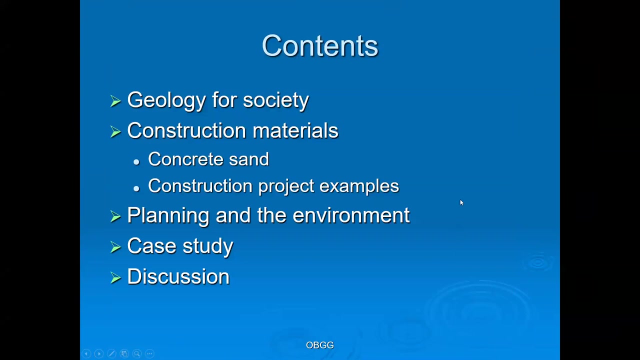 And obviously they needed sand somewhere and they didn't have the sand where they needed it. So here they are, unloading sand off sandbar sandbars. So my talk is not going to be a very technical talk, and these are the kind of topics that I would love to try and cover. 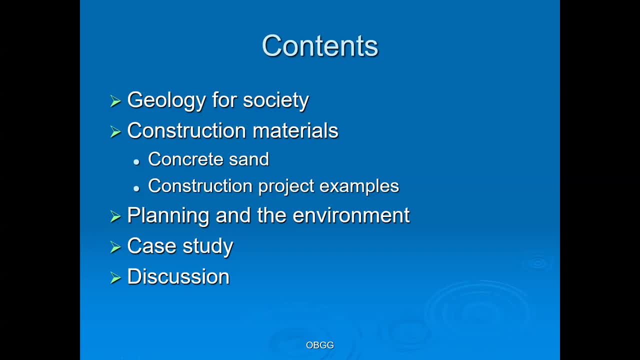 And I believe that geologists have got a lot more to contribute to the environment and to planning and sort of really appreciate it. And we're going to be looking at some aspects of construction materials in the Western Cape And then how planners look at the Western Cape. 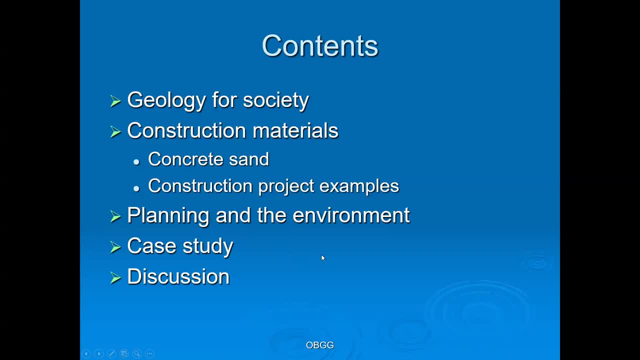 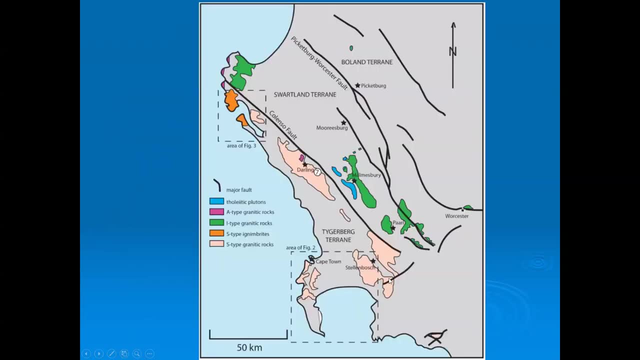 and a little bit of a case study and then maybe some room for some discussion afterwards. So here's a picture just to illustrate where I live in Darling, And it follows up from some of our previous talks with a little bit of a West Coast influence. 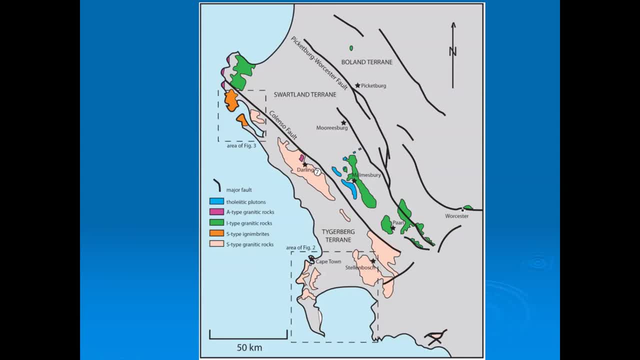 This comes from the field guide before the IGC Congress in 2016 from Stellenbosch University. Geologists have done a lot of work on Cape Granites And there's Darling and the little red A-type granite rocks is a little copy outside Darling that I thought was quite handy. 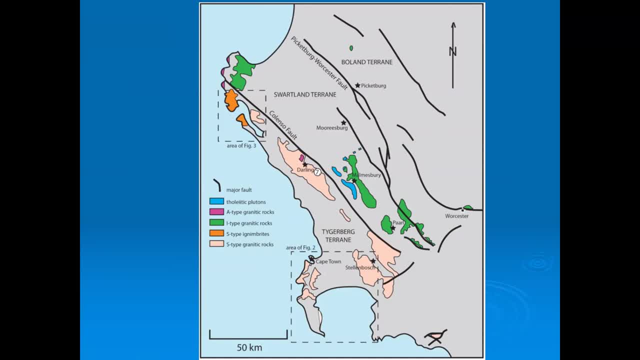 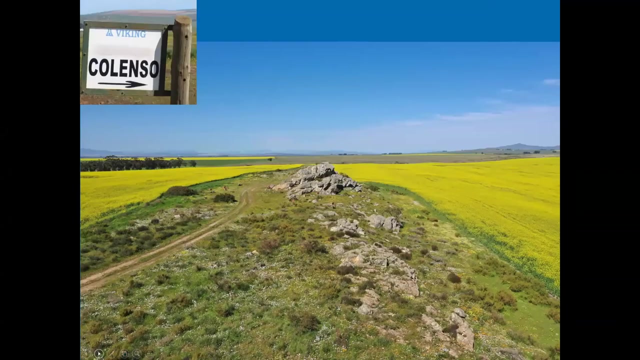 to use for the name of my consultancy, Klippburg. And also here's the Colenso Fort that previous speakers have spoken about, which subdivides the Tigerberg terrain And the Swartland terrain in the Malmesbury group. People haven't often seen what the Colenso Fort looks like. 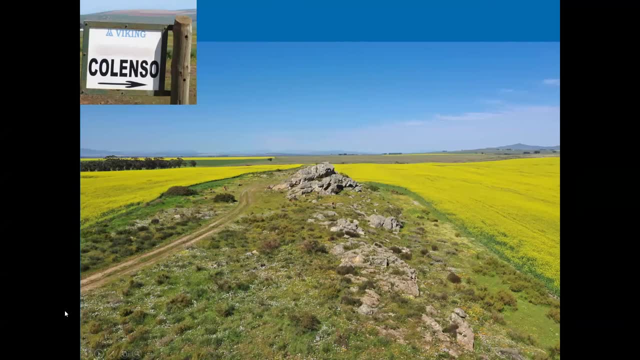 So I went out last week and took a few photographs. This is in the fields just to the north of Darling, One of the few outcrops where the Colenso Fort can be seen, Surrounded by flowers And fields of canola. 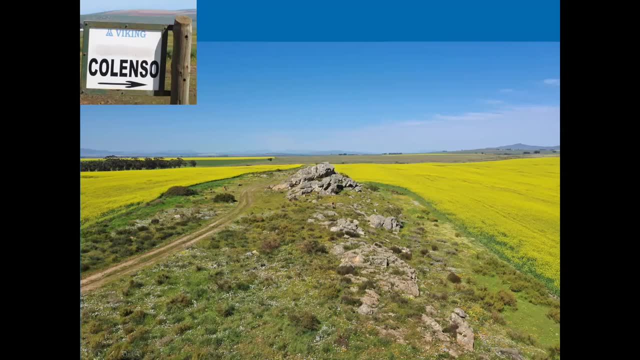 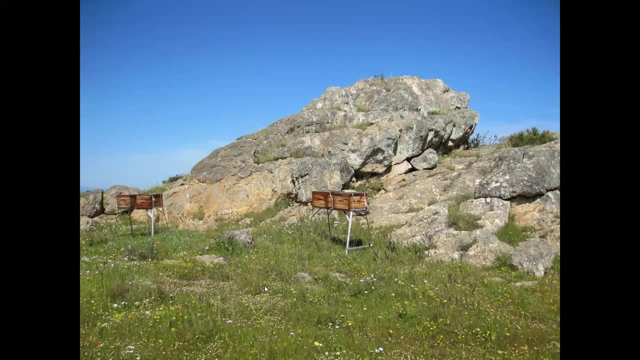 You probably see all the bee boxes all around the outcrop as well. I tried to get a little bit closer, but not too close, Because my drone, I think, had stirred the bees up a little bit and they were getting a little bit aggro. 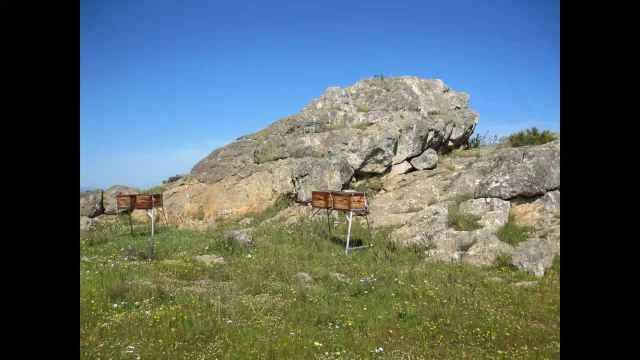 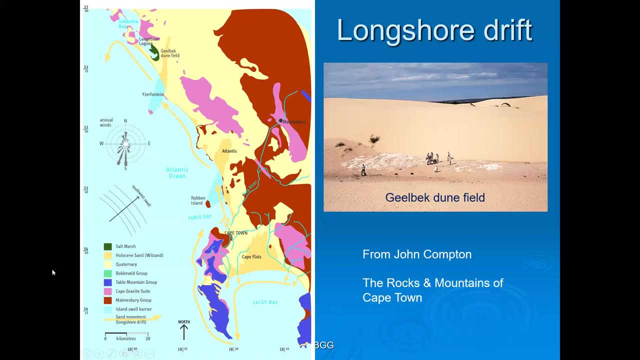 But you can see multiple veining episodes of quartz in the outcrop here of the Colenso Fort. This is just another illustration. I see John's on the call, John Compton, But you know quite often when you talk about the environment. 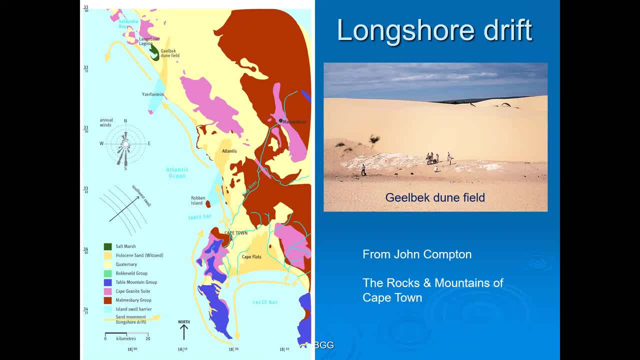 the discussion is pretty much dominated by the biodiversity people, the botanists, ecologists. But you know, geological processes are very important when you look at planning And this is a really nice illustration from John Compton, John Compton's book The Rocks and Mountains of Cape Town. 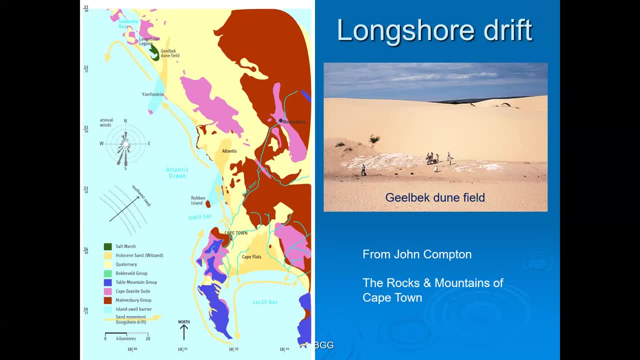 illustrating the longshore sand movement around the Cape Town area and up the West Coast, Also the two islands, Robben Island and Dassin Island, where you've got a shadow in the swell And that allows the fine sand to accumulate on the beach. 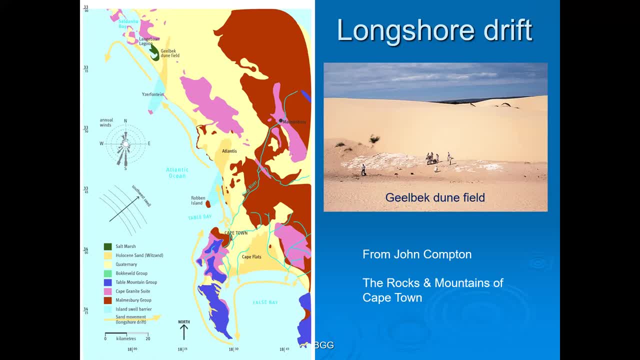 And then you have these really big dune plumes, one at Atlantis And up at Heelbeck in the West Coast National Park, You know. so geologists definitely have got a tale to tell. You know, we do work in the natural environment and we shouldn't let the conversation 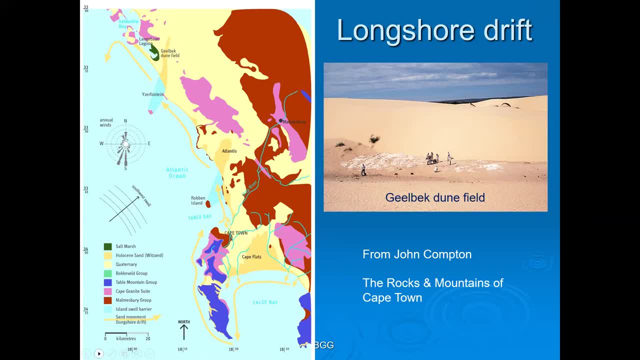 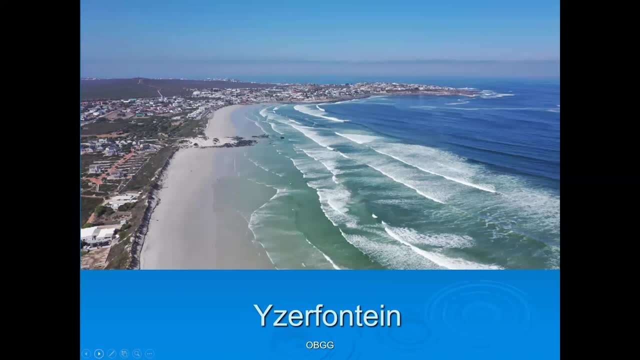 only be dominated by ecologists and botanists. This is just another little story. Duncan knows this. Duncan Miller knows this area very well. A picture of Azervon Plain looking from the north towards the south, with the hallway in the background, Gabbro Point in the mid-ground and then the dune of 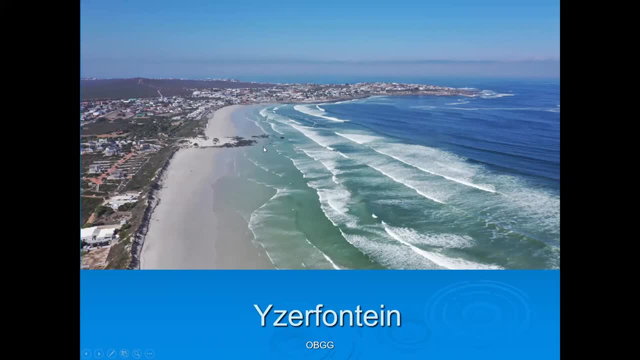 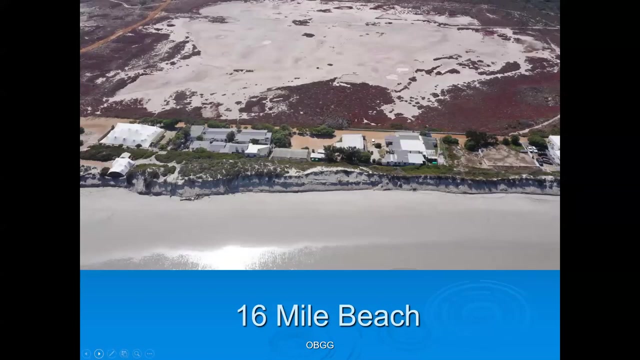 16 mile island stretching up to the West Coast National Park. We've been in Darling since 2011 and this dune has moved back. I can measure it on Google Earth at least 20 meters. This is another picture of the dune and you can see the pan in the background. it's called Roi. 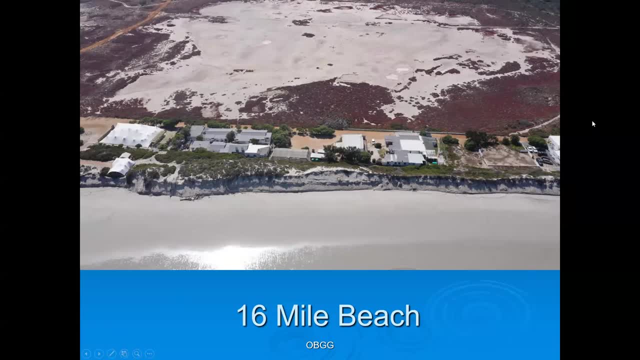 Pan, And obviously the sea was there once before. but if you look at the dune, I think you might agree that the sea is probably heading back to Roi Pan one of these days, And these are the type of things that geologists can contribute to, and 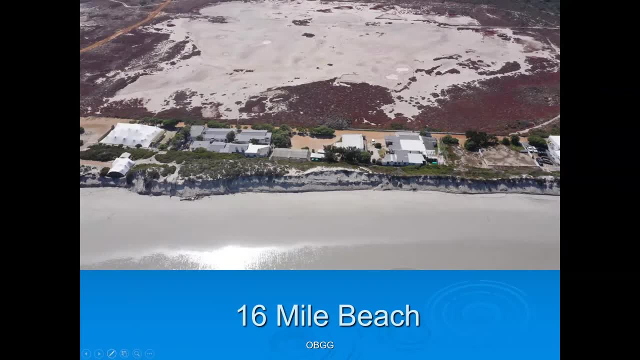 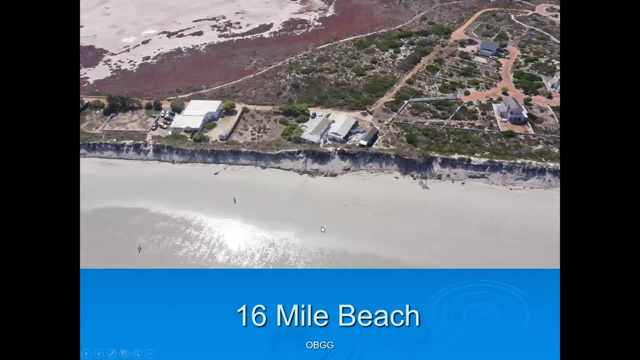 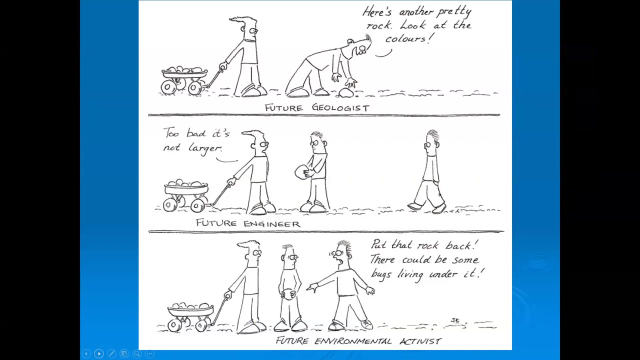 and should be taken into account by planners. Here's another example of 16 mile beach, and would you advise anybody to buy one of these open stands over here? I'm just wondering. can everybody hear me? Yes, you're fine, Okay. 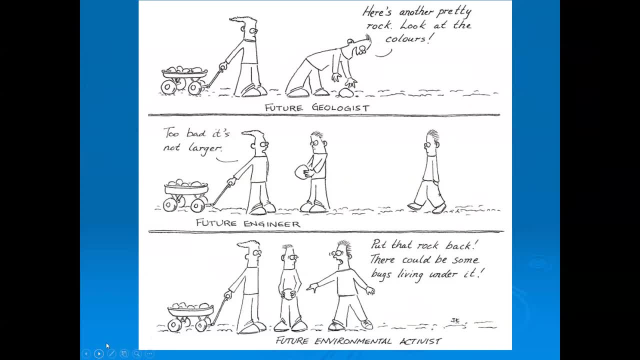 Now, this is another aspect with geology. you know, the world is made of all different types of people and everybody's got their own multicolored sunglasses on and they look at the world from a different point of view. This comes from the Northern Minor, so you can see what the geologists 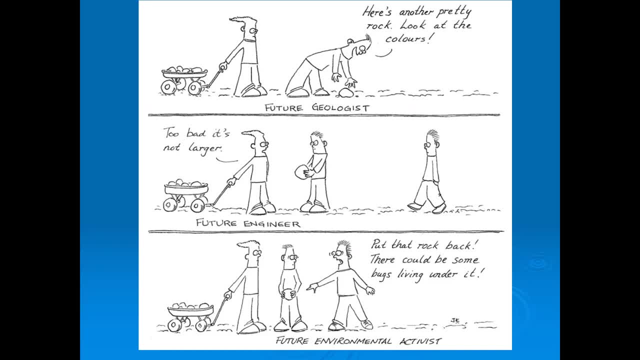 might think, or the mining engineer might think, or the environmental activists might think, And so So the you know, it's not just a, things aren't just simple, and sometimes decisions get made almost by who's shouting the loudest, not really by the facts. 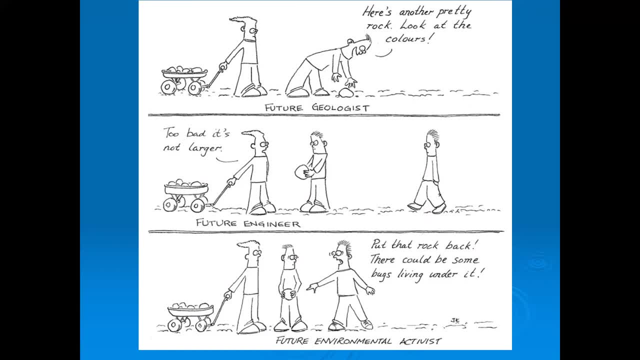 And you know, that's just a fact of the world and that's just something that one needs to deal with. But you know, I think it's important that geologists also put the case forward when it comes up in these type of discussions. 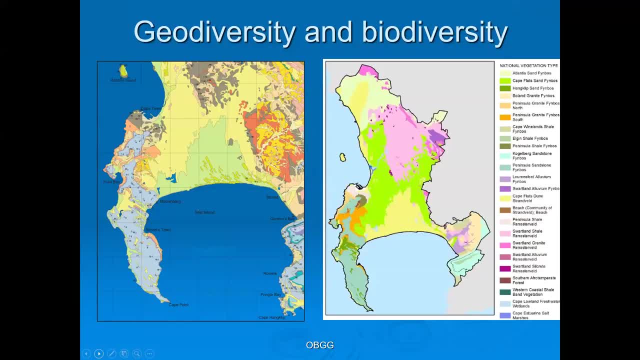 Now geodiversity and biodiversity. The biodiversity people have done a tremendous job. they've probably been off the mark much quicker than the geologists, and they've managed to influence legislation- policy regulations- far more effectively than the geologists. 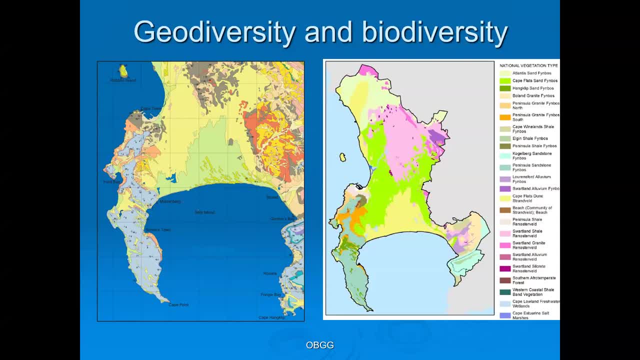 And geologists have managed to, But the fact of the matter is that the geology underpins the biodiversity. So here we have two pictures: On the left is the geological map and on the right is a map of the national vegetation of South Africa. 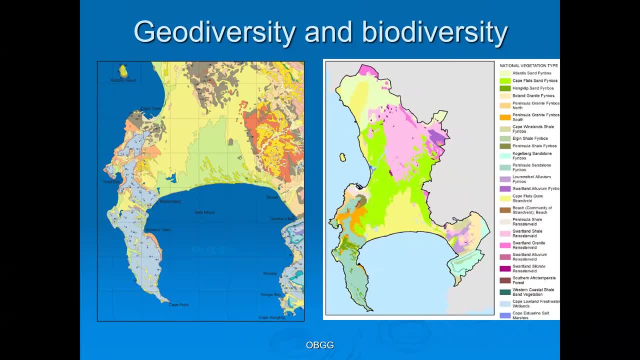 The national vegetation of South Africa. actually it's a very good book and it's available free on the Sandby website. But but if you look at the vegetation types, you will see that they come. they match almost perfectly with the geological units Here we have. 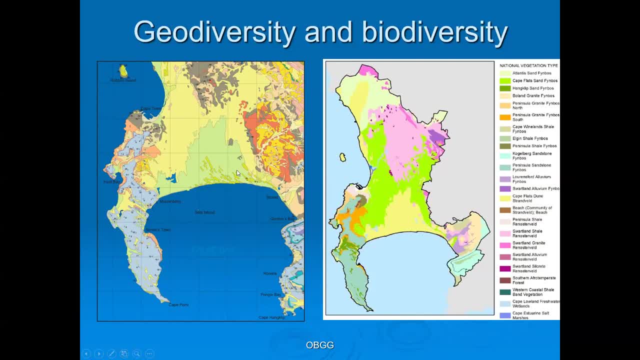 the Witsand Formation, which is the upper sand on the Cape Flats, which contains fragments of seashells, and it's mapped on the vegetation map as Cape Flats-Dune, Strandfold. The other different vegetation types you can see closely match the geology, Peninsula Granite, Fanebos and so on and so forth. So when the national vegetation map was created they actually did recognize that the geology 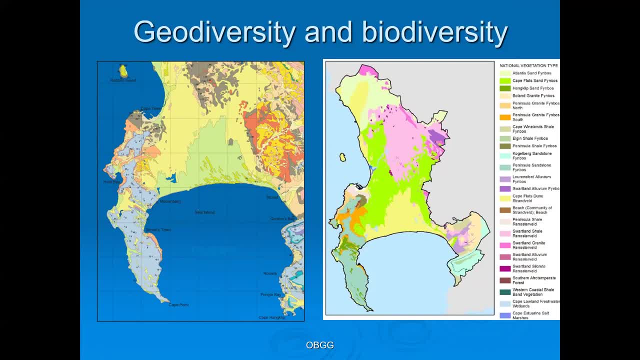 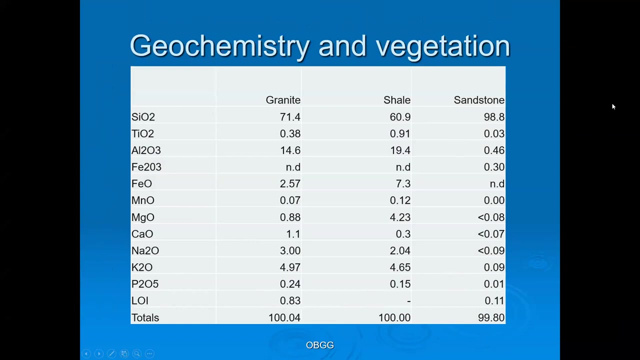 provides the nutrients that go into the soil and the soil determines. you know which plants prefer which soil areas. So there's a very close link between geodiversity and biodiversity And we know this. look at the geochemistry of rocks here in the Western, typical rocks that we see in the Western Cape: granites and shales and sandstones. 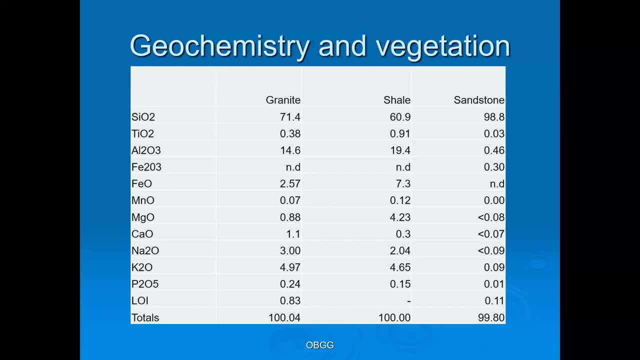 You can see how many greater variety of elements you get in granites and shales compared to the sandstones. The sandstones are almost like a glass bottle: Basically silica with very little else, The granites and the shales much more variable and that will also reflect in the trace elements in granites and shales. 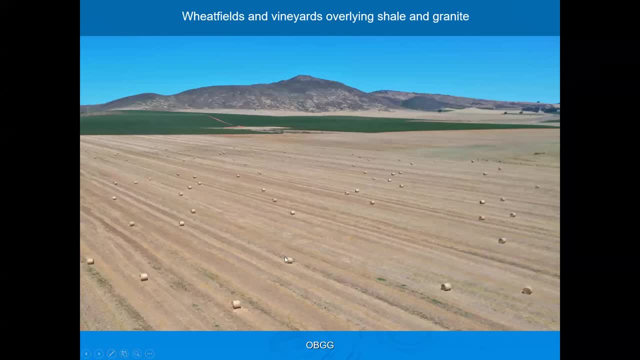 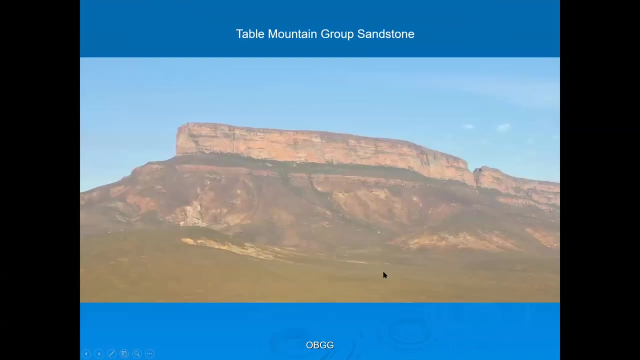 So this is a picture from the Darling area with the Darling granites in the background and some vineyards and and wheat fields. So the cultivated areas are generally overland, Generally overlying the shale and granite areas. This is another very nice example. This is from Matsikama up near Klava and Van Rensdorp on the west coast, So you can see the upper Nardo sandstone of the Table Mountain group and very clearly the different vegetation. 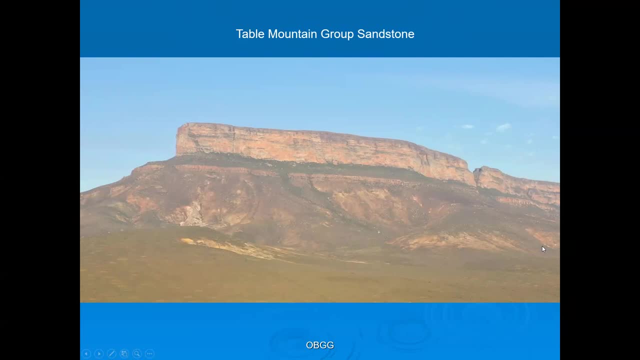 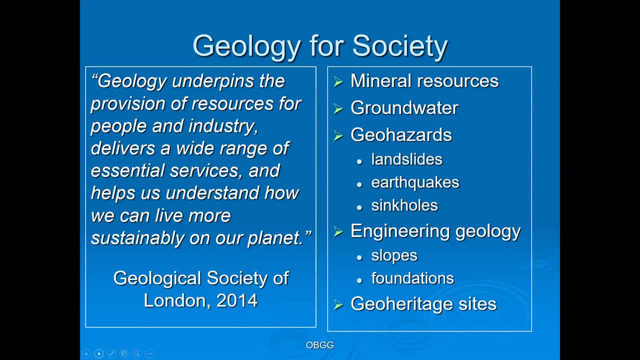 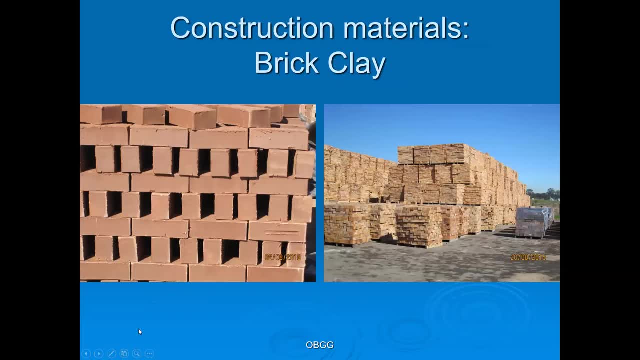 around the world, and I really believe that this information is often neglected or not considered as important. Now, kind of moving on to the topic that was advertised: typical construction materials that are used everywhere and in the Western Cape. One example: brick clay. I never knew much about. 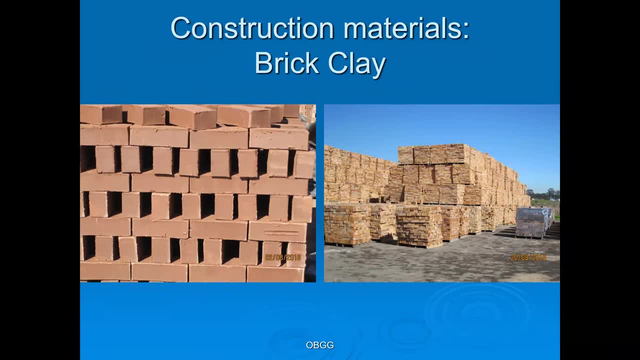 brick clay until I came back to the Western Cape, and now I really I think bricks are magic. They really are. The amount of work that goes into making bricks. the clay gets taken out of the quarry, it gets soured, in other words weathered naturally for six months. 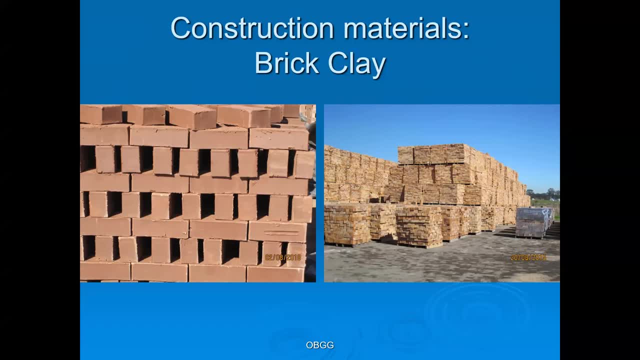 gets blended by the brick maker, put through a mill and then eventually squeezed out, extruded out and then gets packed into clamp kilns where basically the bricks bake themselves. You might have seen, when you drive past Port River, the brick factory and then eventually you get the bricks and you know they've got fantastic properties. 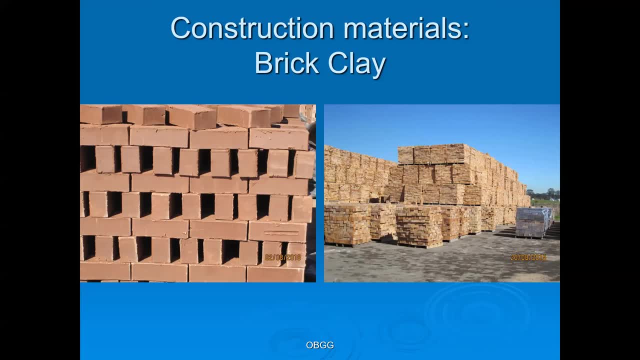 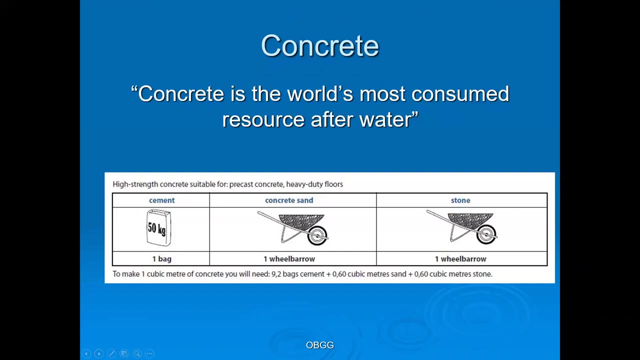 durability, long-lasting, etc. So you know it's a really underappreciated material but you know, really think they are magic. Then the next thing, which is concrete, and there's a statement that concrete is the world's most consumed resource after water. and so to make one cubic meter of 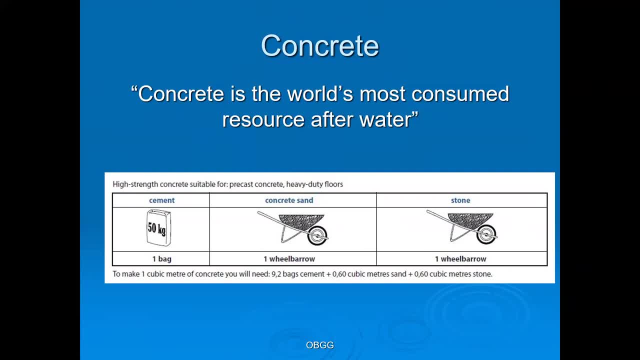 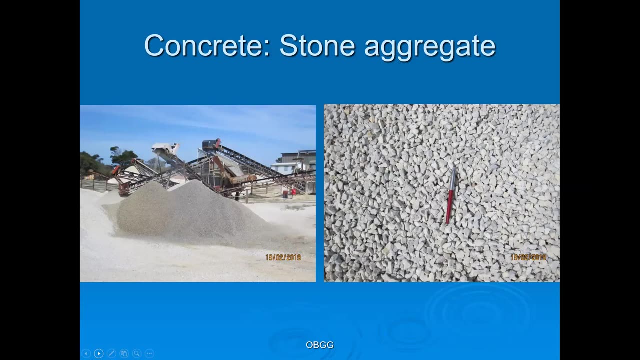 concrete. you actually need 0,6 cubic meters of sand and you need 0,6 cubic meters of stone, and this has all got to come from somewhere. Typical materials. here's a stone aggregate. this is crushed stone. this again from Robert Quarry. 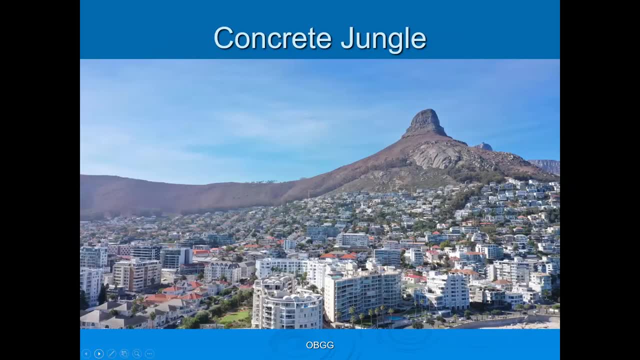 Here's an example. the material is building. material is all around us and this is just a nice example from Seapoint, because you can see the Cape Granite in the background. you can see the Malmesbury Shale on the left-hand side and you can see the capping of. 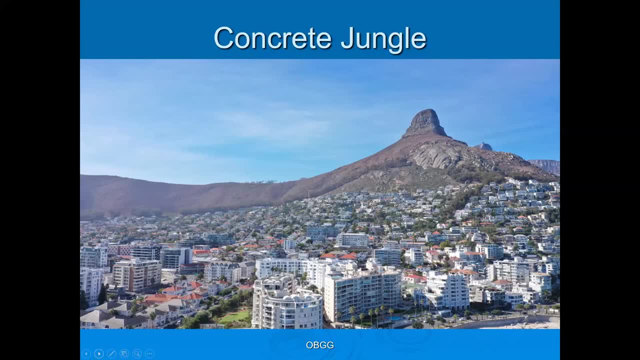 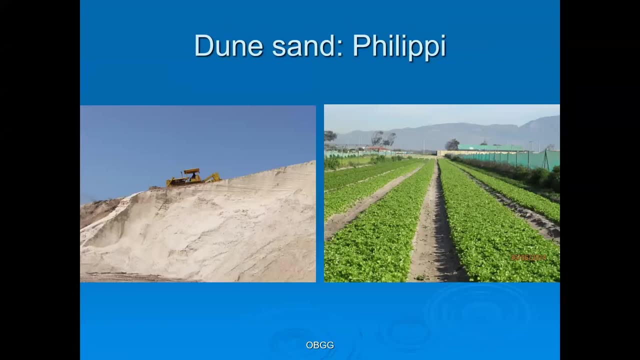 Table Mountain Sandstone in the background. Cape Town, essentially, was built from Philippi. The dune sand in Philippi was used for the freeway construction in the- when was it, Charlie Morris? in the 60s and 70s, and the Philippi sand is. 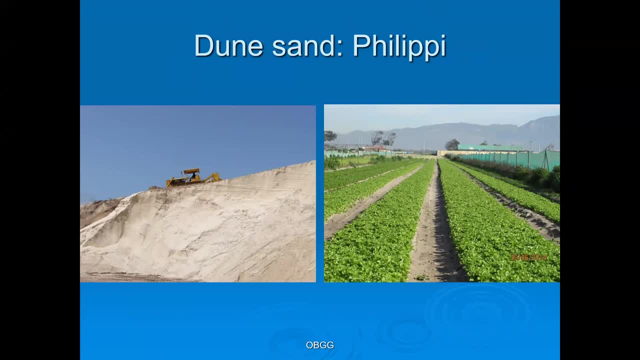 almost over. The very nice thing about the Philippi sand is that it's almost over. The very nice thing about Philippi is that once the overlying dune sand has been removed, it can be rehabilitated to form horticultural fields, and so Philippi is the breadbasket of Cape Town: all carrots. 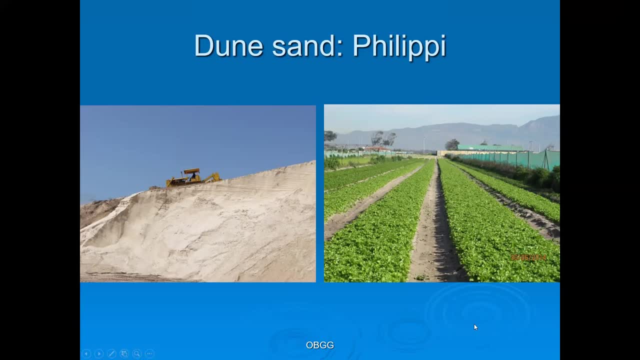 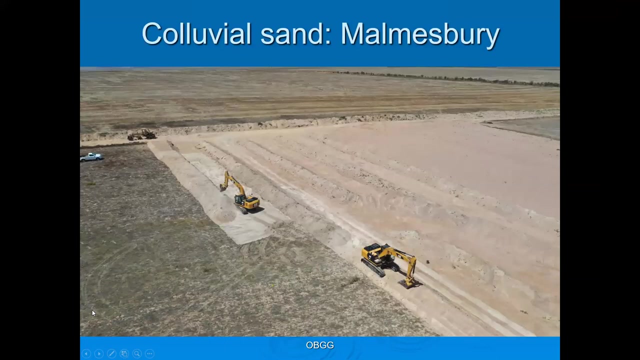 lettuces, vegetables- all sorts of things being grown there. Oh yes, also the nice cross bedding that you can see in the dune in this picture. Then the other type of sand that's mined around the Cape Town area is referred to often as 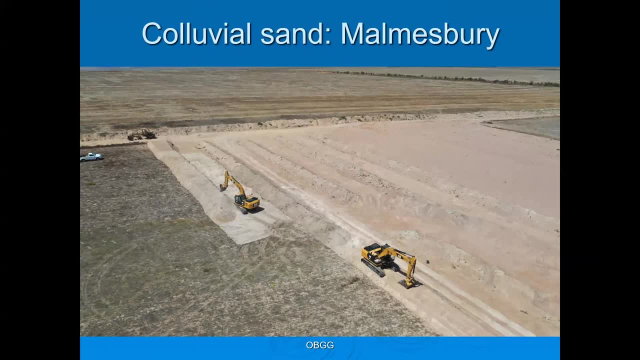 hill wash sand or colubial sand, and this is generally a bit coarser than the sand from the Philippi area and is quite prized for making concrete concrete sand. and here's an example near Darling And this is an example of an area where the sand is being mined around the Cape Town area. 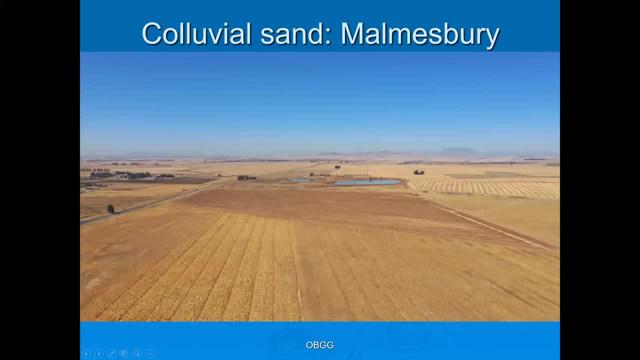 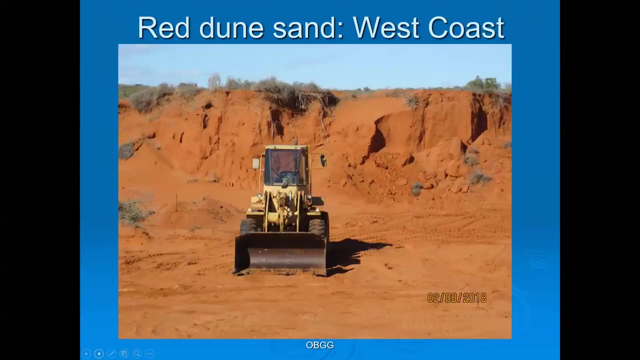 area that was mined for this exact same type of sand between Malmesbury and Clippierville, And it's actually been rehabilitated back to Wheatfields. You can see Table Mountain in the background. This is now another example of red dune sand. 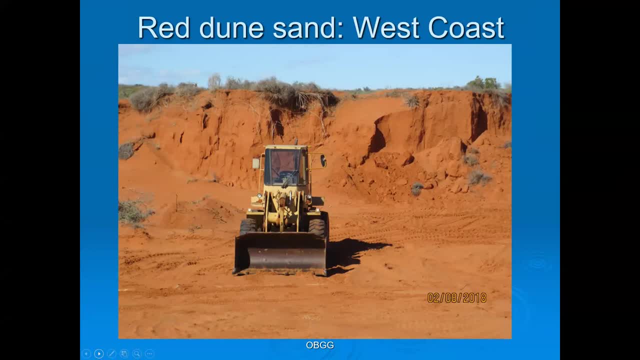 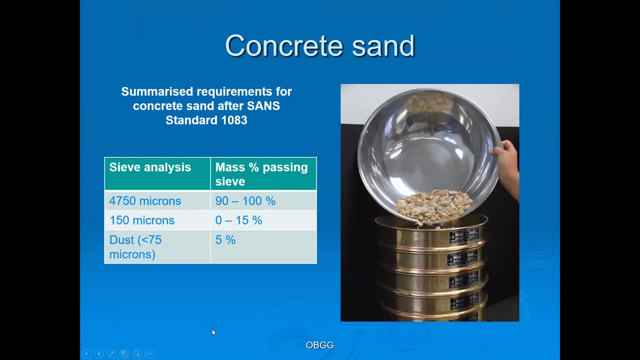 that comes up from the Fredendal area in the West Coast, And the thing is, sand is not just sand. There are actually specifications for concrete sand, plaster sand and mortar sand, And there are tests that need to be done if you want to make sure that your material complies. 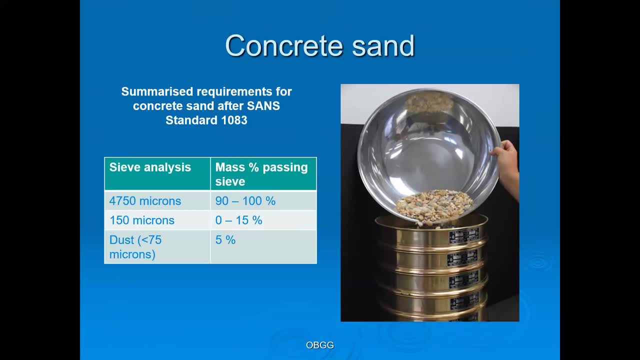 with these standards And they would typically do a sieve analysis for the material through the sieves and make sure that material doesn't contain an excess amount of dust Or the size is the wrong size fraction, And then they would put it up on a graph like this: 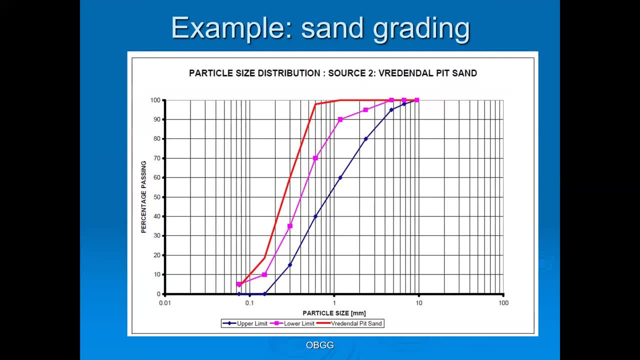 So you can see from this example, the red dune sand up in Fredendal does not fit in within the envelope for concrete sand. It's actually far too fine grained So it's not really suitable for making concrete. But what they use the sand for 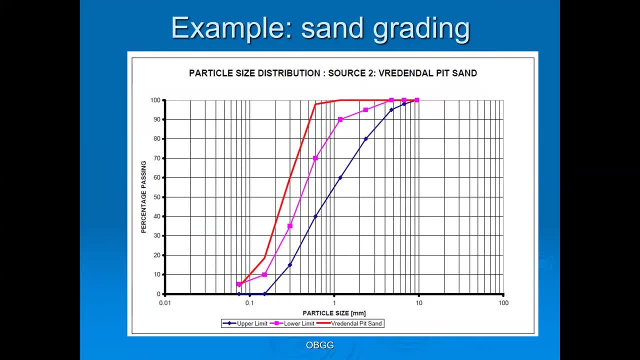 But what they use the sand for. But what they use the sand for When they fill up in the Fredendal area, it's actually just as a filling sand. So when they're working on a site and the site needs to be leveled, 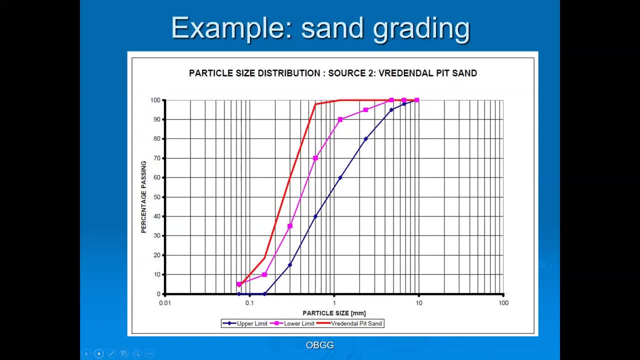 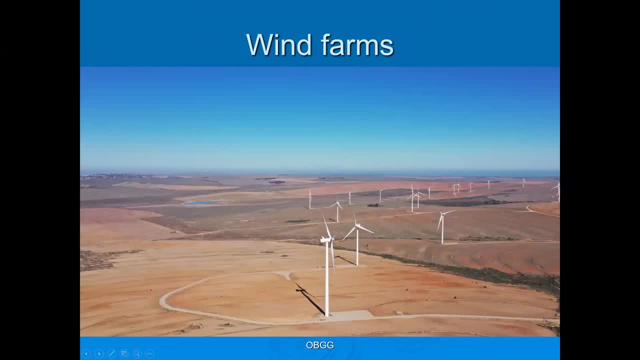 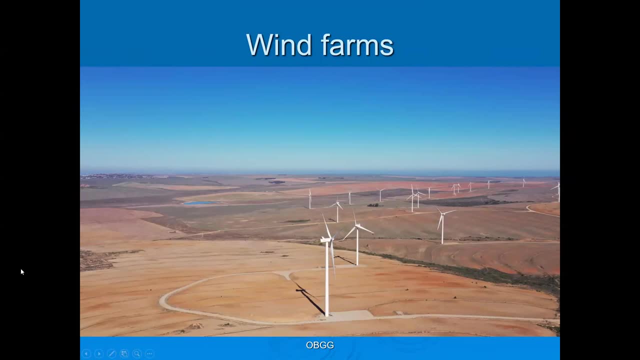 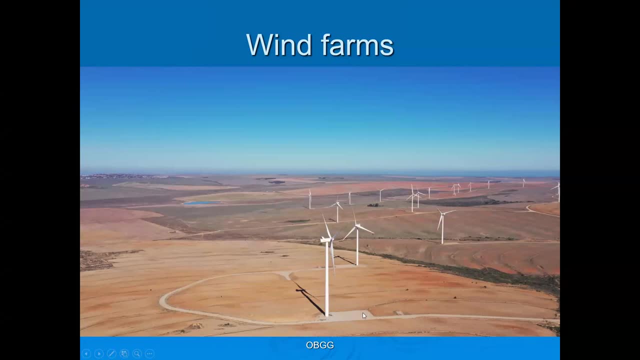 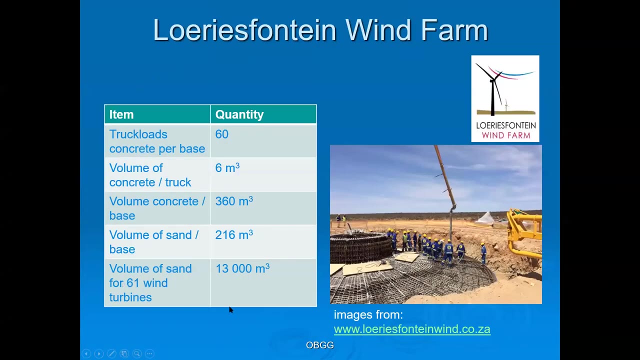 notice that each one has got a concrete area around the base. This is sort of like a little bit of a mini case study from the Lourdes Fontaine wind farm. You can see here they're busy putting a base up. And so you can see here they're busy putting a base up. 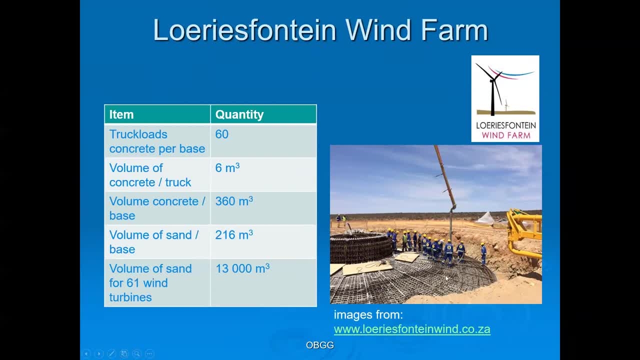 What you can see at the top of the base, with all the rebar getting ready. you can't have one of these wind turbines falling over. You've got to make sure that the reinforced concrete is strong And it's not a trivial amount of concrete that's needed. 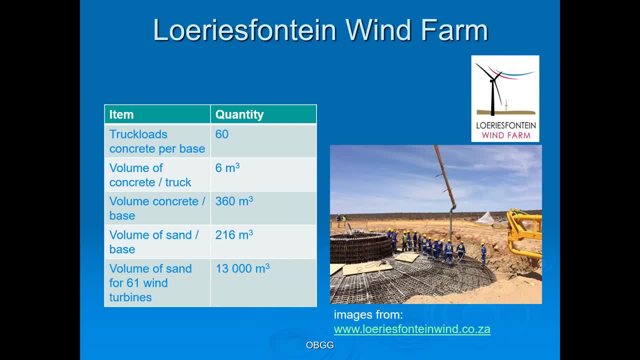 So for the base of each one of these wind turbines you need 60 truckloads of concrete for the base In a concrete mixer. you've got about six cubes In a concrete mixer. you've got about six cubes. volume of the base is 360 cubic meters. so you would need 216 cubic meters of sand for one base. 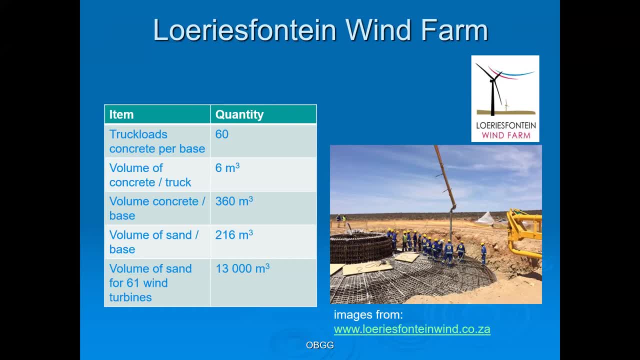 of one wind turbine And this Louries Fontaine wind farm has got 61 wind turbines, so they needed 13,000 cubic meters of sand. It's up in Louries Fontaine and there actually isn't much suitable sand. 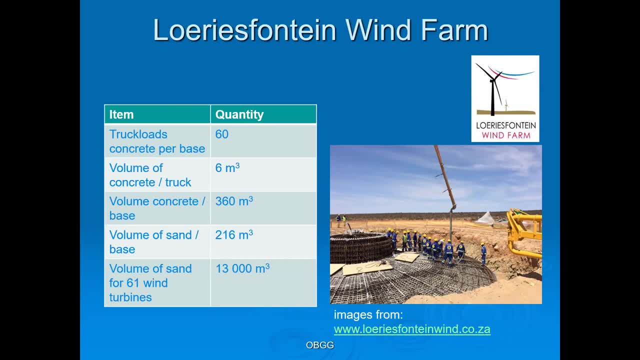 Louries Fontaine is in the Northern Cape, so this sand was literally exported from the Western Cape to the Northern Cape. If you're looking at a 20 cubic meter link truck, that's 650 truckloads of sand that are being exported. 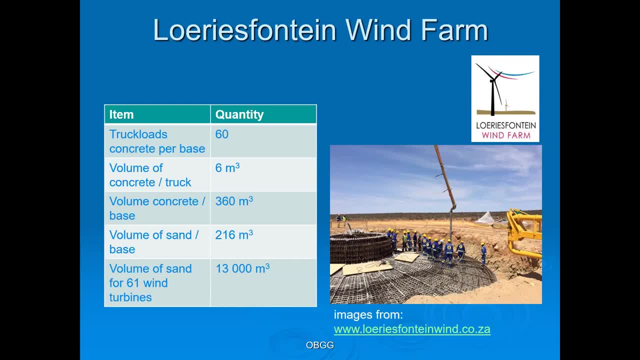 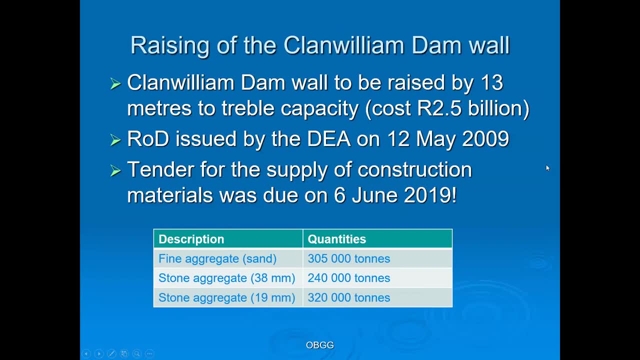 So the amounts of material you're looking at certainly aren't trivial. This is another example. This is a project that was meant to have happened and it hasn't happened so far. There's plants and machinery standing there in Clan William and the Department of Water Affairs never seems to have the money to do this job. 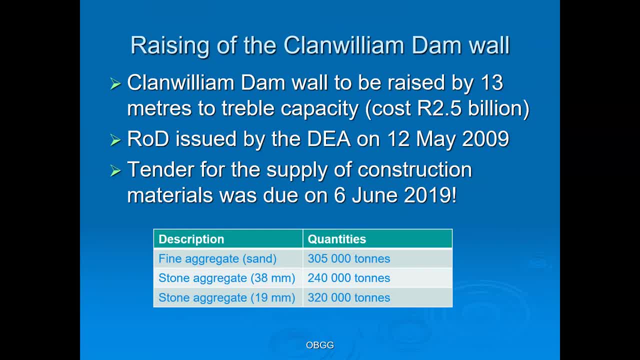 They put out a tender for the supply of these materials in 2019.. They never awarded it, but if you look at the quantities that they want, you know this is even an order of magnitude more than was required for the wind farm: 305,000 tons of sand, 240,000 tons of larger aggregate and 320,000 tons of a 19 millimeter aggregate. 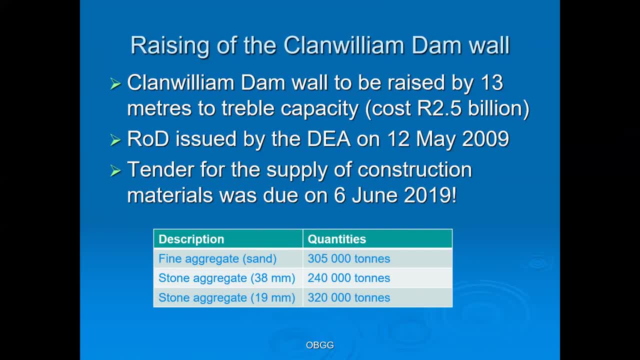 And you know that's the type of thing you think that they should have sorted. As far as I know, there's not a single licensed sand mine anywhere between Citrus Dole and Von Reinsdorf, you know. so it's just an aspect that, to me, planning should be better. 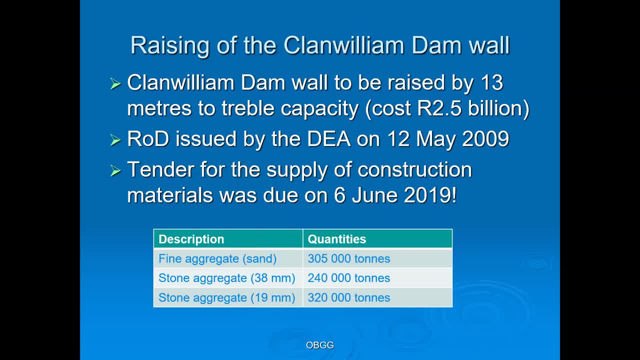 They should maybe be thinking of alternatives. maybe during the drought They could have even got sand from the bottom of the dam and created some more volume at the bottom of the dam. Okay, we're going to move over a little bit towards town planning. 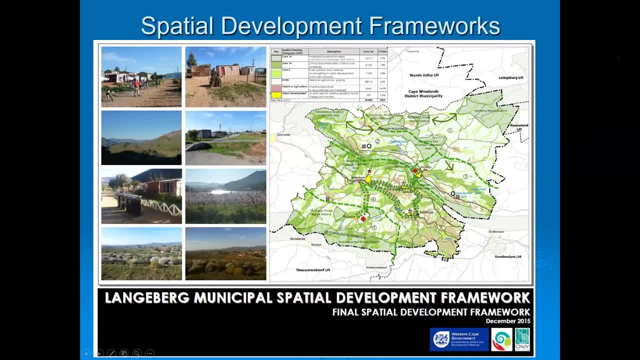 Now every municipality has to put together a spatial development framework and you'll see, in these spatial development frameworks they have the green areas, which they call core areas, and then they have buffer areas, and then they have the urban areas And most of these plans, the basic information, comes from mapping that was done by Cape Nature. 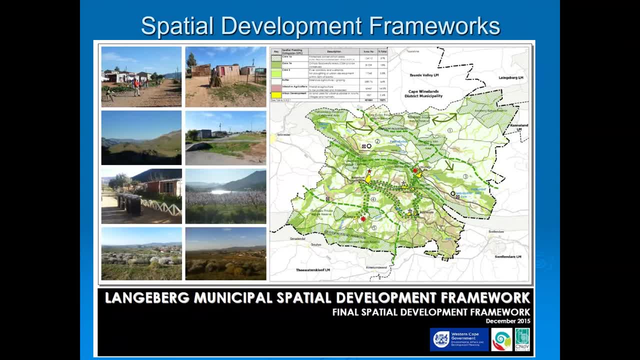 and the South African National Biodiversity Institute called Biodiversity Spatial Planning Frameworks And basically the biodiversity sector got in fast. they made the information available and they made it so easily available that the town planners use it. It's just very simple for them to use and that's. 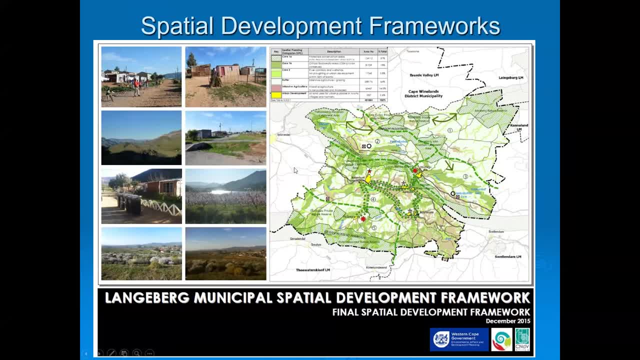 just the accepted way of doing this. Here's the spatial development framework. So this is the Biodiversity Spatial Planning Framework. Here's the Biodiversity Spatial Planning Framework. Here's the Biodiversity Spatial Planning Framework. Here's the Biodiversity Spatial Planning Framework. 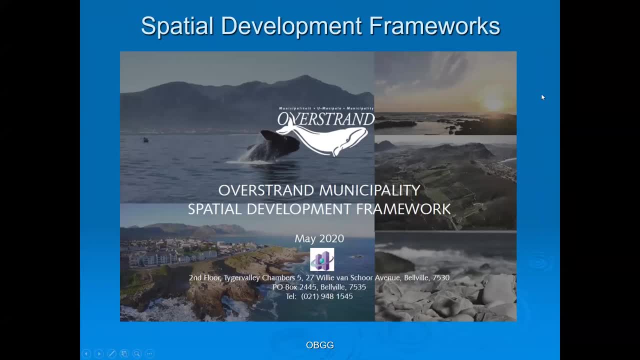 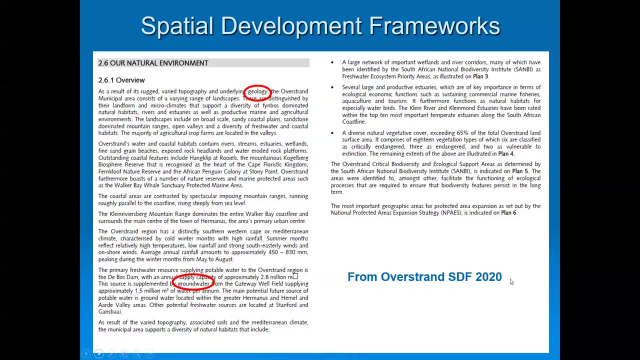 So this is the spatial development framework from your part of the world. down there in the Overburg, I had a quick look at it the other day and I skimmed through it and I found the word geology. I did a word search. it's once. 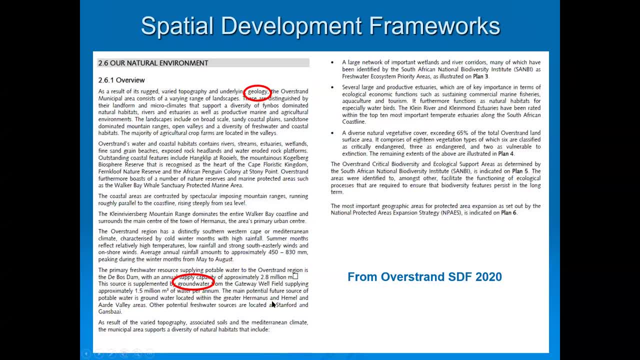 The word geology and the word groundwater also is once in the whole Overburg spatial development framework And if you read through the writing you'll see the spatial development spatial development framework. and then they refer to the over-strand critical biodiversity and ecological support areas determined by SANBI. So what was provided to them by the 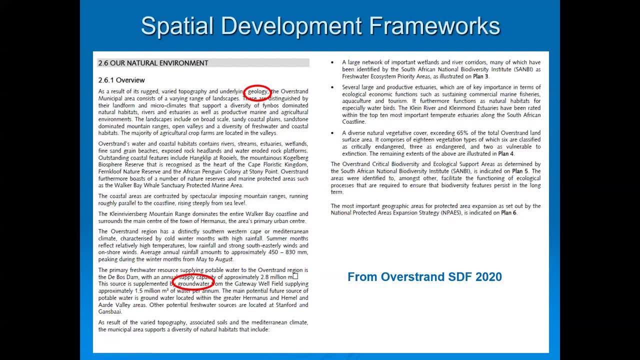 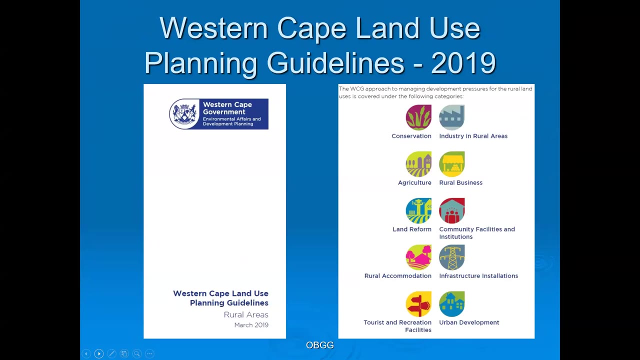 biodiversity, people is taken as reflecting the natural environment. It is a very good document but it obviously comes from that particular point of view. If you look at the Western Cape Land Use Planning Guideline document, look at all these different activities that they want to plan for- Conservation, agriculture, land reform, accommodation- They don't make. 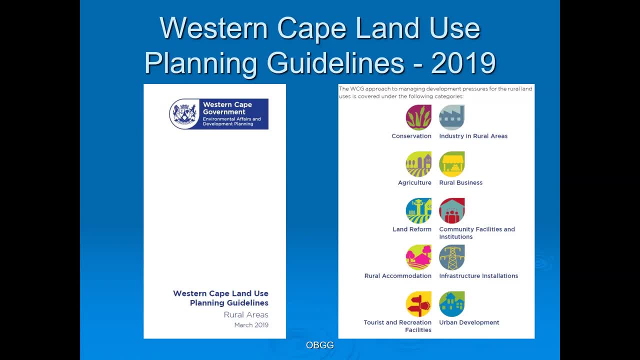 any provision for the land use where the materials come from, and a lot of our construction materials in the Western Cape actually do come from rural areas. If you put in an application away from people, it's actually much better. you know you're not disturbing people and a lot of the mines are out of town. 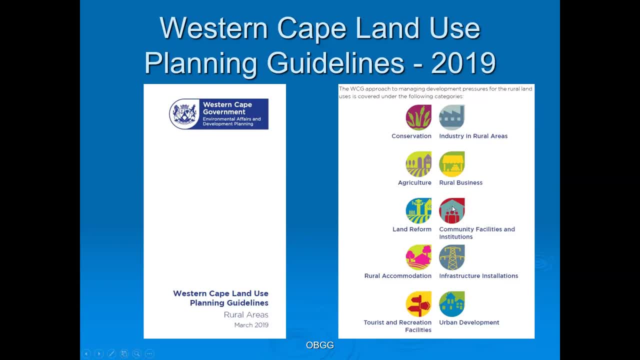 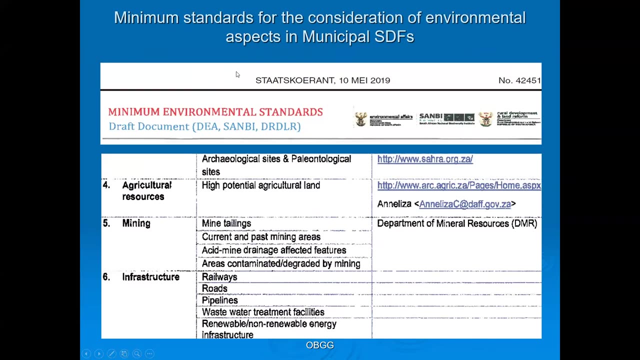 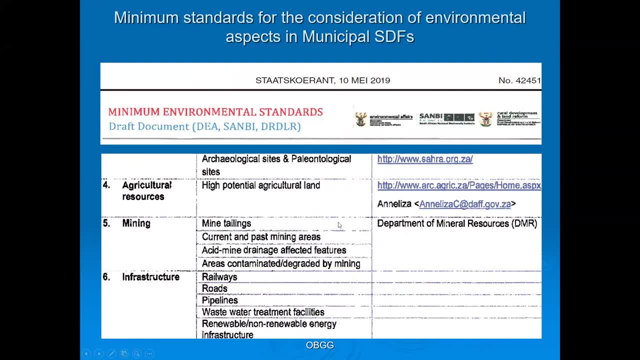 They didn't get a lot of information. They didn't get a lot of information. They didn't really seem to look at anything positive. These are the things they want to look at: Mine tailings, current and past mining areas, acid mine drainage, affected features, areas contaminated and degraded by mining. 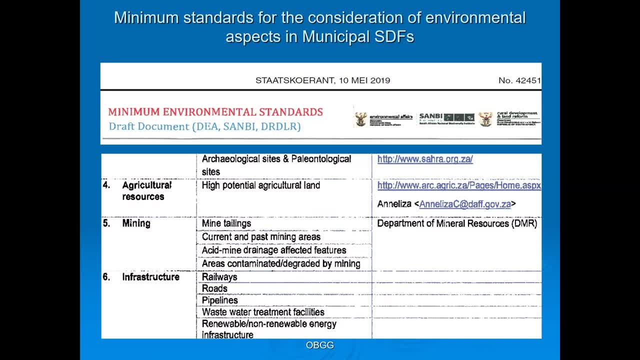 Now, all these municipalities actually need the materials to build their towns. How come they aren't planning for where do their materials come from? You know, do the materials come from checkers or because they're going to have a warehouse? But it's a basic. 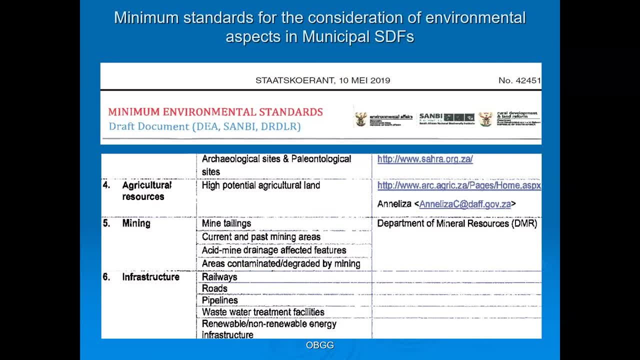 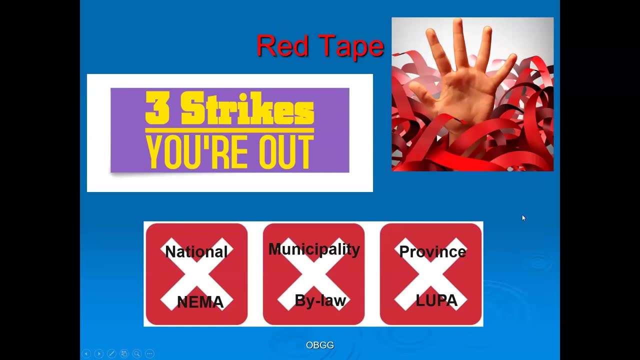 thing that municipalities should make provision for. where is the material coming from that's going to be used to build their towns? The other thing that we're dealing with is that there's so much legislation these days, So you have your national environmental legislation and if you do have eure dei deserts, you have your metro. Do youработ it? Do youre going to get it? 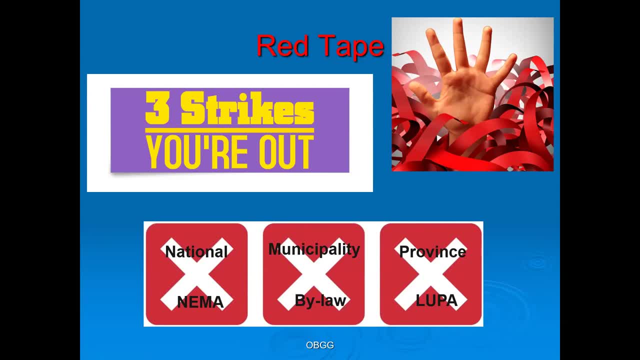 If you do a mining application, you have to remember that it's a dual application. You submit in terms of the Mineral and Petroleum Resources Development Act and simultaneously in terms of the National Environmental Management Act, And the National Environmental Management Act has got very strict timeframes. 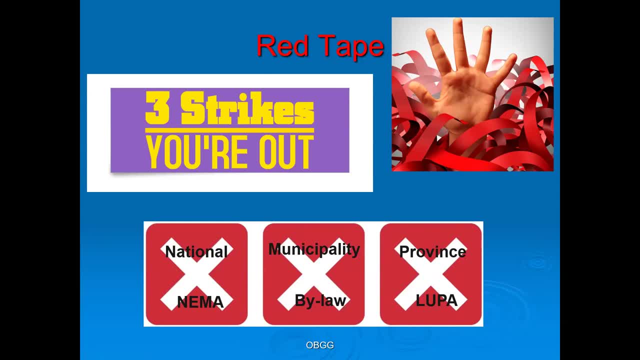 It requires extensive consultation with stakeholders interested in affected parties And these timeframes are pretty inflexible. So for a small mine or mining permit a basic assessment is required and that process takes six months. If it's a mining right, it's a full environmental impact assessment. 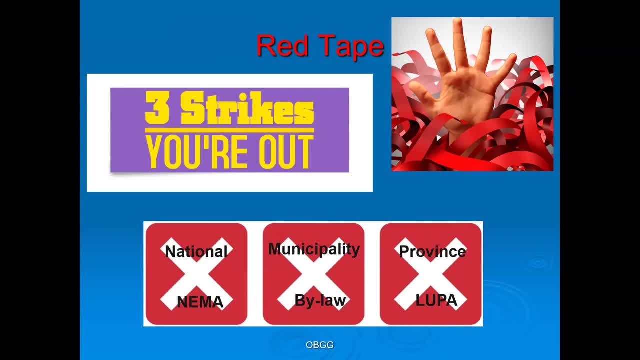 and that process. That process takes 12 months, And so that's like the limiting factor. So if the National Minister of Mineral Resources says that they're going to speed up their processing, well he can't actually, because the mining right or mining permit can't be issued. 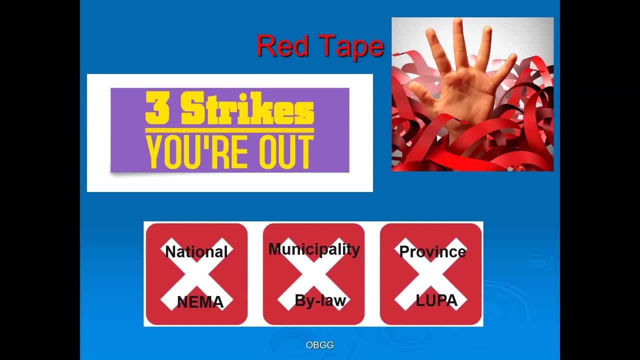 until environmental authorisation is granted. So the permission to speed up mining right applications doesn't lie with the Minister of Mineral Resources. It actually depends on the process of the National Environmental Management Act and that affects That's the same for all applications. 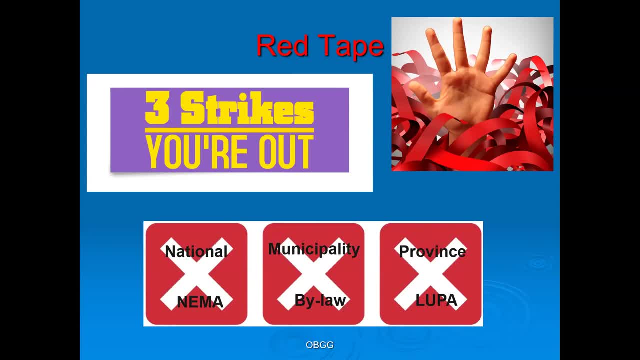 whether it is a mining application or just a normal construction municipal type application. And here in the Western Cape we're also affected by laws that might not- that might not be effective if the street business apply in other provinces. but the municipalities also want mining applications and to be approved. 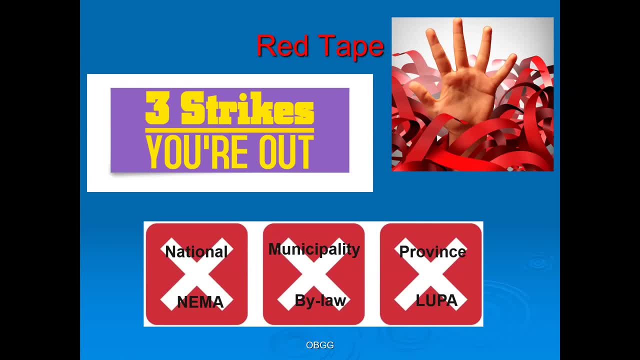 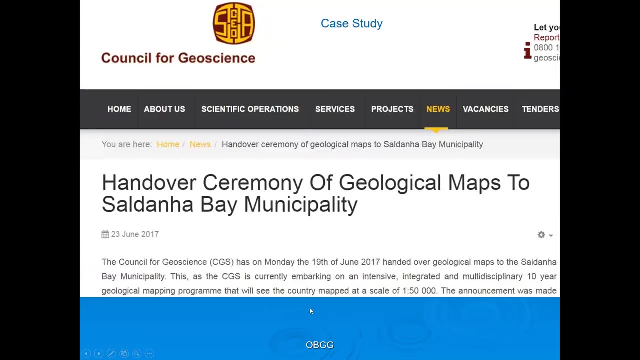 by the municipality and in some cases on agricultural ground. the province also requires a third permission, which is for the provincial land use planning act. now, this is a totally separate issue. this is a little bit of a case study, because the council for geoscience has done mapping and- and there's more mapping than we- 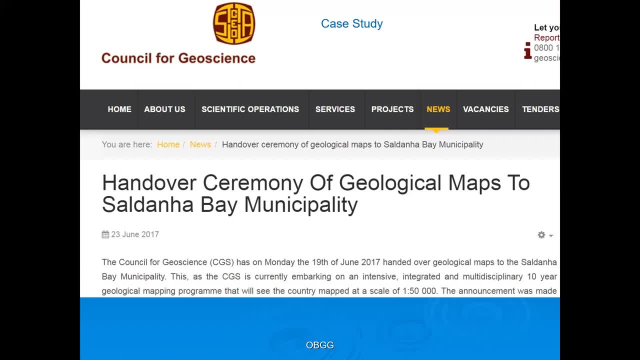 actually i realized there's more- one in 50 000 maps that have been made available recently and in this little short case study, the council for geoscience has done mapping and there's more mapping than we actually. i realized they actually handed over the brand new one in 50 000 maps for sildana bay, friedenberg and feltrift. 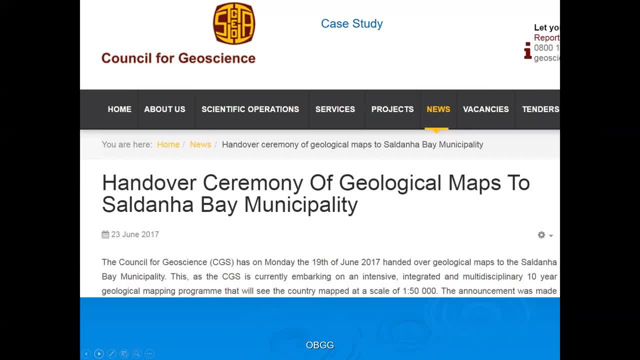 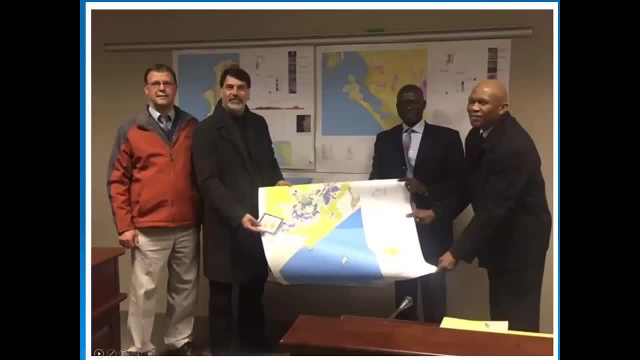 to the, to the municipality in in the sildana bay area. um even refers to the colenza fort. and there's proof, there's the map. there's the mayor of sildana bay municipality. he's got the map. he's got the cd with the digital copy. 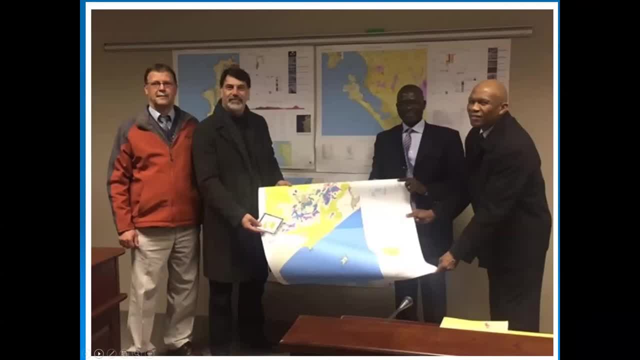 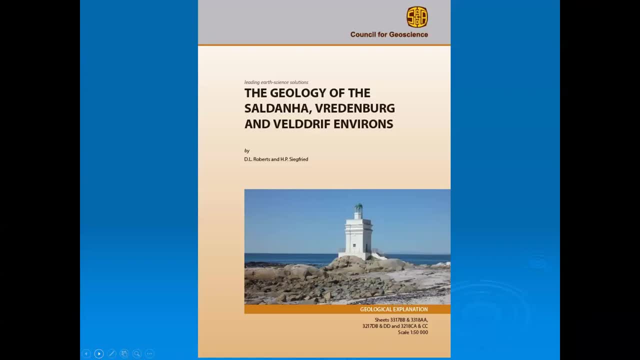 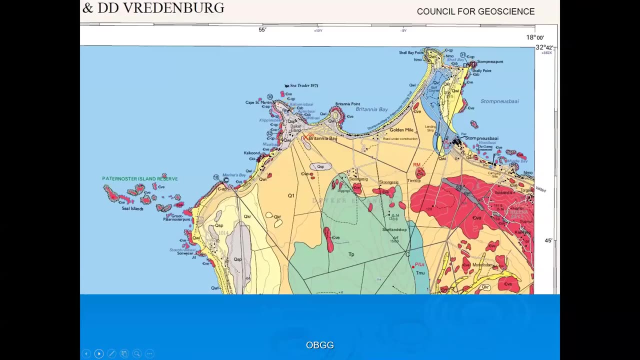 of the maps. he's got the report um. it's actually a very nice document and it was done by peter siegfried and dave roberts got a lot of detail in it. it's even got geological stops you could take yourself on your own geo trail- and the numbered positions with photographs that you can access. 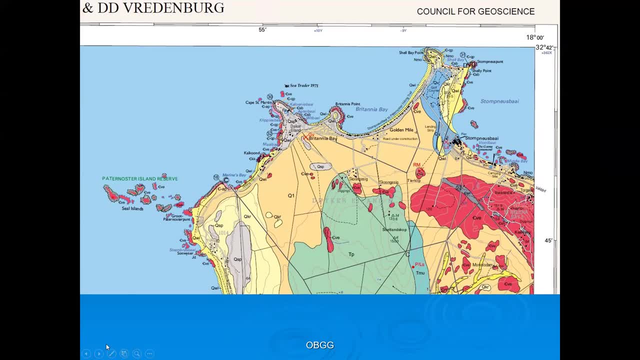 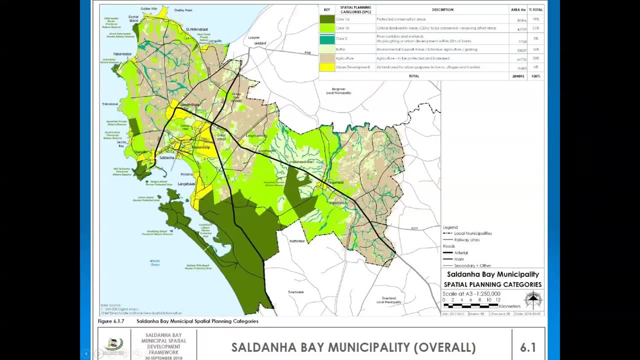 drive around. it's really a high quality map and it was a particularly ideal map. it's a very good map, given on a plate to the sodana bay municipality, and again we go back to the spatial development framework that was drawn up for the municipality and again it's divided into these core areas. 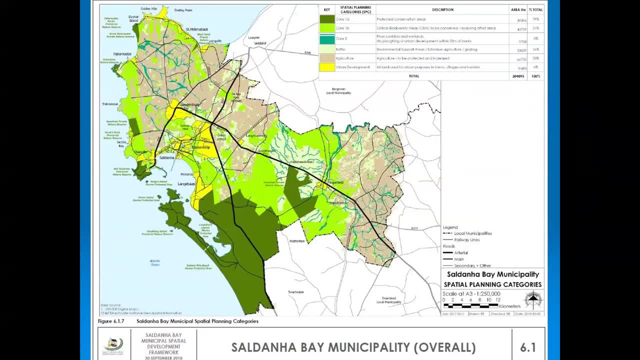 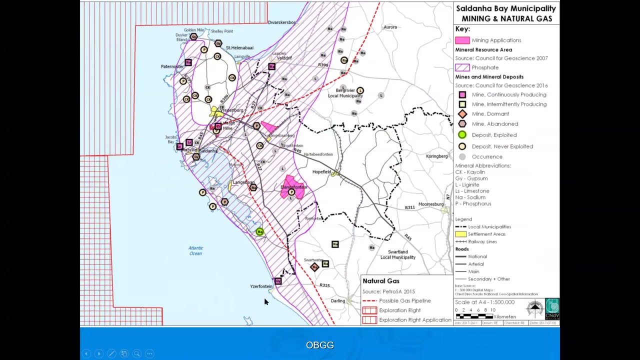 and buffer areas and pretty much derived from the mapping that was provided to them by sandby and cape nature on the western cape biodiversity spatial framework maps. but in in their documents, the town planning document, they've got a section on mining and natural gas. now if you look at it you'll see they go back to information that comes from 2007. 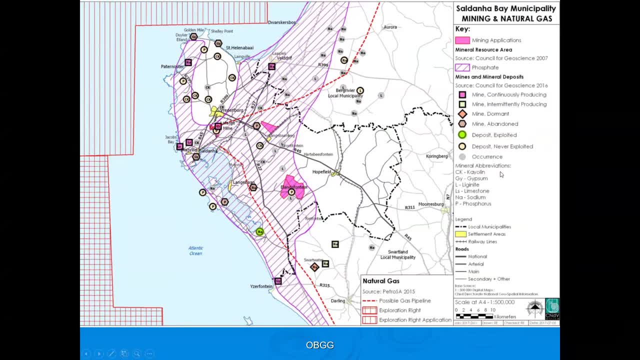 um, they have things wrong. they can't spell kaolin, they put phosphorus instead of phosphate. um, and what's even worse is they've interpreted an area which, which is hashed in purple, um, and they call it phosphate, and it covers a huge area. now, if anybody has, 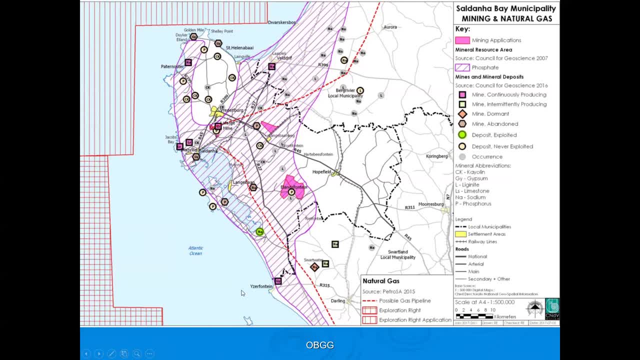 read the geological reports. the phosphate deposits deposits are in more carbon derived Obviously né she says that still relaxed and through process across all our geological不是 Hokkaido, but in recent years we've discovered these ph nivea, also more discreet areas. So around Ilans Fontaine there's a deposit. 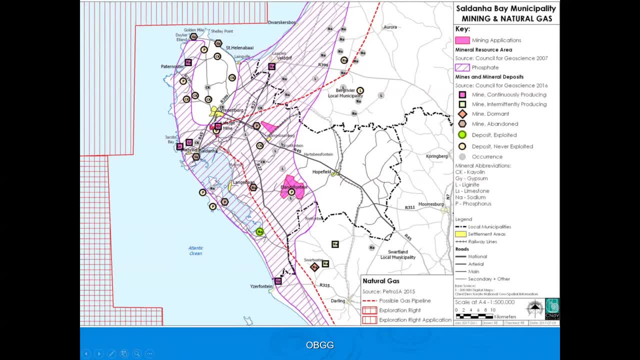 there's another deposit closer to town, but maybe there are currencies of phosphate in other areas, but it's certainly not all to all covered in phosphate. And then the following map: they've got hazard and impacts and they've got down here. 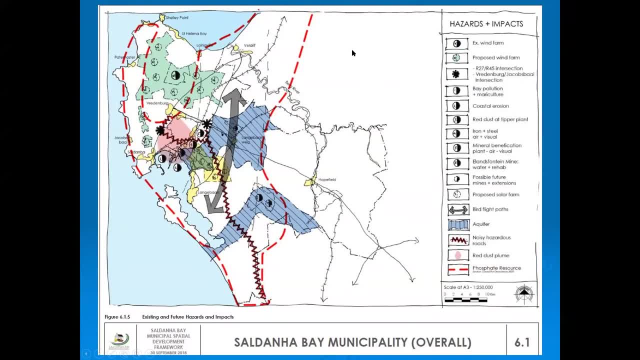 phosphate resource, as if this is sort of like a major thing that everybody has to be concerned about in Saldanha Bay. It's not correct. And these town planners- they're meant to be one of the best town planners- and it's wrong and it concerns me. 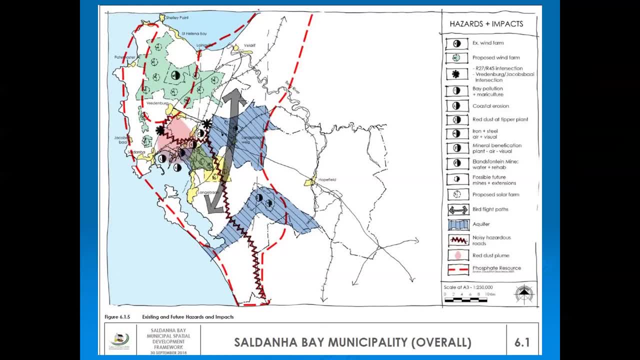 And they're putting down mines here as hazards. Now the quarries that Saldanha Bay is built out of. why should that be a hazard? It can be a very well managed operation. It can have a fairly confined footprint. 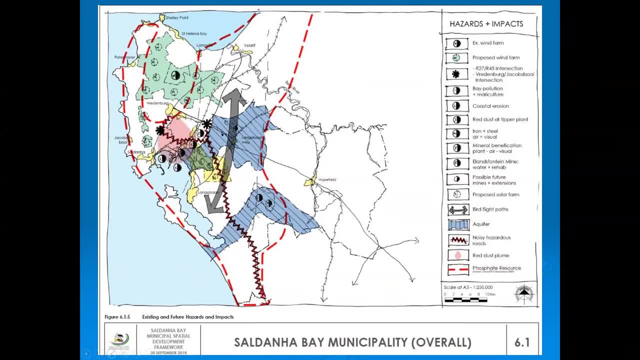 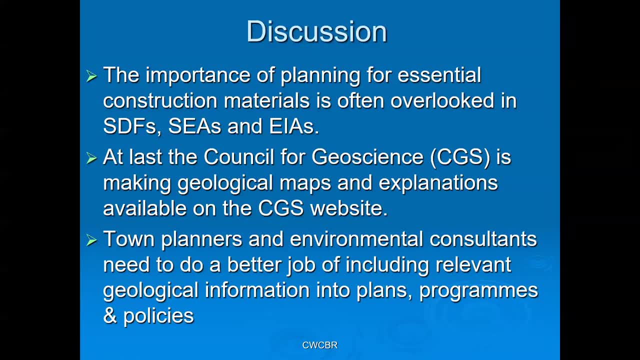 And you know. so I just I think it's wrong. So the importance of planning for essential construction. it's often overlooked, and this is by provincial and local scale, EIAs and planning. Then, at last, the Council for Geoscience. 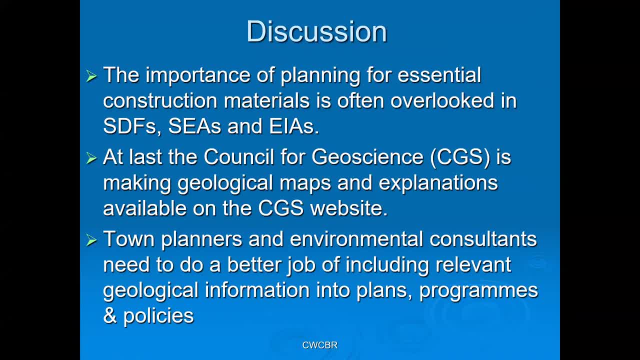 is making geological maps and explanations available on the CGS website, And that's something I've been sort of trying to motivate for quite a few years. I've written letters to the Council for Geoscience. I had a letter published in the Geo Bulletin. 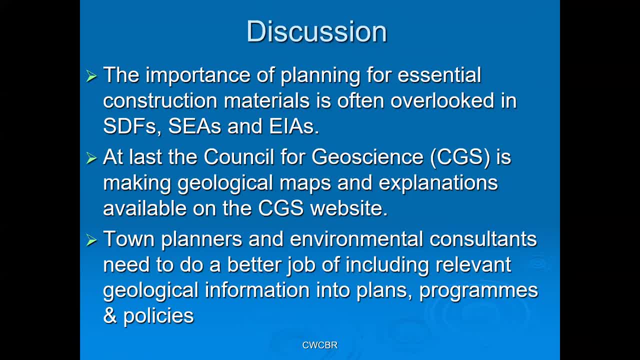 kind of constitutionally by me and my wife last year And that is definitely progress. In the Western Cape we've got a very good website called Cape Farm Appa, If anybody's interested. it's got all sorts of information on farms all over the Western Cape. 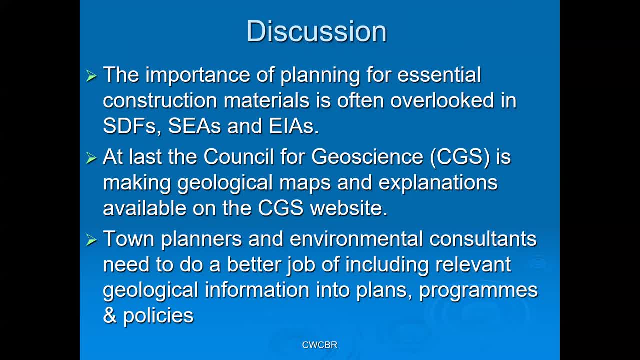 It's got cadastral boundaries of properties, It's got water resources, conservation resources and Cameron from the clients- Oh hello, Donald parfois fu. the council managed to get them to put the one in one million mapping, which is which is progress. 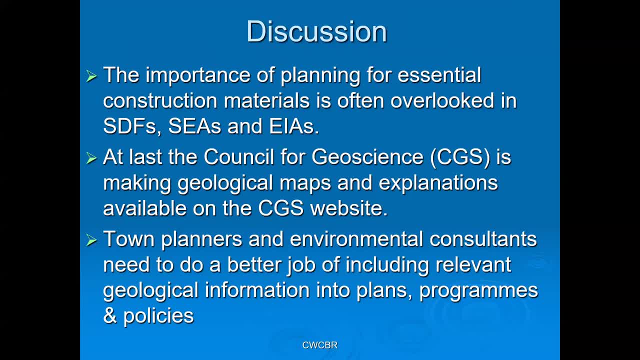 um, eventually it would be nice to even get the one in 250 000 mapping available digitally um in you know, in england you can get uh ideology. you've got all the bgs mapping available on your cell phone, um and i think we should aim to get our geological information accessible, you know. 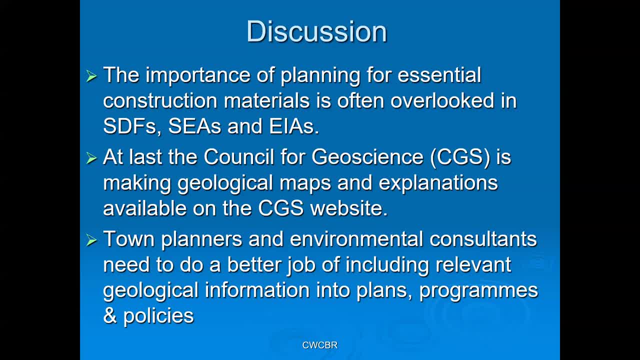 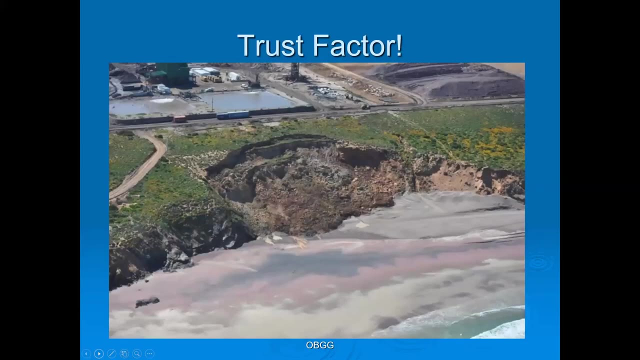 the sooner the better. um, this was a talk that i gave to the iaia- well, part of it- and i was trying to encourage them to get better geological information into plans and policies and so on. so i'm just repeating that, um, but, but. but the converse is is true, and i think kenny mentioned it as well, you know, in. 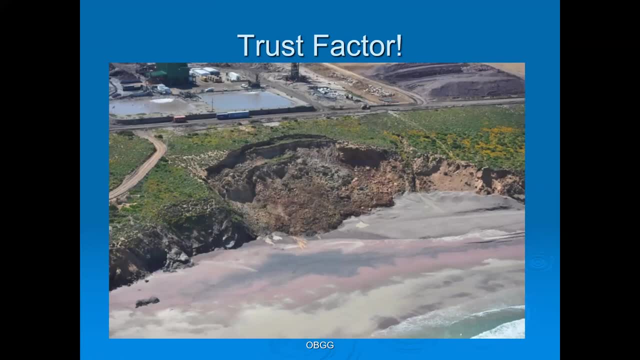 geology and mining. there is a trust factor and people can be rightfully concerned about things that have happened in the past and and also things that are currently happening. this this is uh the tolman operation up the west coast at uh hillville carew, a heavy mineral sand operation and uh, you know, over mining, undermining the cliffs, and you have. 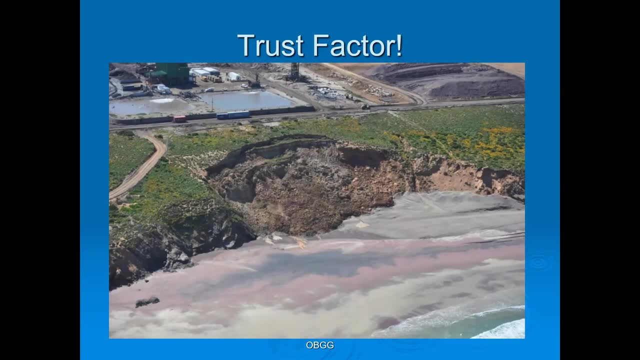 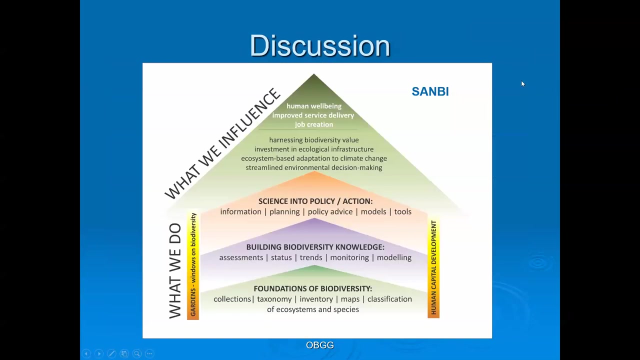 a cliff collapse. so you know, i think when things are done wrong, then geologists also need to say- and maybe not a very clear way to to end it, but i just sort of put this up as an example, because this is kind of what what the ecologists and the biodiversity people 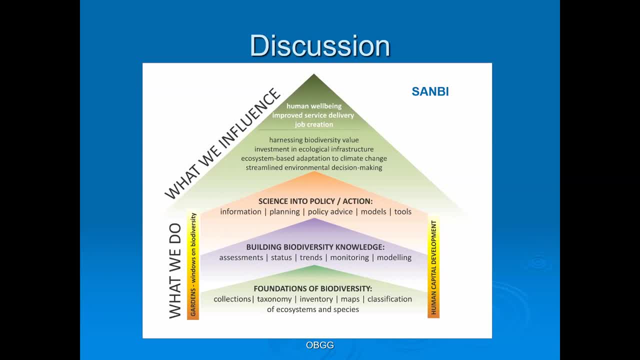 have done and how the conversation has been going, and and so the old sanby was the south african national um biodiversity institute and i now might be going back to the greenland, but i think we will go back to the south african national botanical institute and the south african national botanical institute. 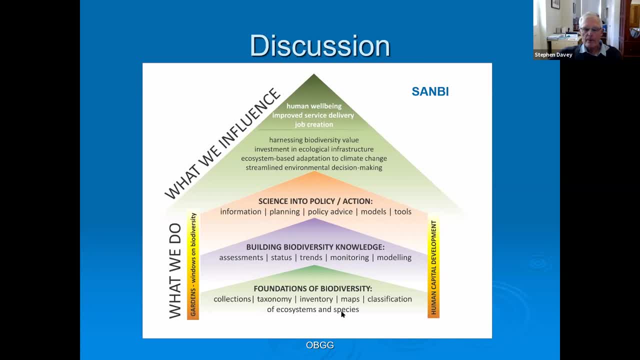 and south african national botanical institute, which was, you know, a scientific body that would do these type of things- connections, taxonomy mapping, very serious science. They grasped the opportunity and they got money from the Global Environmental Fund. they did botanical and vegetation mapping of South Africa, which they've made available. 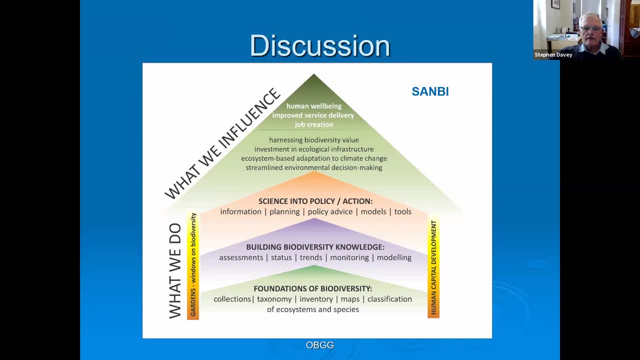 And they've kind of moved out of just being scientists and have really gone out of their way to influence policies and legislation and things like that. And you know, I think that, if we can, the geologists should also try and move out and get the message out and influence. 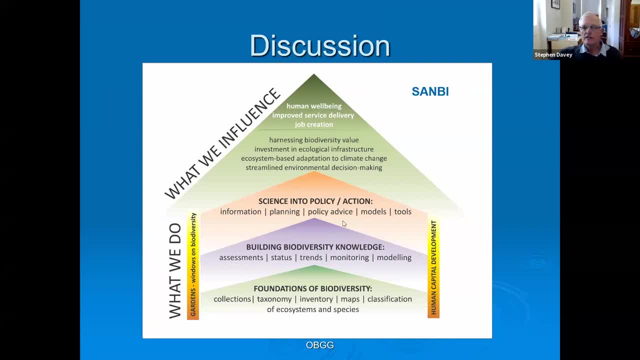 just as much as they can, Just as much as the people in the biodiversity sector have done, Yeah, so I think that's pretty much what I've got to say. Henny and Jonny, do you want to start the conversation, or what's next? 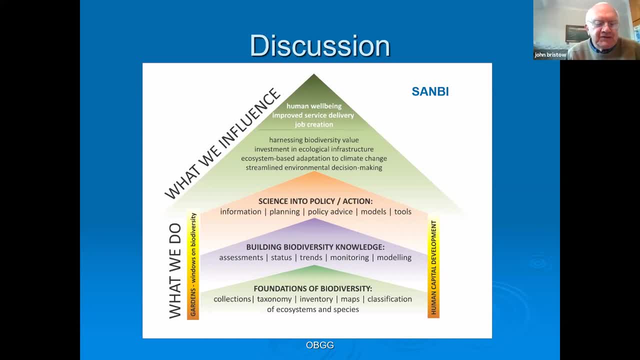 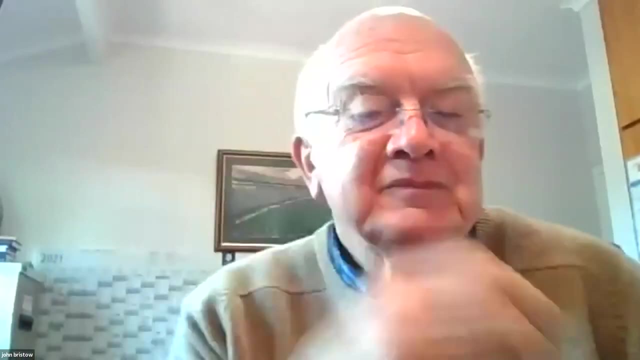 Thank you very much. Thanks, Stephen. That's excellent. I certainly believe there's a whole lot of discussion that will follow from that. You can download or stop sharing your screen and then we'll open up the discussion. Okay, Question time. ladies and gents. 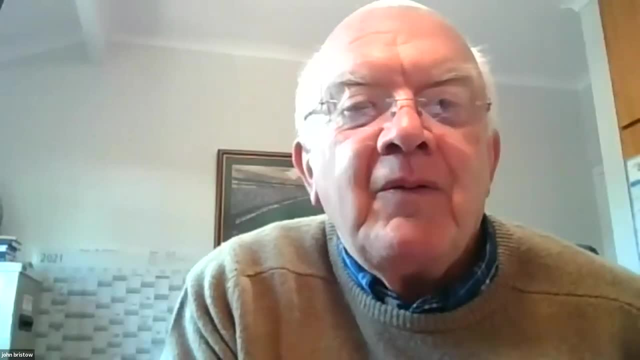 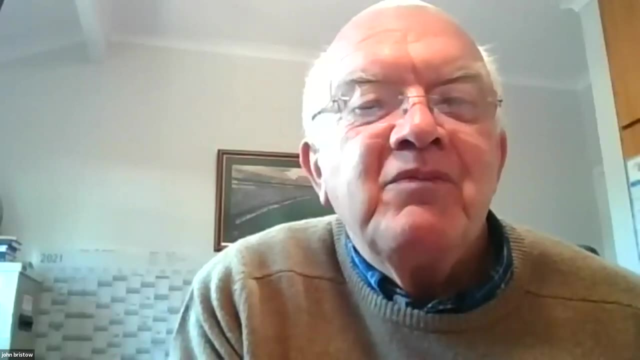 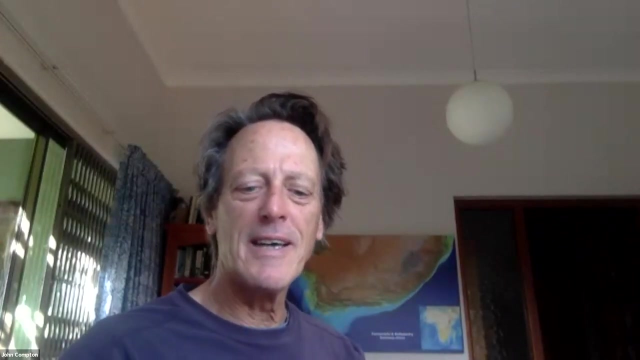 Who wants to kick off Any questions? I have a question, Jon, go for it. Thanks, Stephen, for that very interesting talk. It was nice to be brought up to date on things like the Clan William Dam, which I've noticed. they've got all the equipment it looks like there and the cement making stuff. 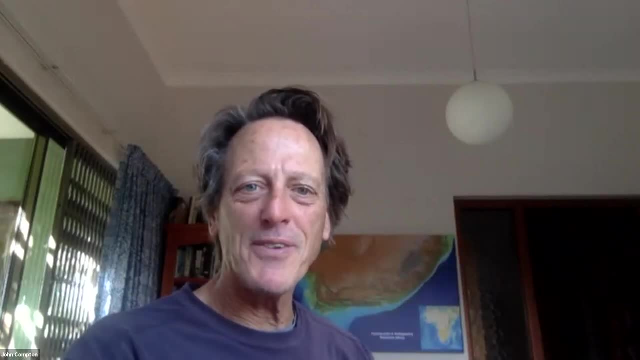 Everything looks good to go But, as you mentioned, nothing's happened And I am sort of curious if you know what sort of holding ultimately holding that up. I suppose, as you said, it's the money. you know that they're having trouble raising all the money. 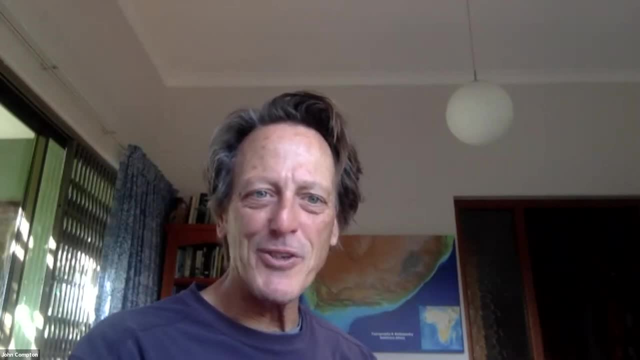 But it looks like they're really on the verge of starting. You know, it seems like an odd situation there. And then the other thing I just wanted to comment on was the phosphate. I think this is very interesting for me as a scientist, because we've often been interested in phosphate, both offshore and onshore. 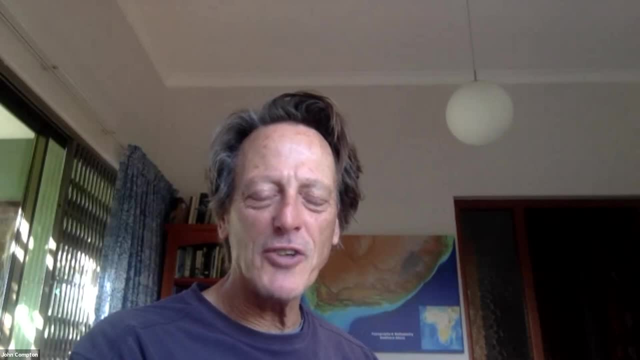 And if you look at the old 1 in 250,000 geological map, they have little spot soil analyses of phosphate In the soil And it's quite high. I think that's how they define that whole region that you showed. the hatch, the purple hatched area, was defined on the basis of really quite unusually high phosphate in the top soil samples that they took. 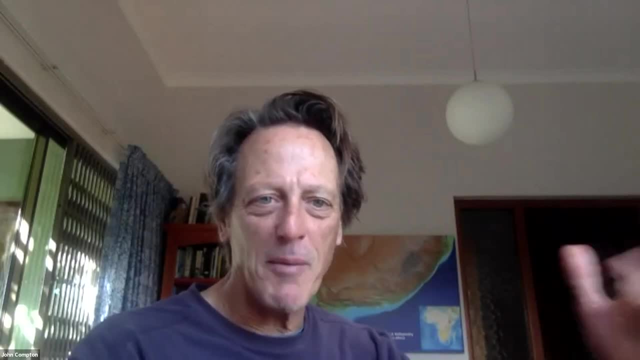 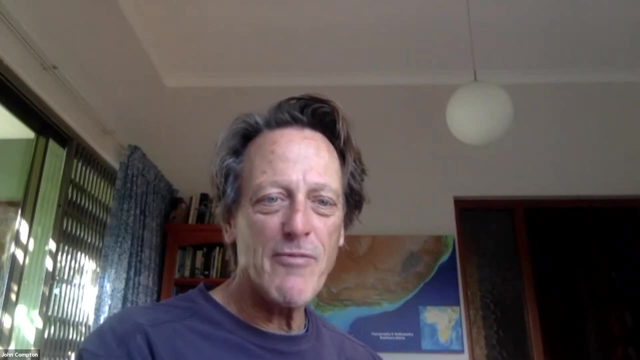 I think it's sort of random sampling And it's not a huge number of samples, but that's how they sort of defined it. And then I guess the idea is that there's the potential for phosphate deposits at depth Right. That's the. we don't really know where these phosphate deposits might be. 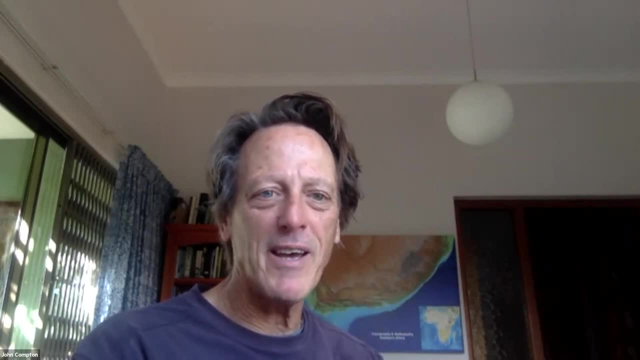 I mean obviously historically the Kempfoss mine at Langebandeach, now the West Coast Fossil Park, was the big one And now the Ylansfontein site is potentially going to be developed or has been developed And I guess there's a sense that 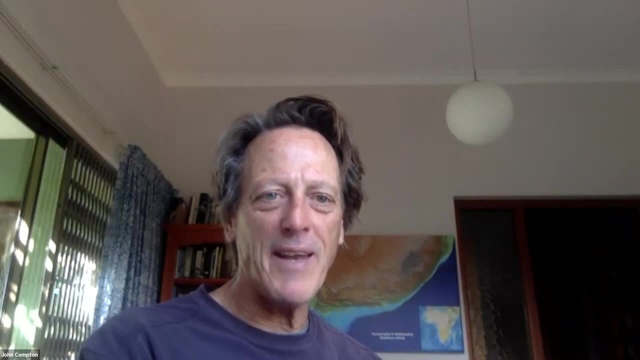 There's the potential throughout that area- not everywhere, but certainly within that corridor- that's maybe sand covered or whatever- that may contain deeper, more rich phosphate deposits, which is kind of intriguing. So anyway, those are just my two comments. So I don't know if you want to follow up at all on the Clan William Dam and what's holding that up. 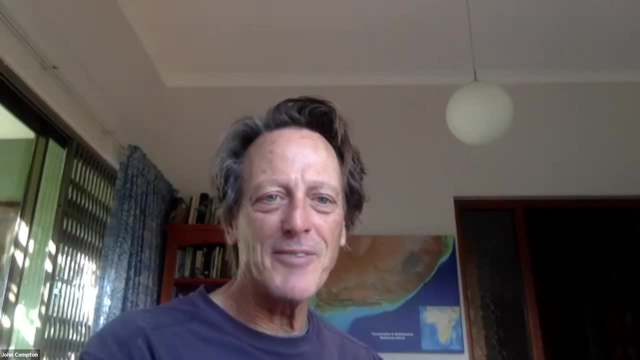 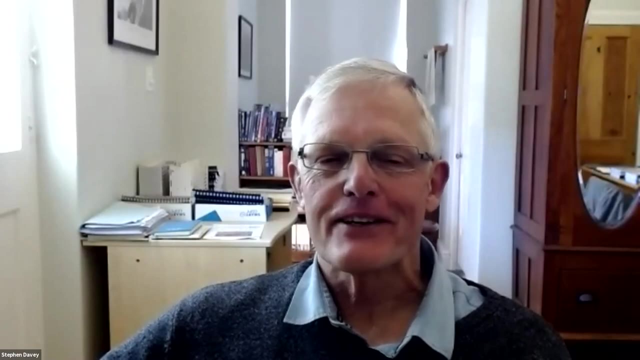 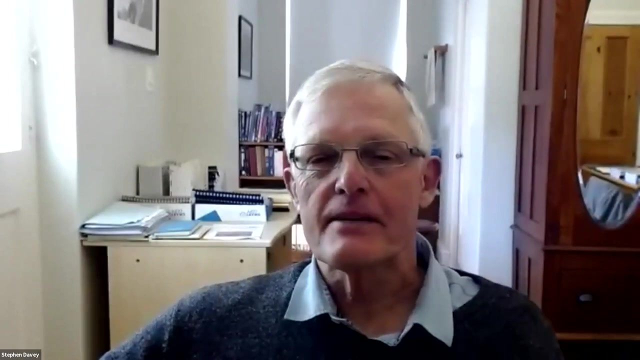 And also any other thoughts on the phosphate. Thank you With the Clan William Dam the Department of Water and Sanitation. I think they've spent their money on other projects and they just don't have the funds at the moment And I understand there's some very frustrated people that are on that project and just sitting around in Clan William waiting for something to happen. 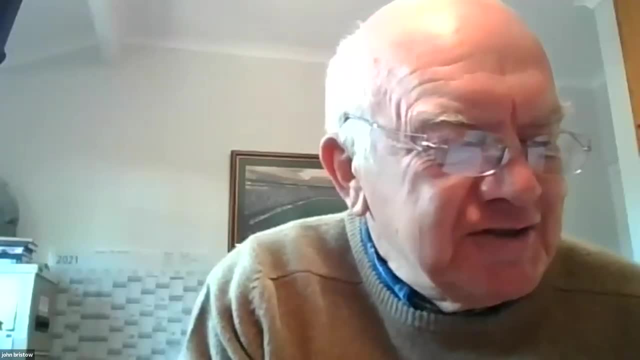 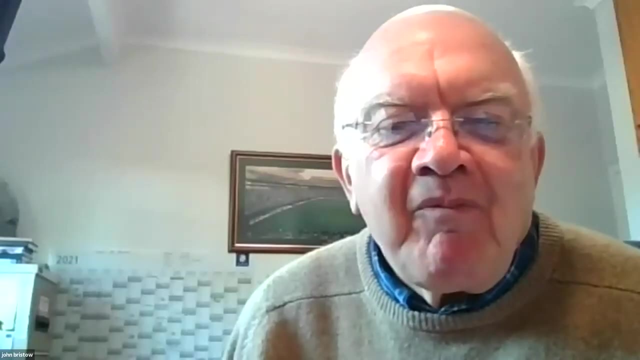 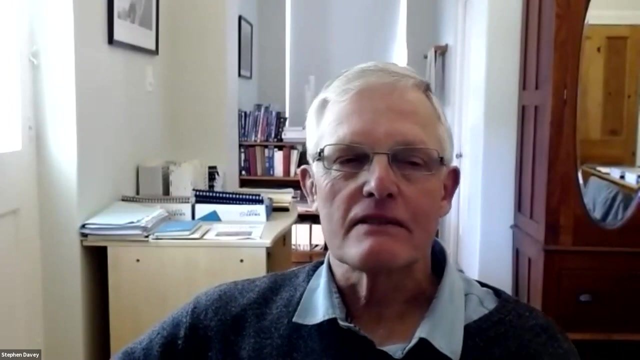 Stephen, be polite. I understand that that money has been stolen a couple of times Anyway. Then with the phosphate, actually there's been quite a lot of exploration that was done. Salmon Coal and various other companies trawled in the Sordana Bay area, you know, as far back as the 60s. 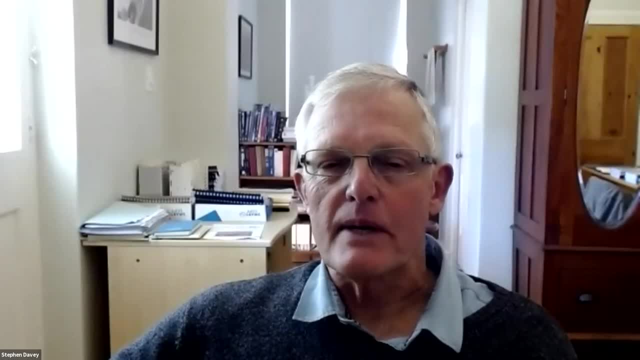 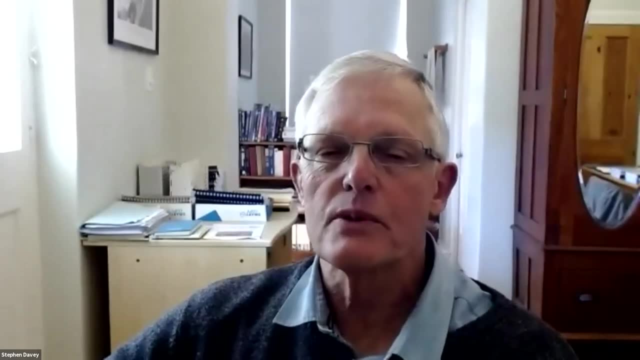 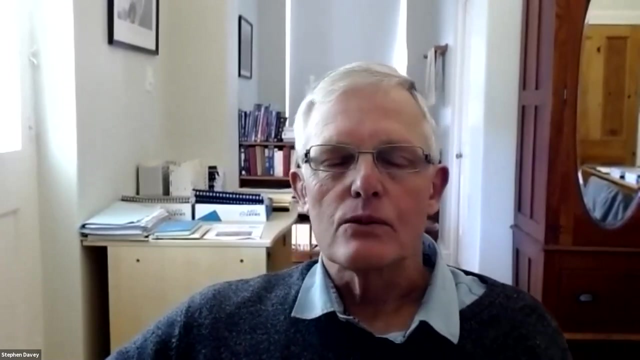 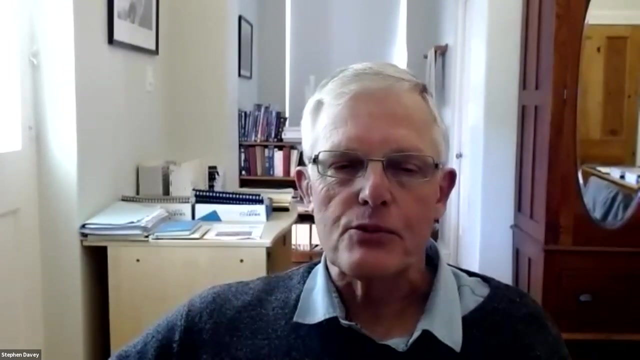 And so most of the deposits that are known are known. I think there's one at a place called Baker Island And there's one between Friedenburg and Friedenburg and Sordana Bay And one heading out towards Paternoster And all the rest. you know, the town planners don't really know the difference between the mineral currents and the mineral deposits. 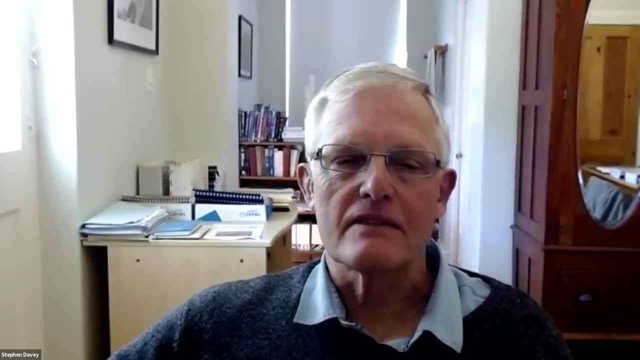 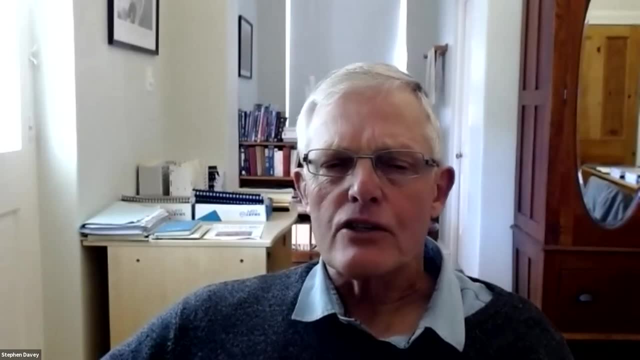 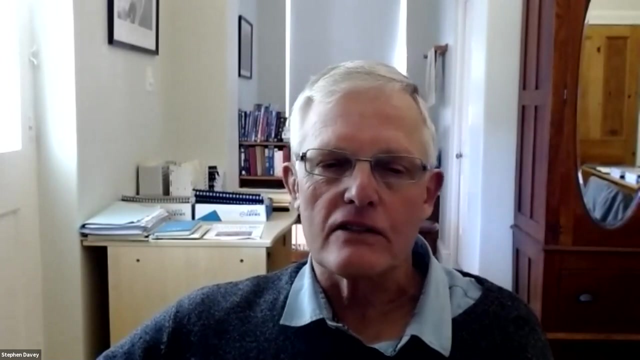 So you know, a small amount doesn't necessarily mean a mine, And so, from the available information, there are two or three other spots apart from Jyllandsberg And the fossil park that could be looked at, but it's certainly not wall to wall covered in phosphate. 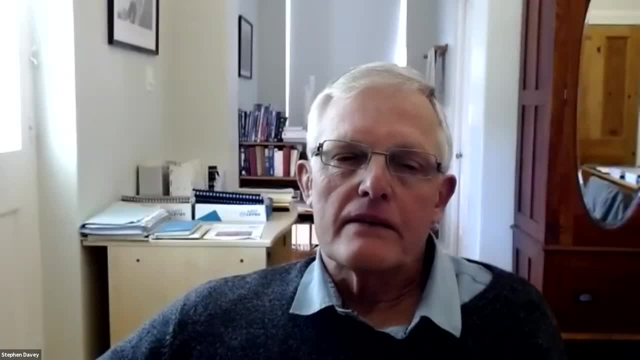 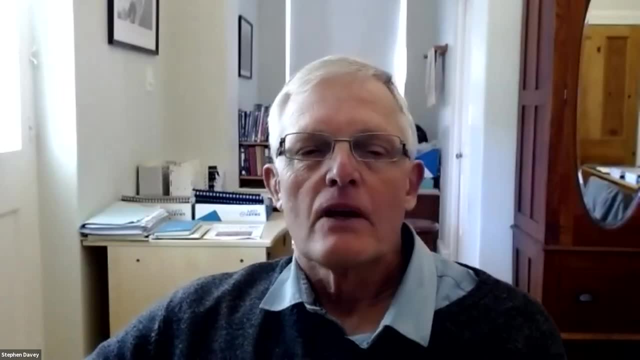 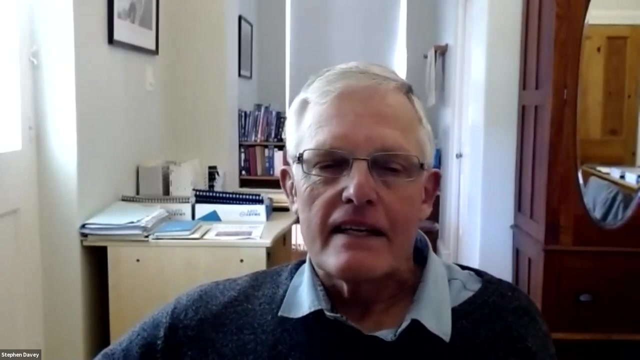 And the other thing is: you know the amount of information that's been obtained, paleontological information from the fossil park, which was a chemphos salmon coal bulletin mine. Nowadays it's almost as if the mine is not appreciated. 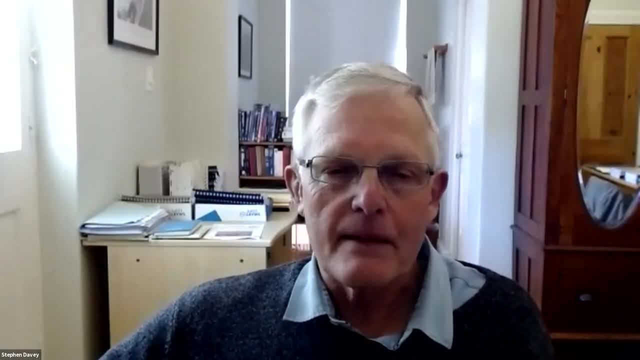 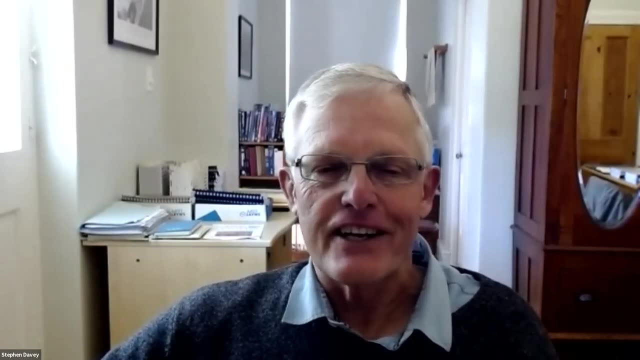 Because if there wasn't a mine there, then they wouldn't have been able to find all these amazing fossils at the fossil park, you know. So it's sort of like a chicken and an egg. Yeah, that's a very good point. 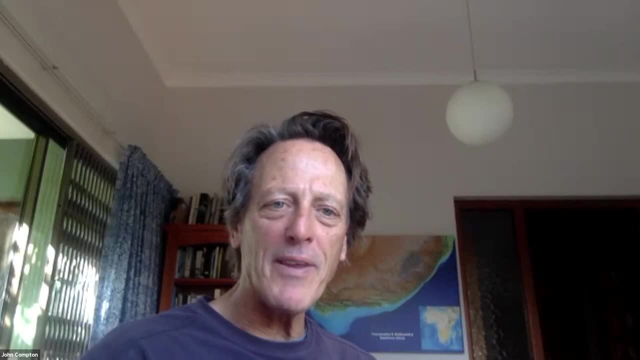 And that's when they were very concerned about the Ilungsfontein mine. I said: well, who knows, Maybe they'll find another great fossil deposit And it'll help fill some of the paleontological gaps on the West Coast, which might be very interesting. 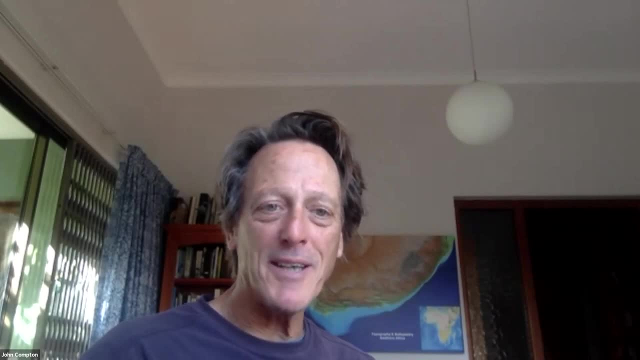 But in the end you know they haven't mined it enough yet to know how much fossil material might be there. But I agree with you that the mines are certainly one way to discover, you know, deposits that otherwise never would have been known. 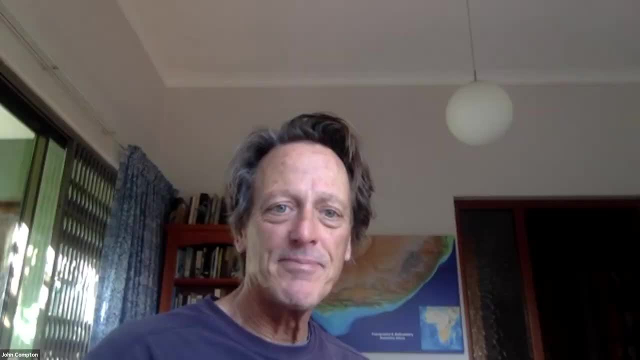 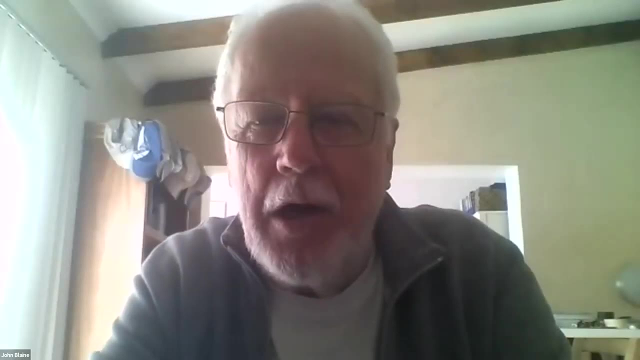 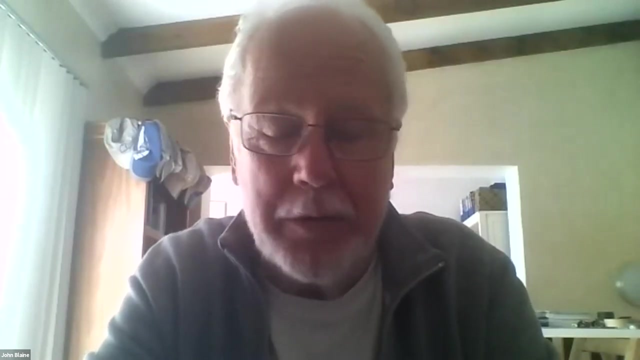 Spectacular deposits, Exactly. Thank you, John Blaine has got his hand up. Thanks, Eddie And Stephen. it was an eye-opener to me. I must say The volumes that you quote, that are quoted there for just one wind turbine are just mind-blowing. 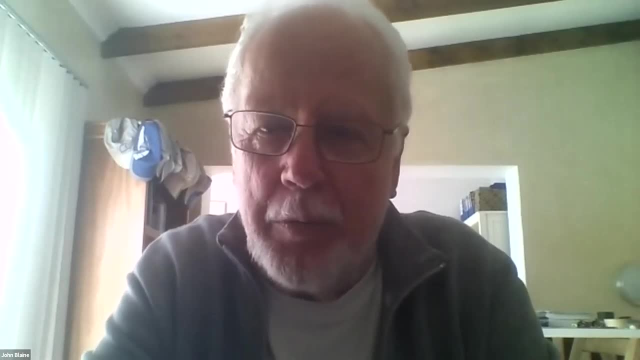 And you see these things going up in the Karoo, you wonder where all the material is coming from as well. But just two main things. I want to comment on Your very last slide, I think from Sandby was quite an eye-opener. 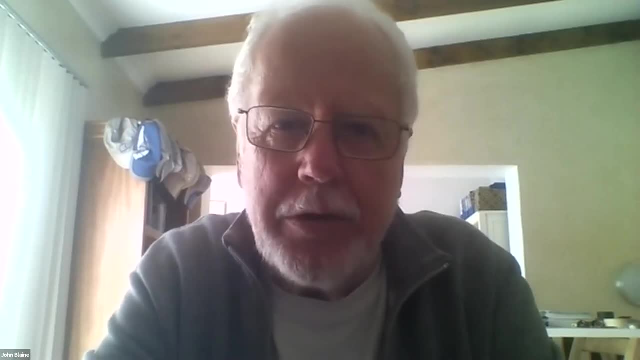 Unless I really missed it. it was in fine print, But geology- underlying absolutely everything in that diagram, was missing completely. So that's obviously a glaring error on the part of the geological fraternity and the Council for Geoscience. I think are our primary culprits. 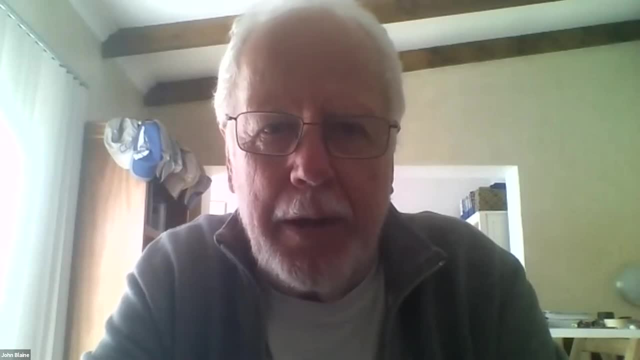 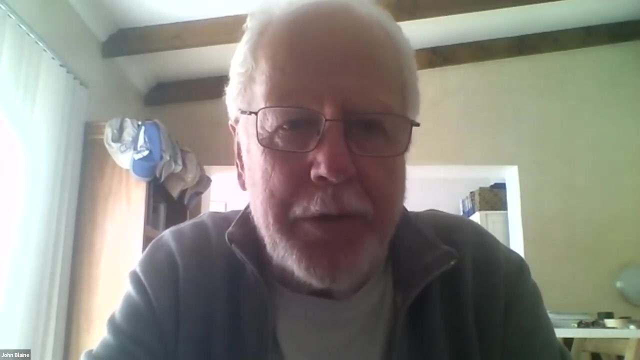 And then I'd just like to quote or point out: my biggest experience of the lack of communication between municipalities and the Council for Geoscience is up in the Limpopo province, at Mokopani, where they allowed the development of an extended township of Mokopani, laid out by the municipality. 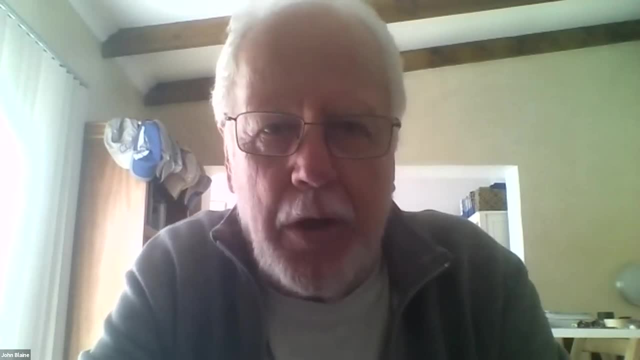 right on top of one of the original examples of the flat reef on the northern limb. Subsequently, there was a lot of drilling that went on right through this township. But of course they could never- this is Ivanhoe- they could never even plan to mine that area. 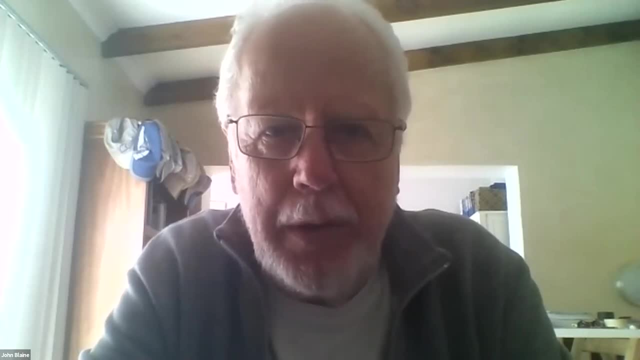 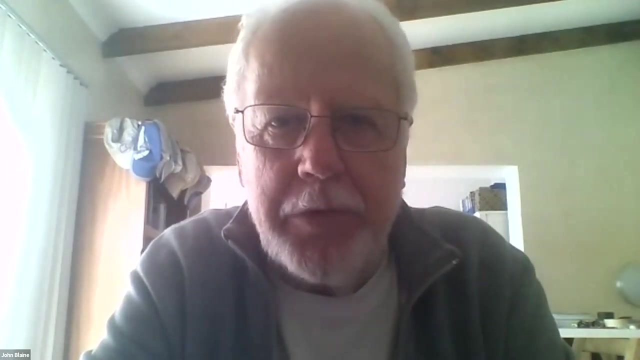 because they had to move tens of thousands of people And even though they went through all the process of, in fact, identifying new ground nearby to this, is the mining company to relocate these people. that was never going to happen. So, as a result, there's a sterilized mineral resource there which could have been a huge benefit. 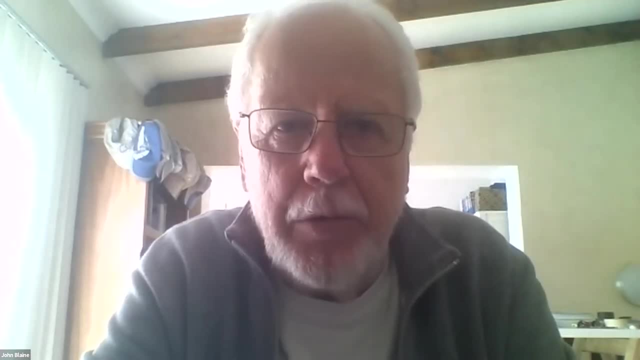 not only to the community but to the country, which, through lack of planning and communication between the Council for Geoscience and municipalities, which is actually just dead in the water. The only positive upshot of that is that Ivanhoe had to drill further down. and discovered a completely new deposit further down dip, which they now call flat reef, typical Ivanhoe style, which is on the card some stage to be developed, But there is nonetheless a huge near surface open cost resource which is never, ever going to be mined. 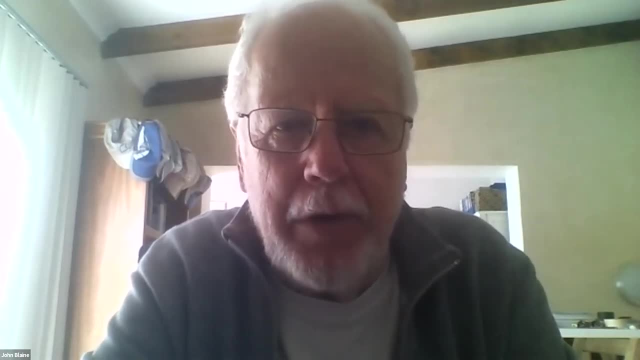 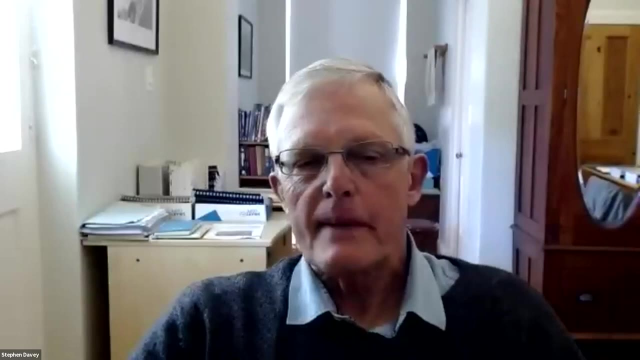 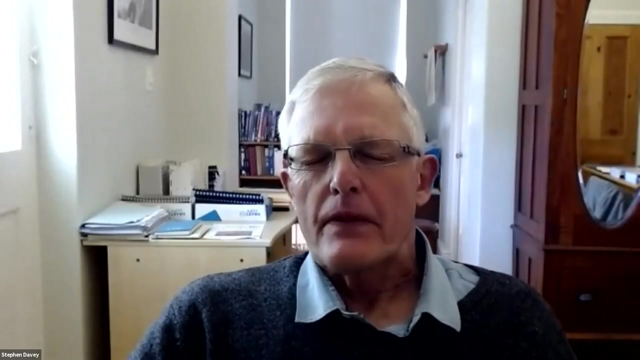 And I think the Council for Geoscience really has to do that. The Council for Geoscience really has to take the blame for a lot of that. I agree, The municipalities need to take the mineral resources into account, And it seems to be that they think that the mineral resources are a national competence. 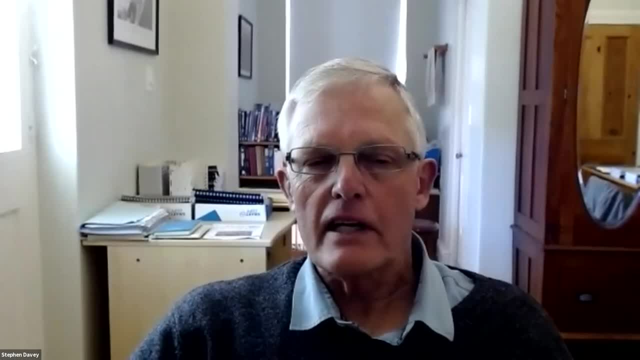 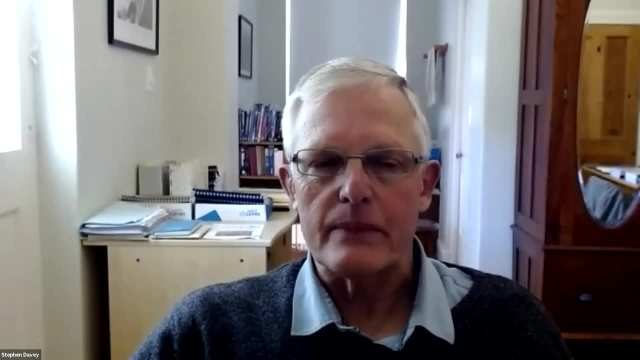 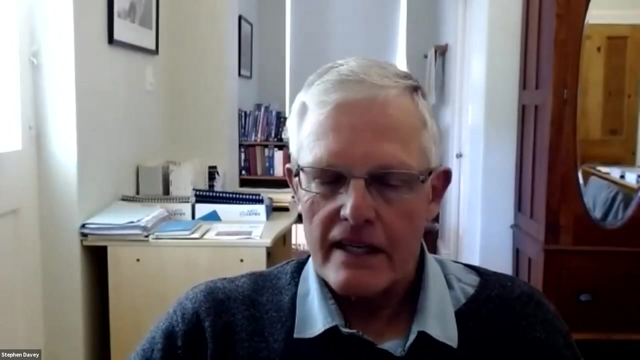 And when it comes to mining, they're not really interested until the moment that somebody puts in an application and then they suddenly want to patrol it. But they're not taking responsibility for the planning of it, But it's just when you apply, then they want to be in charge. 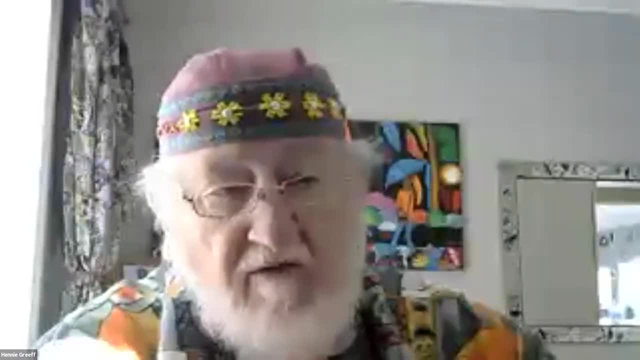 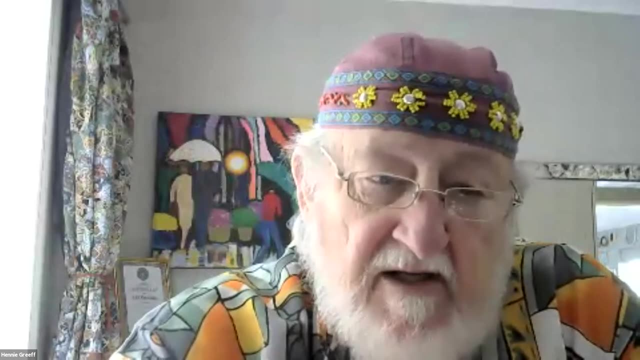 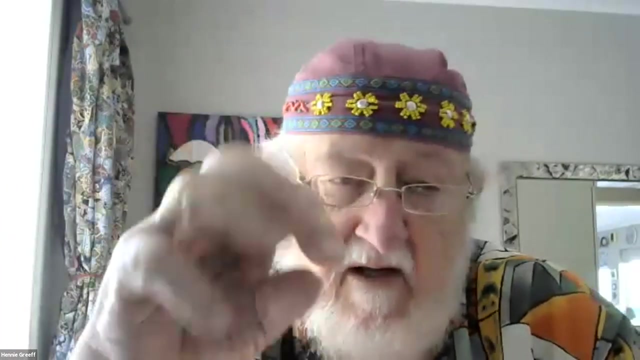 How do you suggest we go forward with this? Would we be putting pressure on the town planners to incorporate something like a building factor and saying, look, in the next years we're going to be building so many houses, we'll be needing so much building materials, and maybe put an incentive factor on this? 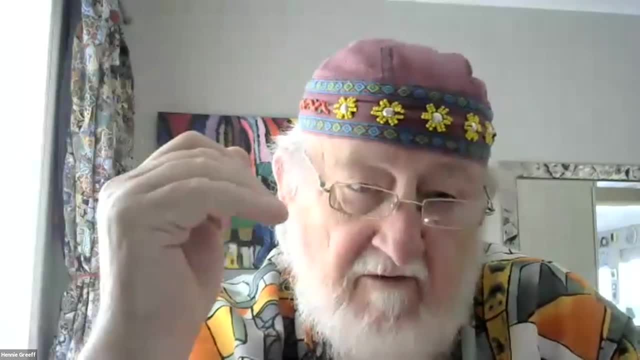 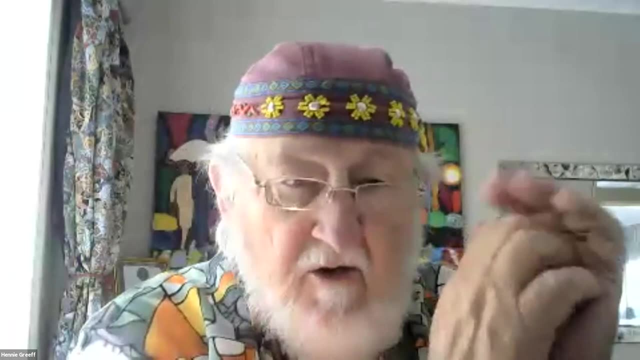 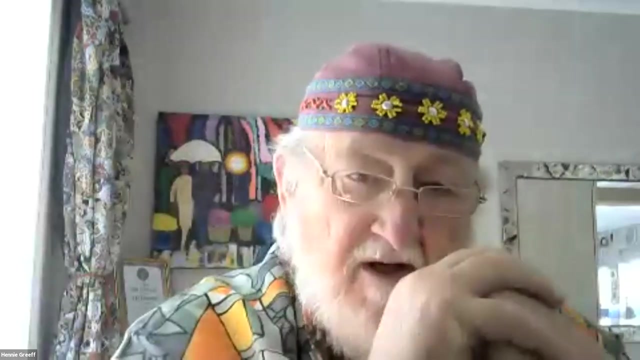 say, for instance, sand, If you come with a license and you say I'm so many miles from the source that you actually get a plus. So to put pressure for them to start planning how much the volumes are and then by that means put pressure on geoscience to provide that information, 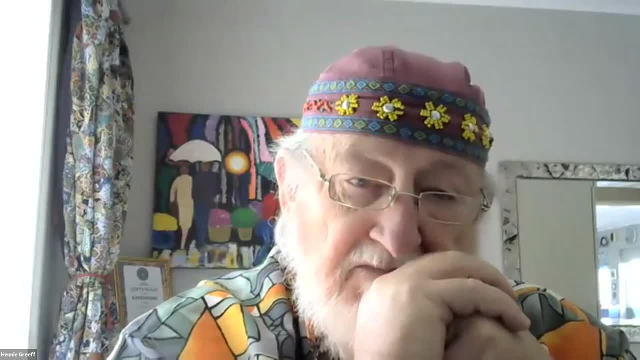 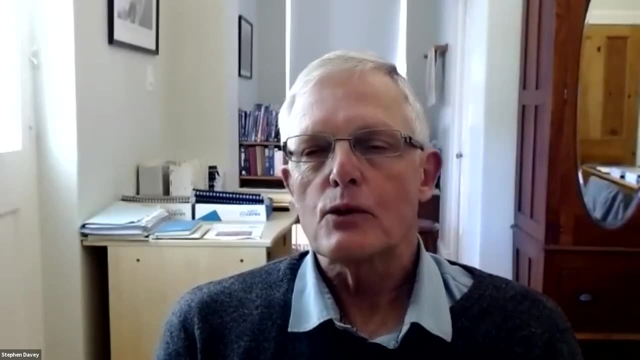 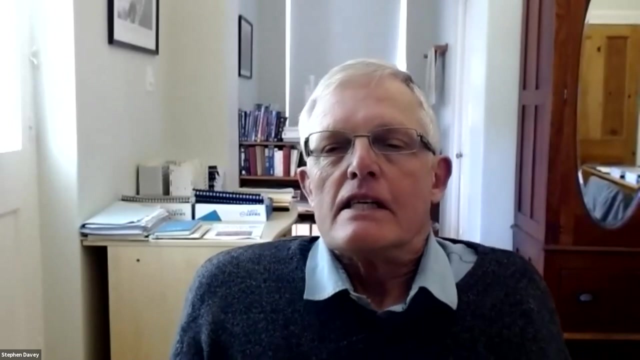 How do you see us doing this? Well, I think obviously the big picture. ideally, you want your Council of Geoscience to be more active and more proactive, But on an individual scale, in an individual municipality. you guys are in the over strand. 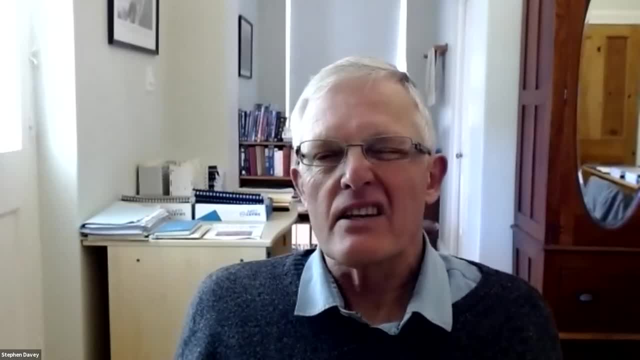 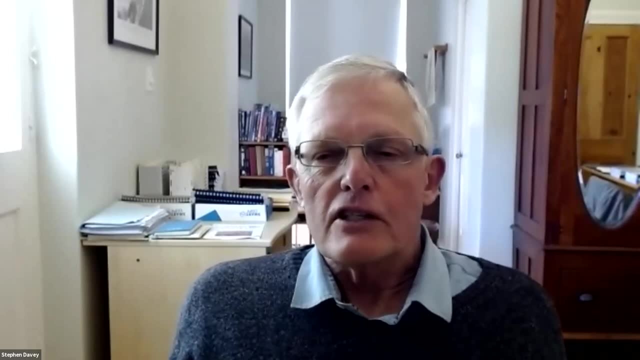 So when these documents come out from the municipality- because I think they have to do a spatial development framework every five years- then it would be worthwhile for the geologists to look at them And if there are things that are missing or things that are obviously wrong, 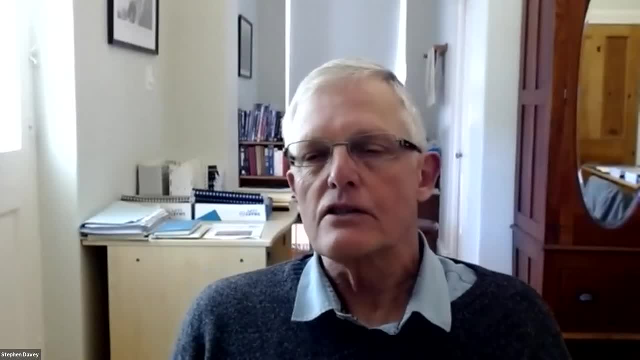 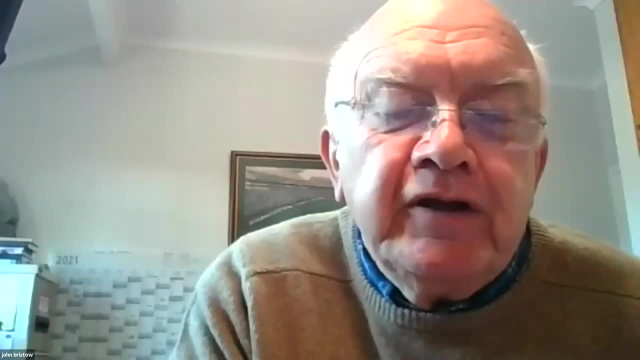 then that's the ideal moment to point it out to them, To point it out to the planners in the municipality. Yeah, Stephen, I mean that's critical, And I think, Henny and John, it all goes back to raising the profile of the profession. 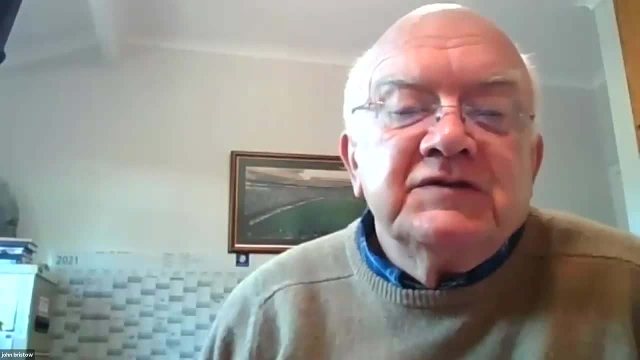 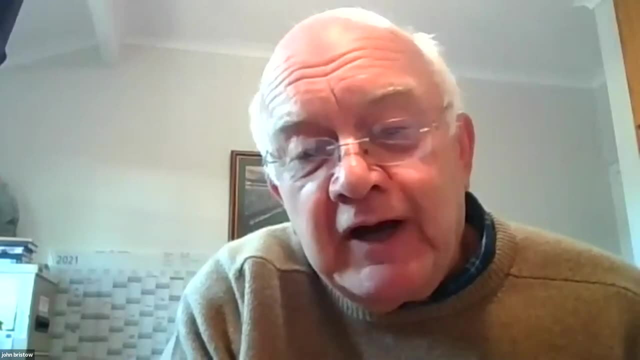 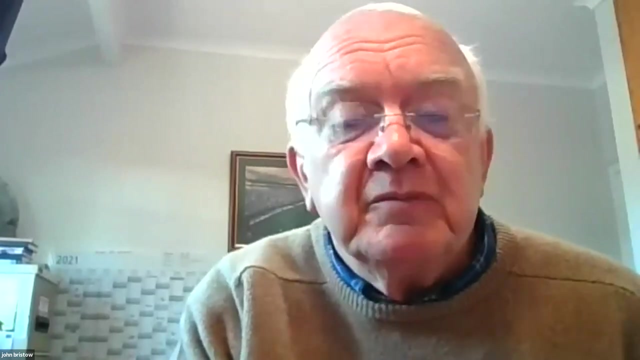 And if you look at us here in South Africa- and I'm on my hobby horse- the geological profession in South Africa is really tarnished by its mining, And mining has made big holes, It does environmental damage, It kills people, And so the image of mining in this country. 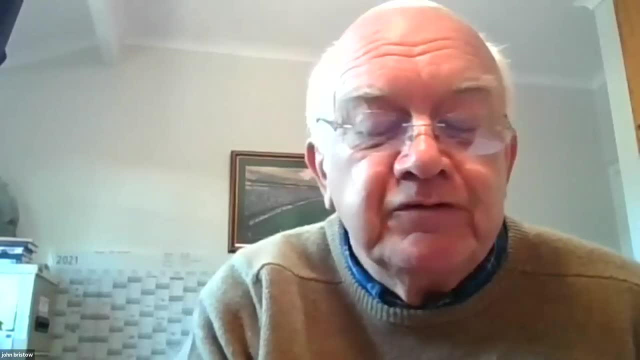 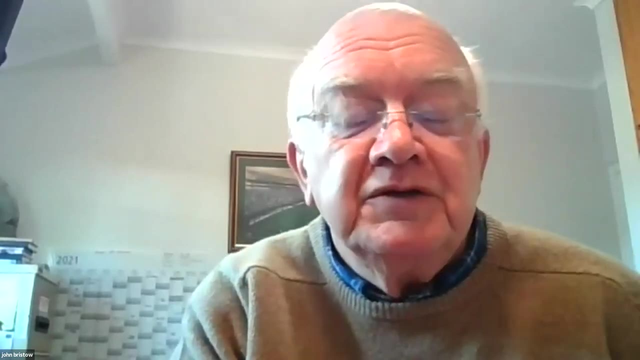 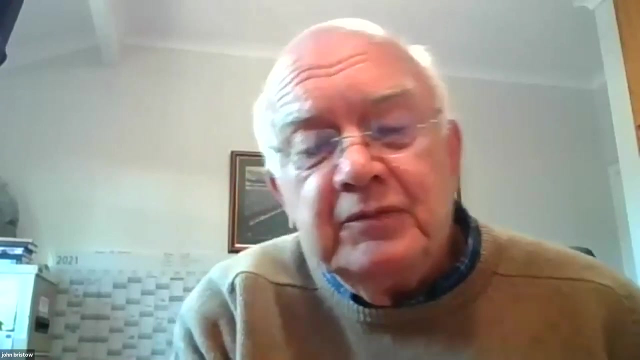 and we then get caught up in that backwash is actually awful, if you want to be honest about it. So I think we as a profession, starting with our professional bodies, really need to look at how we can turn this around, And obviously some of that goes back to geo heritage projects. 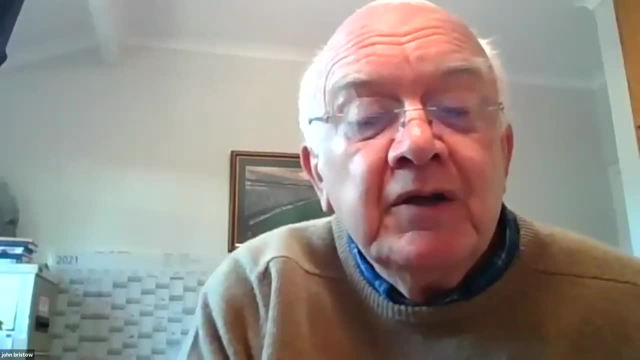 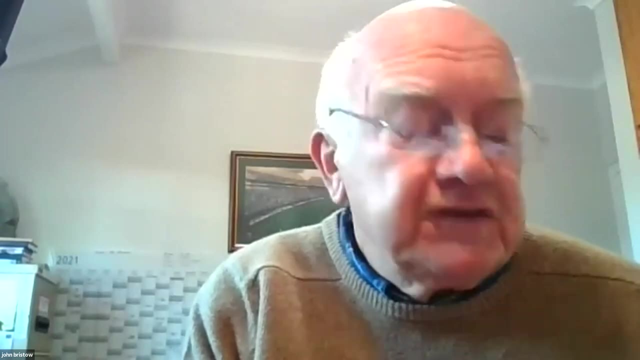 There's a bunch of people on this talk who are involved in geo heritage. It involves getting school kids involved and teaching them the benefits And then just to extend it and I have to leave at 11,. but it's really good, Stephen, that you brought up the wind farms. 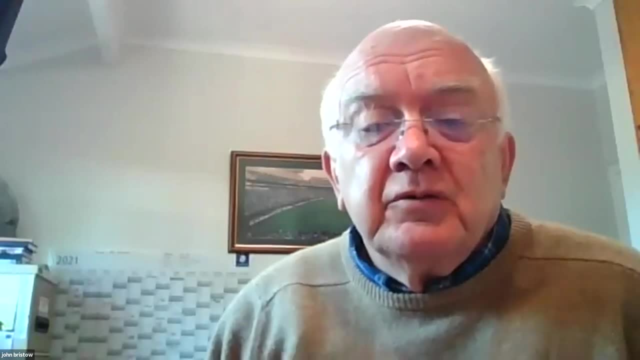 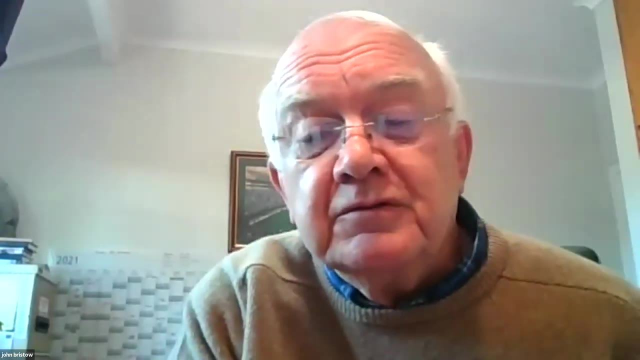 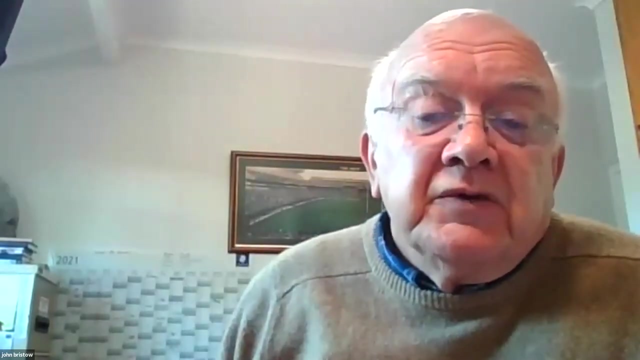 And John commented on it again too- And the footprint that's been developed in the Karoo is actually quite frightening. People should drive up to where did we go, Sutherland, John, and see what's actually going on. What's actually going on there in terms of damage to the environment? 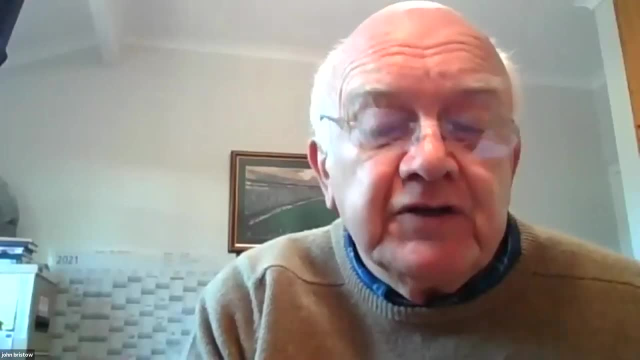 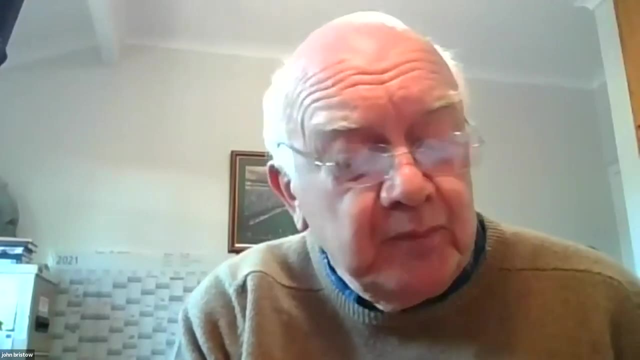 But the other side of it, when you get to climate change, no one talks. I get to see a politician talk about cement, which you, Ray, mentioned, Stephen, And there's a lovely article that was published in The Guardian in 2019,. 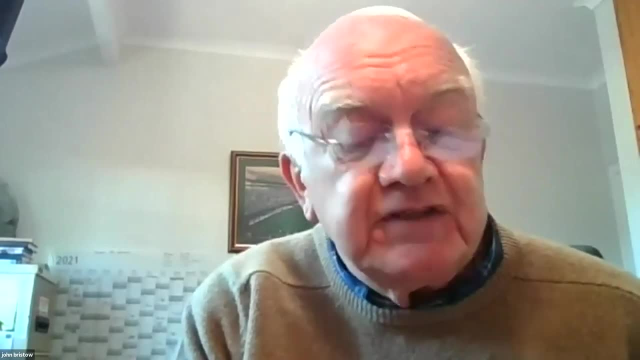 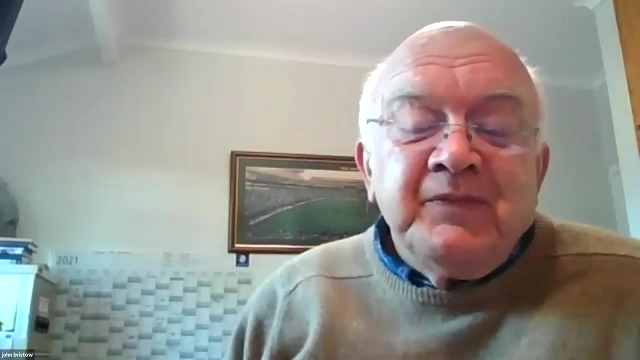 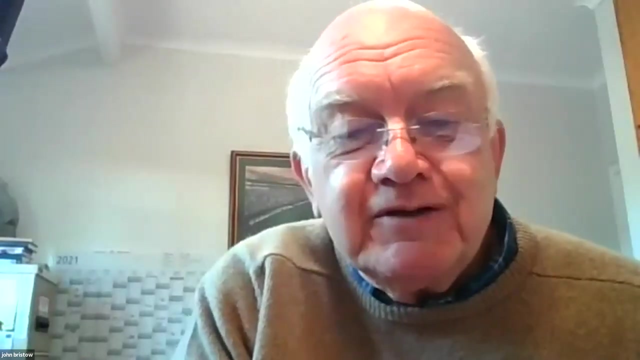 and it says concrete, the most destructive material on earth, And that just gets forgotten. And if you look at those pictures of Cape Town and the flats and all of these popular places around the Cape are not going to stop growing And that needs cement and sand and all these other commodities. 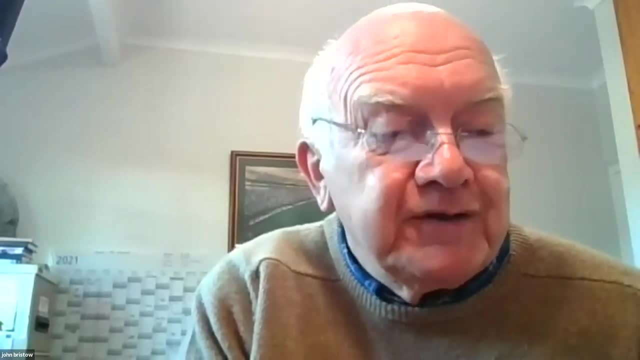 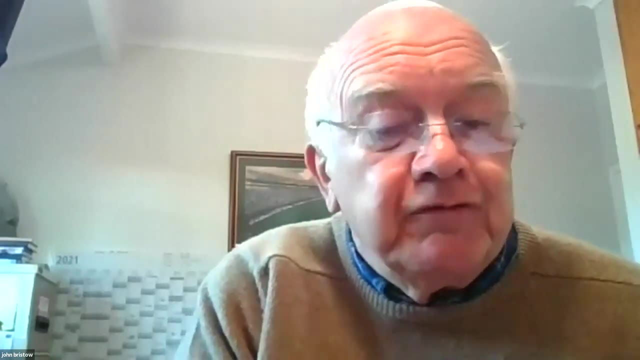 So this view of the world that you're going to stop coal mining and you're going to stop making holes in the ground is just quite bizarre, And if we really want to worry and be concerned about climate change, let's go and look at basic things like cement. 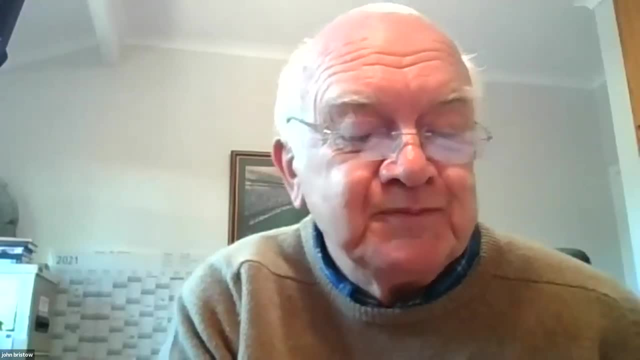 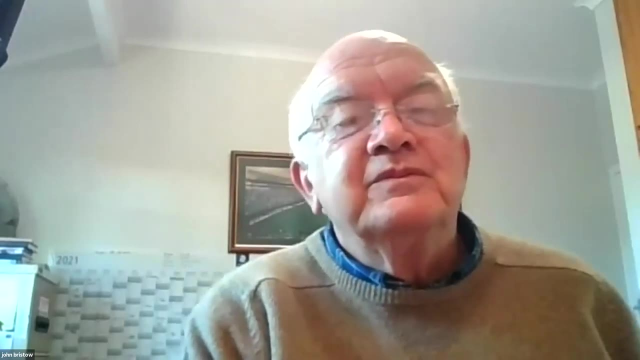 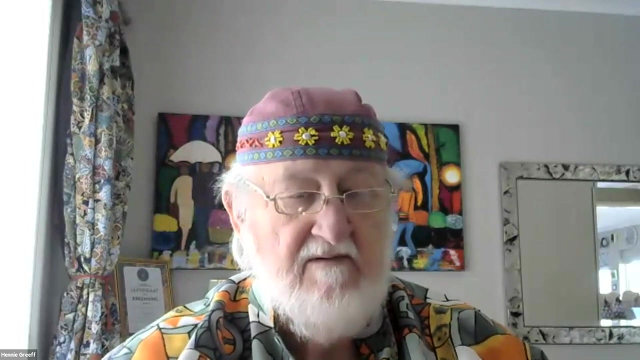 Cement and manufacturing of cement is just hugely destructive. So that's my for the day, John. can you hear me? Sorry, let's just get Dylan a quick one, and then you, Kovacs, Dylan, you can unmute yourself. Thanks. 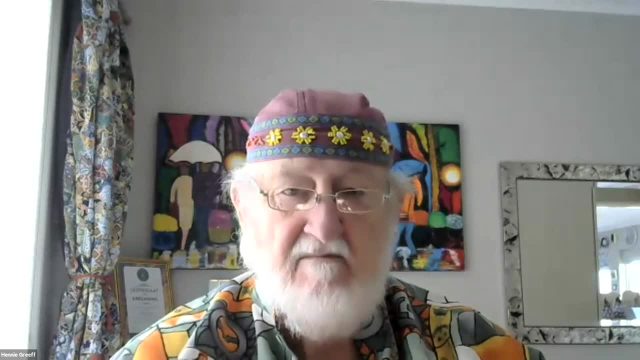 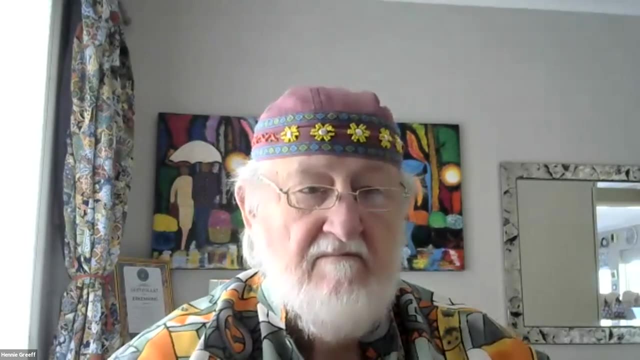 Thanks, Stephen, for the last presentation. Yeah, I think I mean, from what I've seen with a lot of these tenders for the SDFs and integrated investment plans are, yeah, the municipal officials that write the terms of reference aren't really educated. 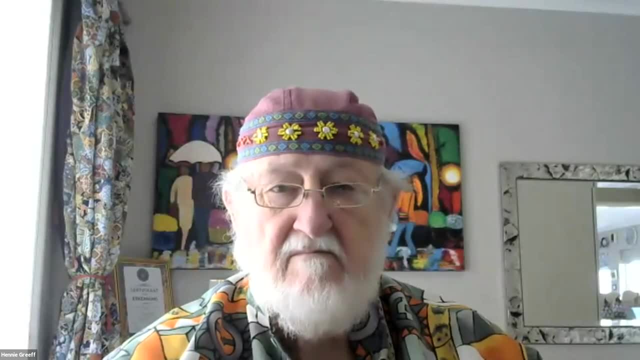 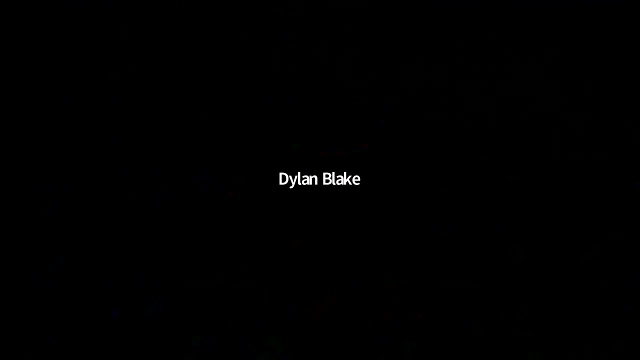 in terms of geology and hydrogeology and stuff like that. So that's why the TOR is always written and focused towards the more ecological and environmental side of things, And that's why the geology and stuff is always left as an afterthought. 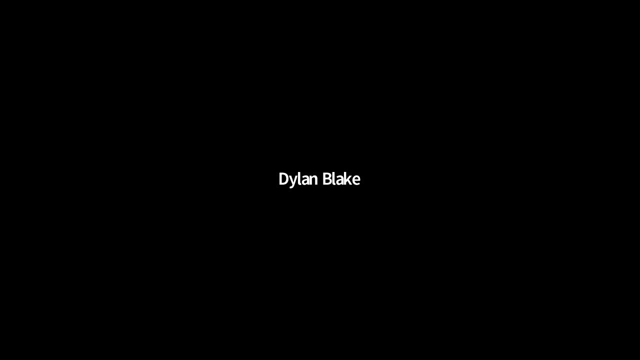 And that's also a factor because the environmental lobbyists are so strong in the country and they always push. you know it's their prerogative, They push what they want to be done. So I think, yeah, I think, if the geoscience community. 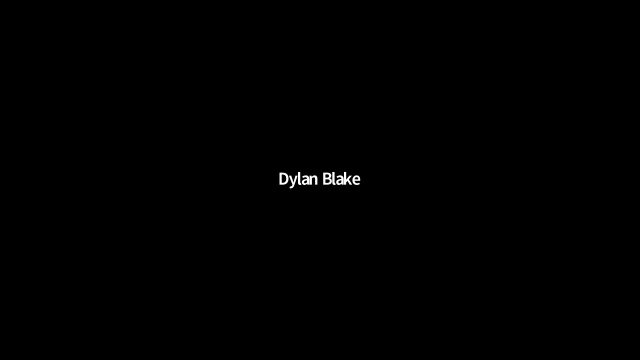 had a stronger lobbying aspect to it and educational aspect, which has been improved, strangely, because of COVID. you know, I saw John yesterday and I was saying you know there's a lot more access to geological presentations to the general public now. Yeah. 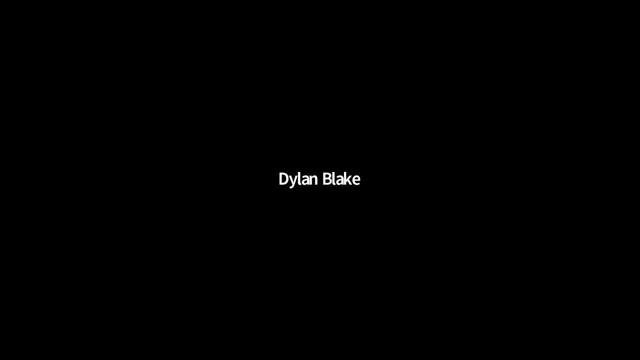 So I think that's an important thing And we've learned that from the various groundwater projects we've worked on- that even educating the ecologists and botanists themselves on geology helps them kind of not be so panicked about developments, whether it be mining or groundwater developments. 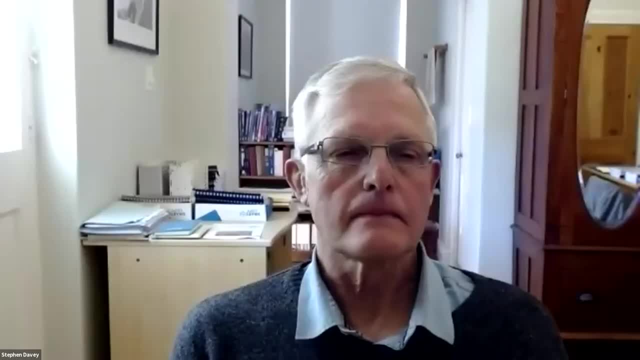 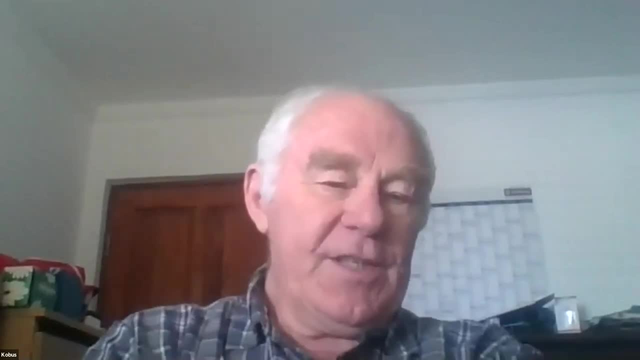 and stuff like that. Thanks, Thanks, Dylan Gwilmis. Yeah, I just want to make a comment on, you know, that point of, let's say, geologists being more involved in, or their input, you know, into, town planning. 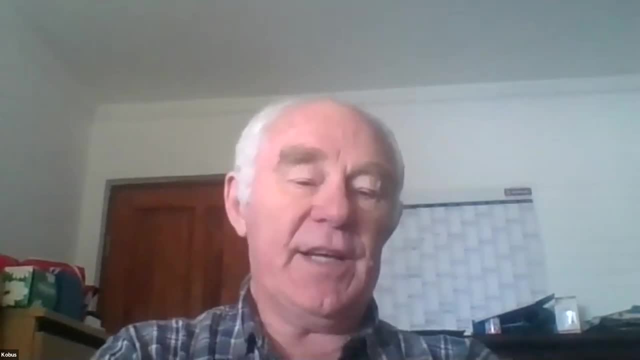 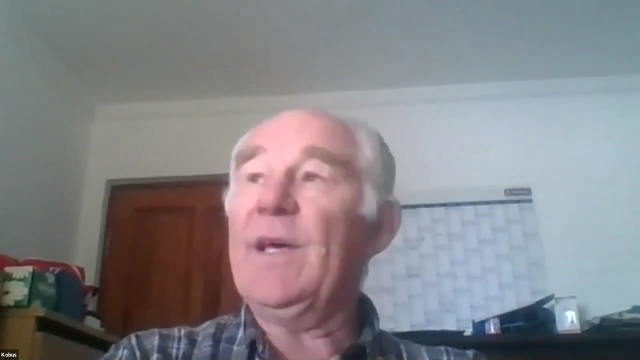 And the one major problem there is that, as I understand it- and I've never gone, you know, let's say to the real sort of bottom end by reading the Act and so on, but I think when they established the Council for Geosciences Act, 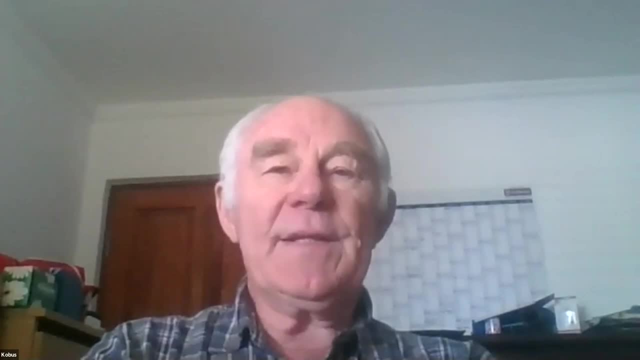 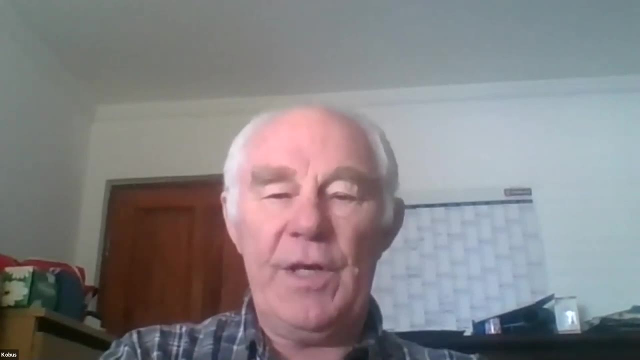 I think the guys there- and I wouldn't mention names or whatever, but the things, what they did is they have some sort of a clause there. I think that no other State Department may employ geologists. All geologists are that give advice to central government. 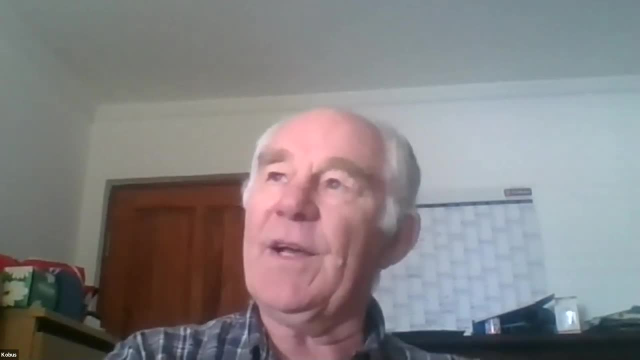 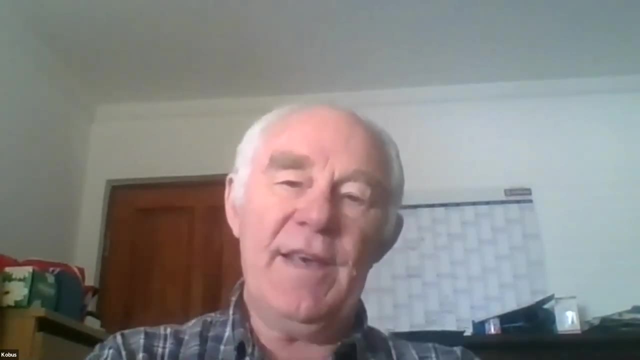 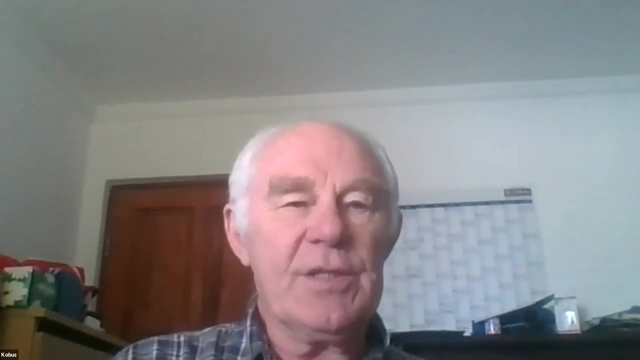 local, provincial government and even local government, I think, are not allowed to be sort of employed geologists. So because obviously they do this whole sort of self-preserving type of sort of thing, They, you know, they want to do all their jobs. 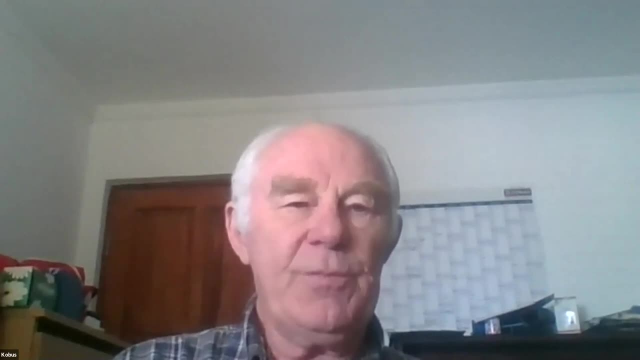 And so what one finds is you know where I would think there should be, at Free State and Gauteng and Western Cape or whatever you know, there should be three, four different types of geologists employed, you know, in the provinces. 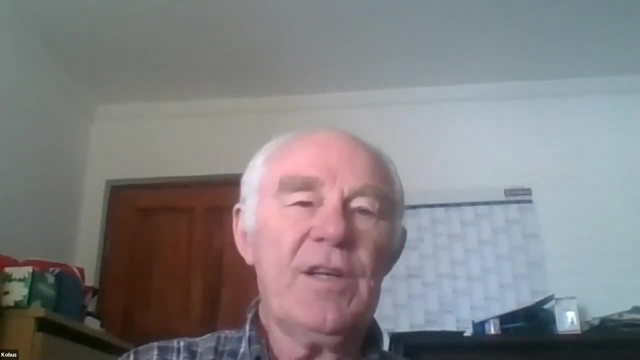 I think you will all agree with me. then there's none. There's not no post for a geologist. I think no one that are actually called or registered as a geologist are actually allowed To be employed in such a position. you know, for a provincial. 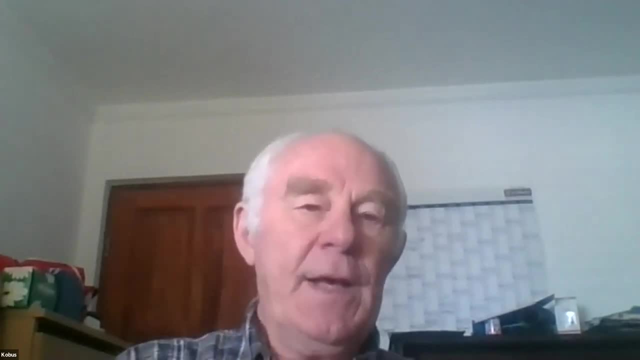 a local government or a central government department, And I think that is one of our major problems, because you know, as myself sort of working in engineering, geology, let's say, for most of my life, you know we find that all the time. 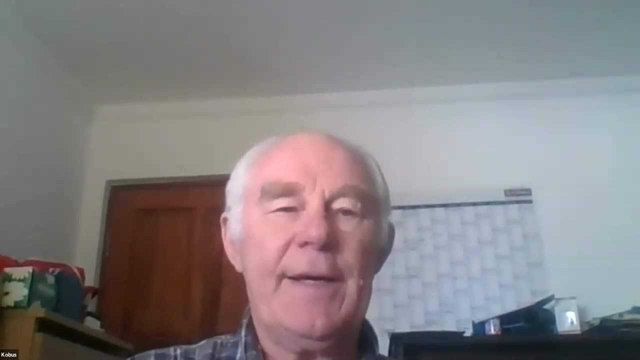 you know that. I mean you are speaking to people that almost don't even know that you know engineering, geology or geology should have an input, you know, into planning and things like that, And obviously how to rectify that on a present condition I don't know. 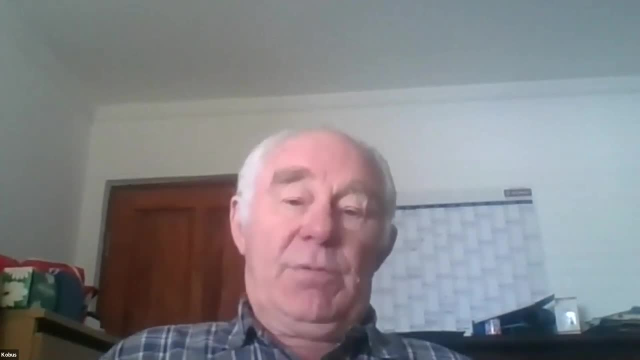 But you know, I fully agree obviously with what is said here And I think that is that you know all these places, you know I would say Cape Town needs, let's say at least, let's say, two or three people giving geological input, and even. 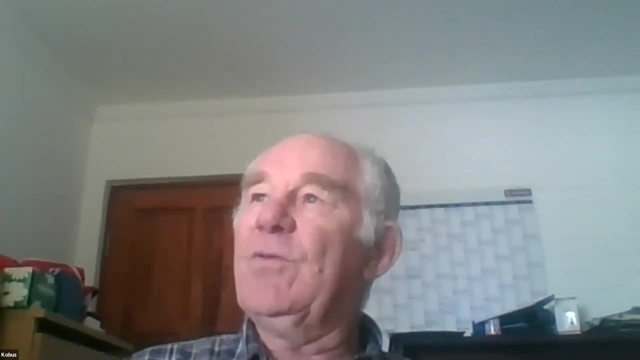 let's say, all these, perhaps even plus some other you know would need, let's say, one, to give input, But at the moment everything rests on the Council for Geoscience And I just don't think that, you know, they can handle it. 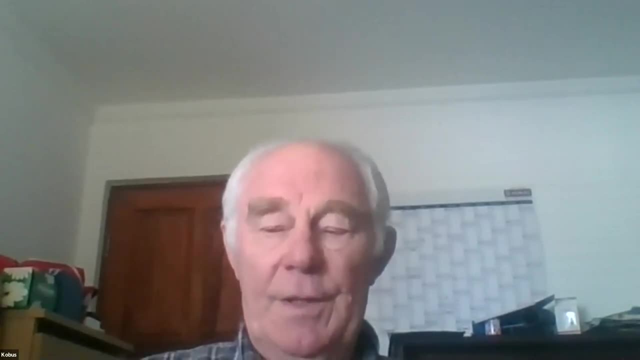 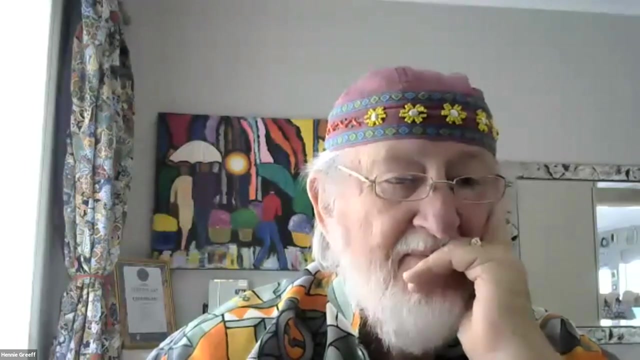 So I think it's a major problem in South Africa. Thanks, Thanks, Koovis. Peter van Niekerk. Peter van Niekerk wants something about water. I hope No, not water, Henny, but I was actually 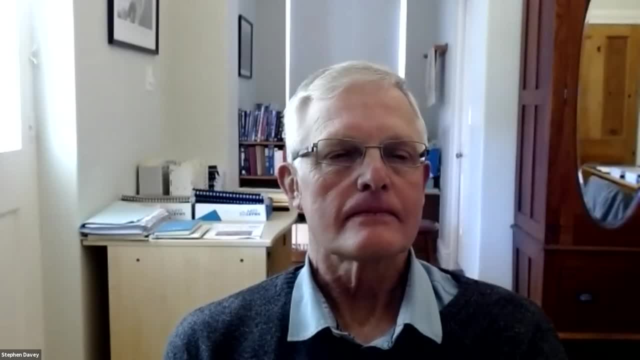 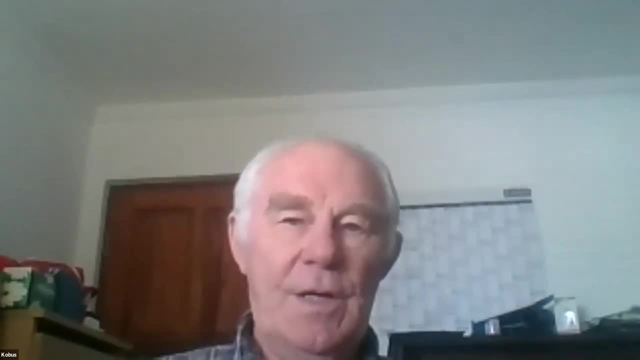 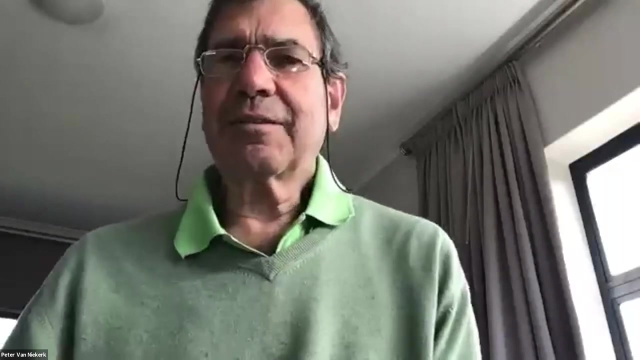 I can't hear Peter. Sorry, Peter, you muted yourself. Am I unmuted now? My apologies, I just wanted to take your hand down and I actually muted you. Sorry, Peter, Just start again. Okay, No, I said jokingly. I wanted to ask whether wine and geology 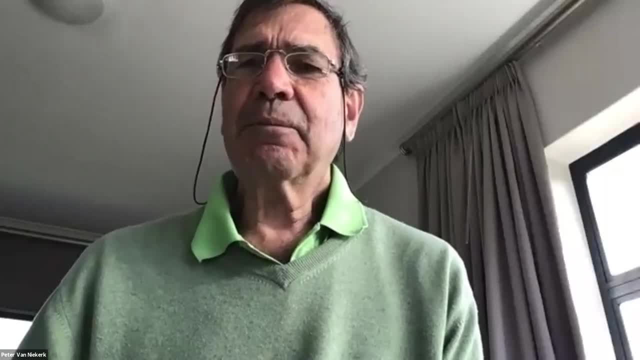 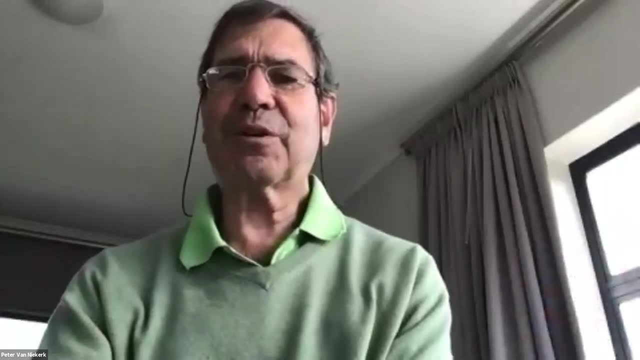 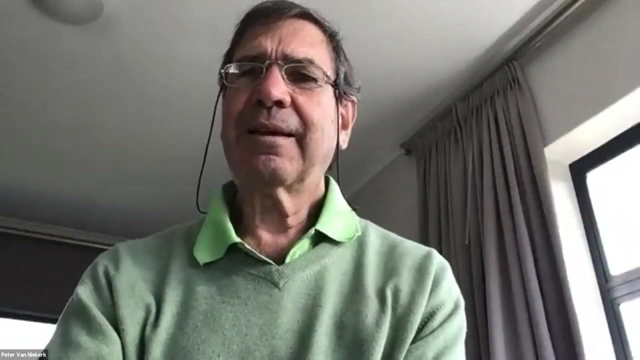 doesn't come together somehow as well. But, more seriously, I've known, you know, many of these talks of- and I'm an engineer, I've come from a completely from a side, another side, But listening to you, geoscientists and the many very serious issues. 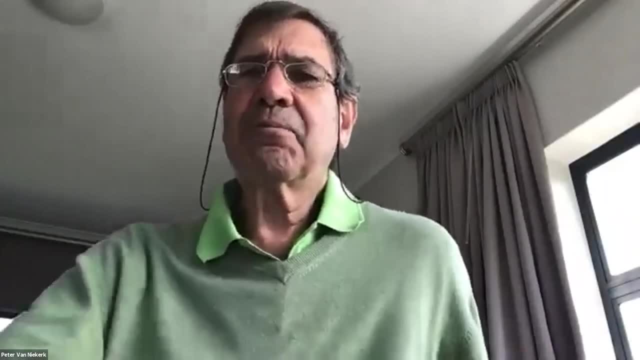 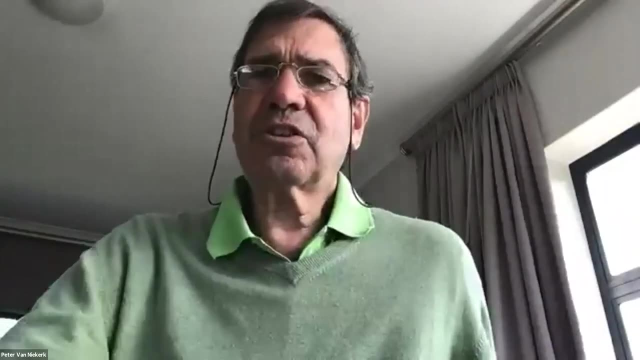 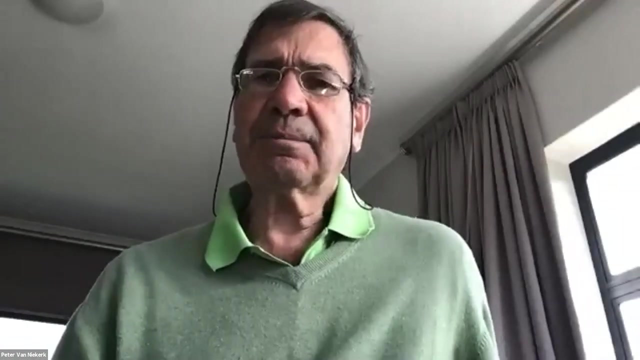 that you raise, like today, with the issue, for instance, of the spatial development that doesn't include geology and the mapping, et cetera, as you would like to see it. I was wondering whether there isn't a mechanism of entering the information at the right spots or the right places. 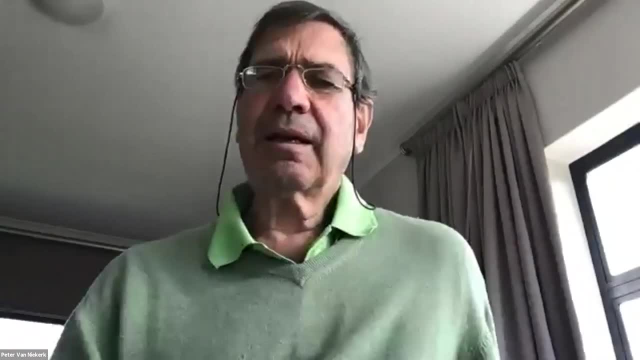 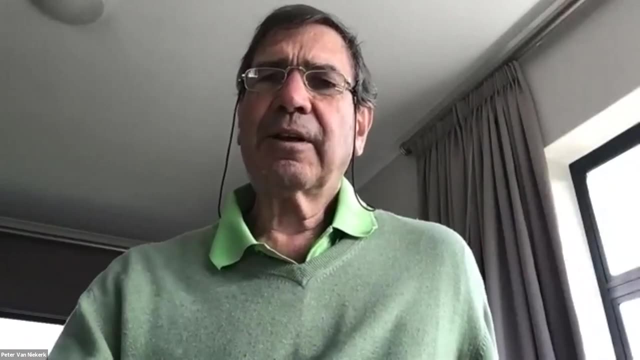 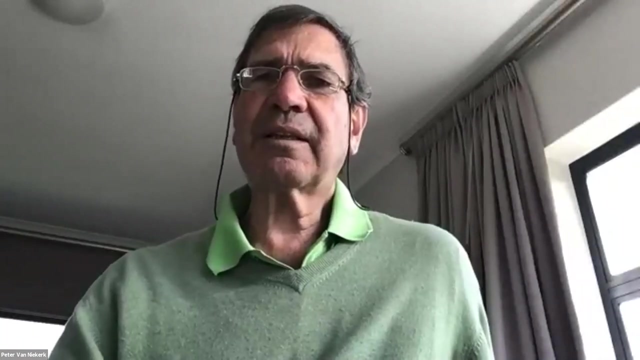 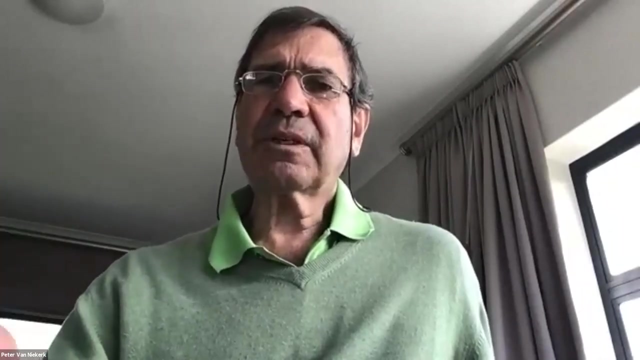 at government There is. I'm not sure whether the geological sciences is a subset of the South African Academy of Sciences, for instance, whether there isn't an avenue through the academy to actually write letters to the president or the minister, The appropriate department, and say this is a serious issue that you have. 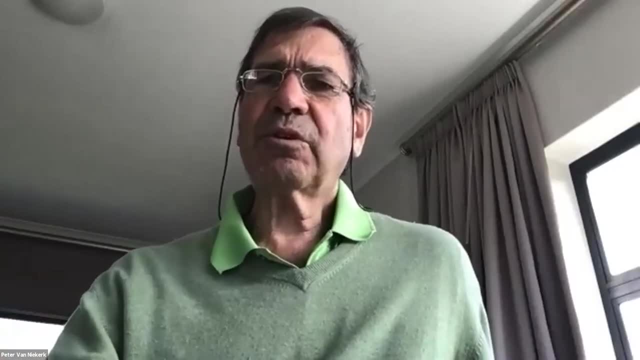 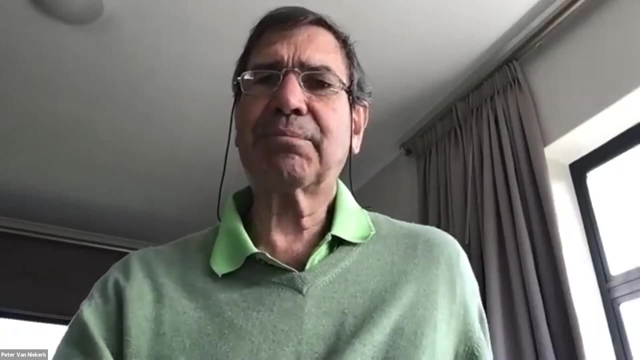 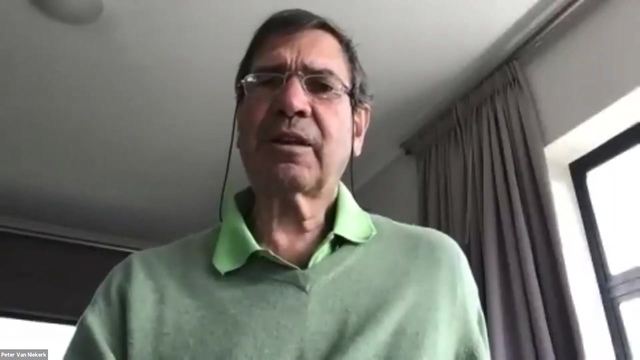 and put it into a two or three pager in a Saxon form And then, and also to then put it out in the media, that had been done. This is what we do from the engineering side. We have a South African Academy of Engineering. 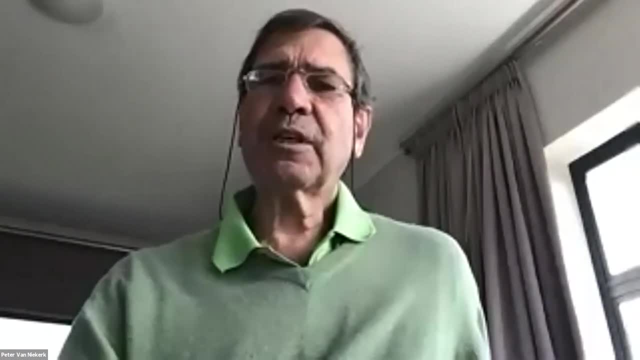 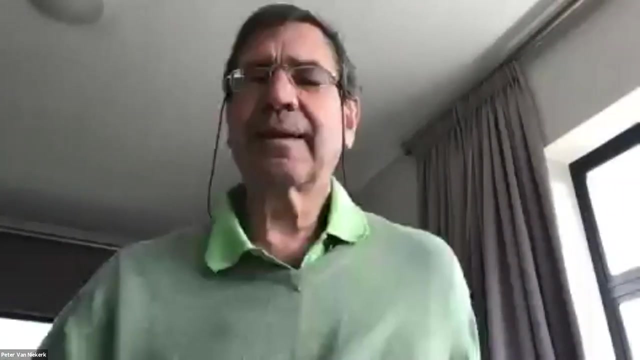 If we feel strongly about something, then we put it down into such a paper and we send it to the appropriate politicians And they may be directed generals of the departments that are that have to be targeted. So I'm putting this to you. 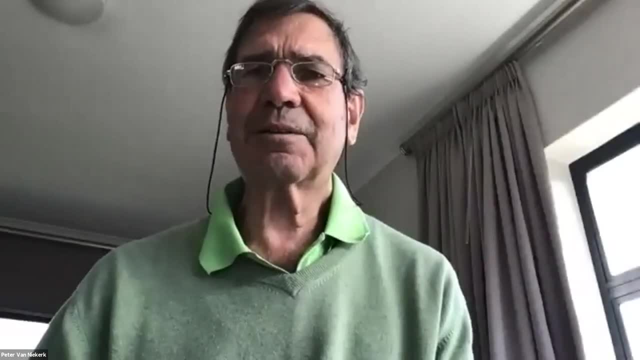 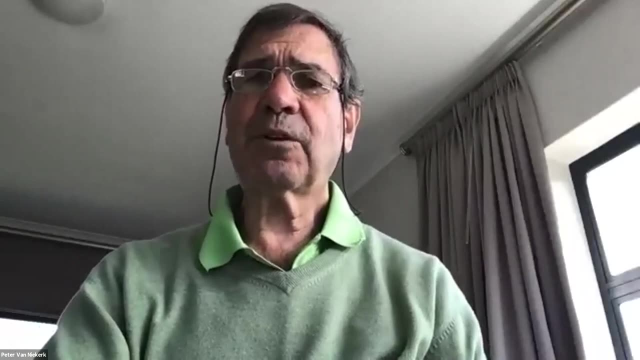 And unfortunately, John is not with us any longer. he's left, But I would like to think that that is something that the Oberberg geoscientists may want to follow up on. Thanks, Thank you. Thank you, Peter Dylan. 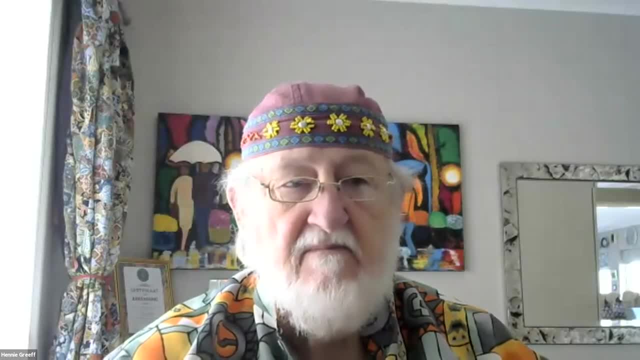 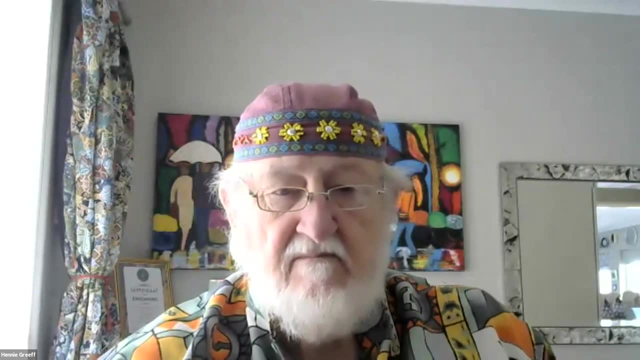 Yeah, I think Peter is correct. I mean we have the GSSA, but I mean, yeah, the GSSA was always, has always been- more focused on mining, I think. But I think it's starting to change and move towards more pressing issues. 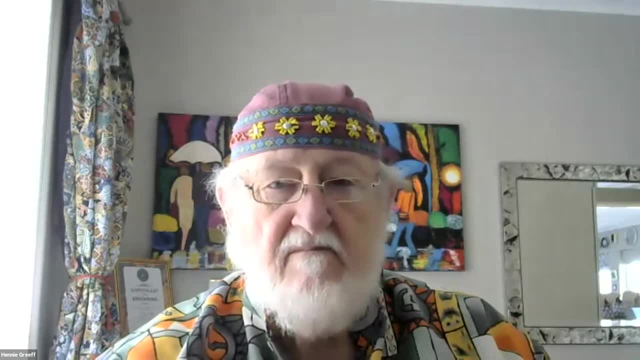 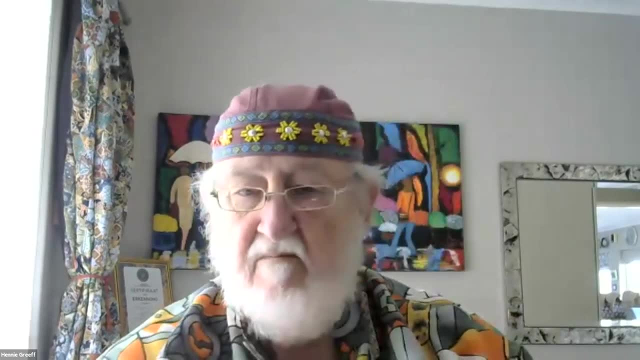 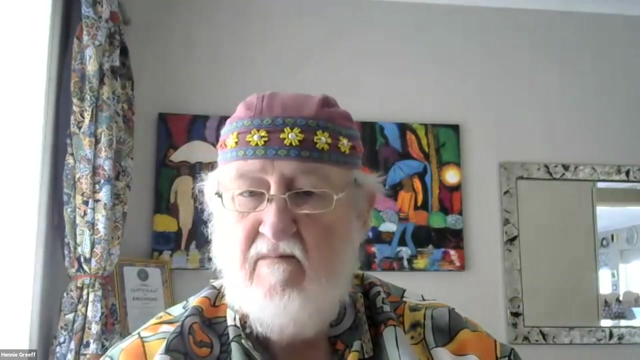 like we discussed here, And then, just on what Clive said, the City of Fairtown actually now employs two hydrogeologists, actual city employees, And I think they that's the first of its kind in South Africa. Yeah, it does help a lot with they have input into all various things. 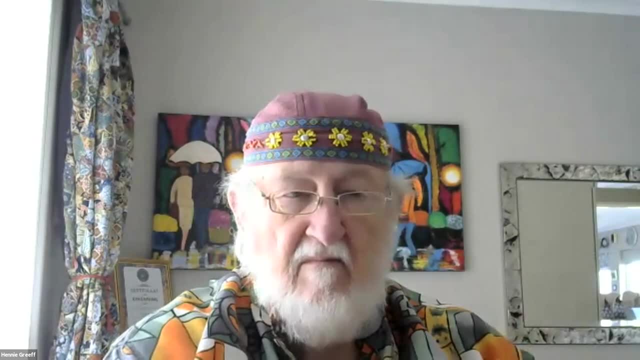 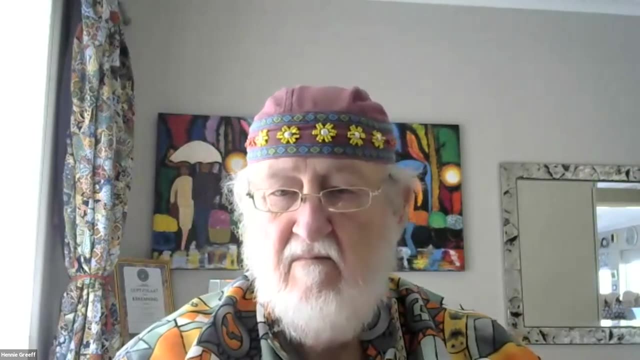 groundwater related, but also contamination et cetera, across all the various departments in the city, And I fully agree that that kind of stuff, geologists as well, and engineering geologists, that they should be appointed on a municipal basis. It would just make things a lot easier, I think. 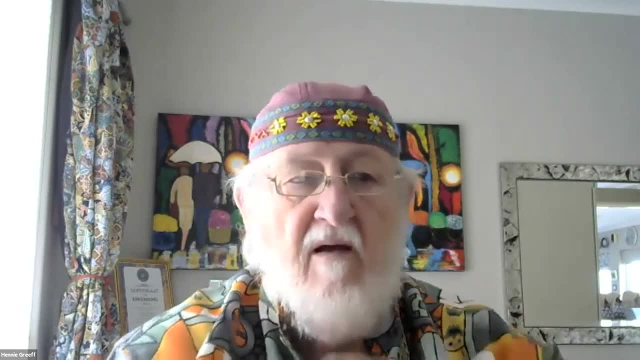 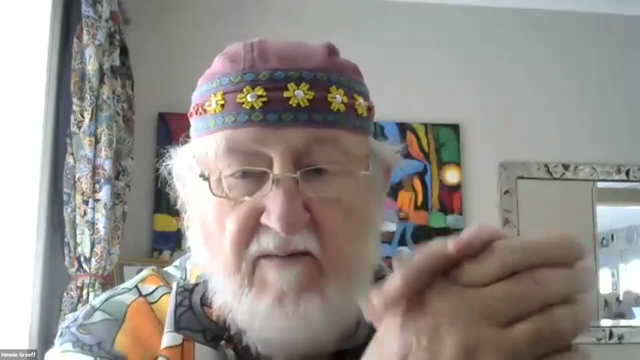 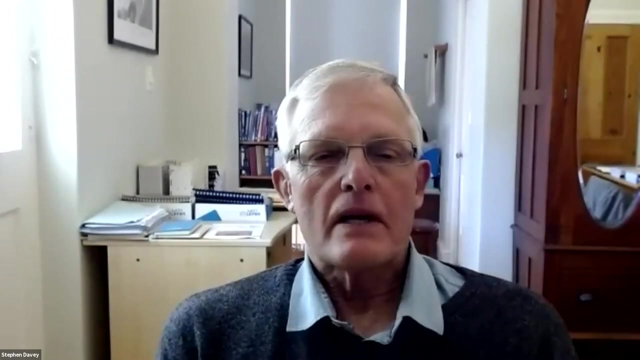 Yeah, Thanks, Dylan. There's a question from Julia Edelman for you, Stephen, asking that is the crushing and milling of stone to produce sand seen as too costly? Yeah, that is an option And Doug Cole actually mentioned it in the he wrote a Council for Geoscience. 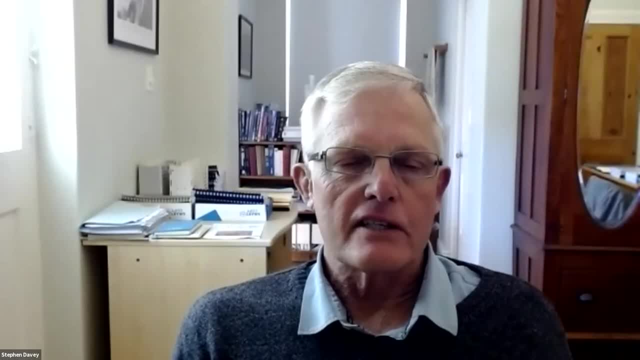 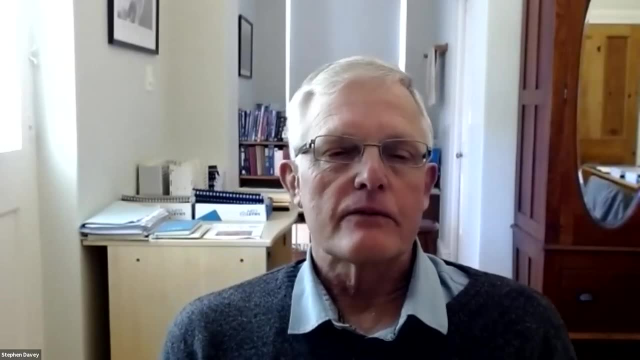 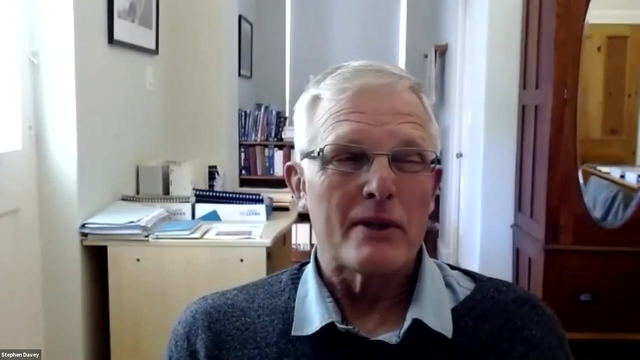 bulletin in about 2001 on the sand in the Western Cape. Yeah, And he said: eventually that is going to be an alternative that we've got to look at is manufacturing sand instead of just using natural sand. The thing is that at the moment, manufactured sand probably costs about four times as much. 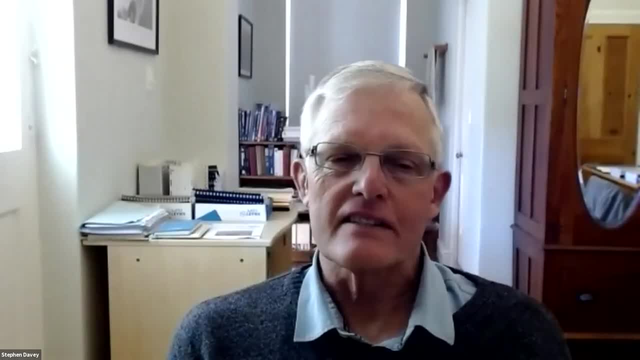 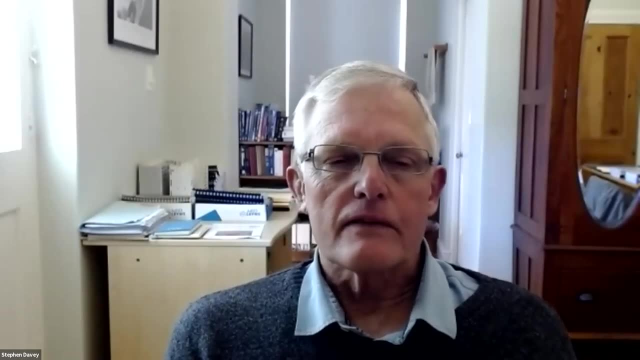 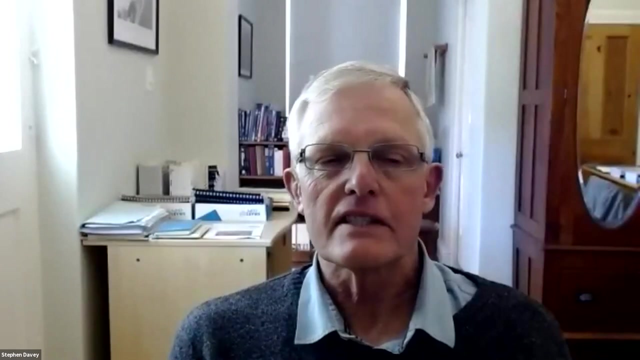 as natural sand. So obviously you know, if people have a choice they would still go for natural sand. But there is quite a lot of- they call it crusher dust from crushing plants That is used. It's used for making like concrete blocks and pavers and material like that. So material from crushing plants is being used as well at the moment, So it does help keep the natural sand too. To maybe just come in here on sand, I worked in Qatar for seven years and I couldn't believe that they actually import sand. 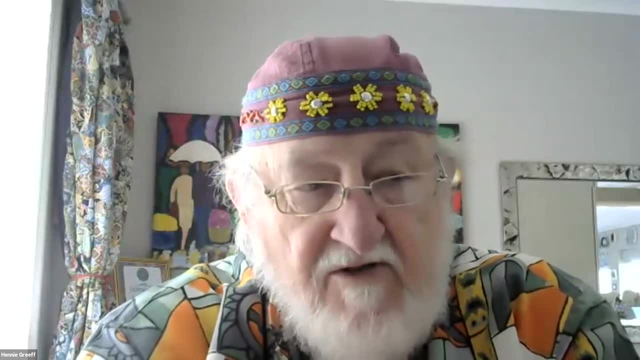 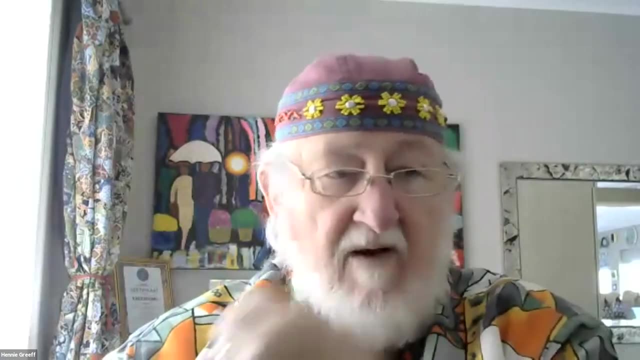 This is how far they go to protect their natural resources, So they wanted. they didn't want to use their own sand, so they buy sand cheaply from next door. It's just one of those things that you plan. well, you know you do things like that. 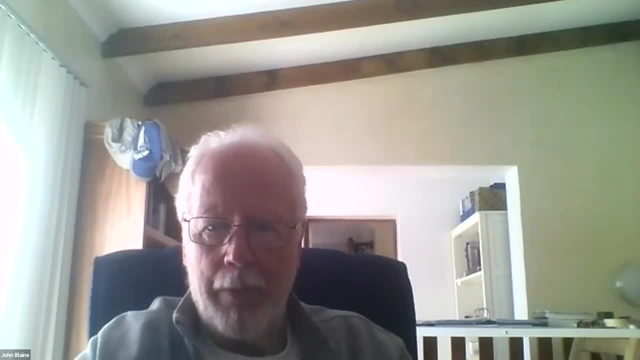 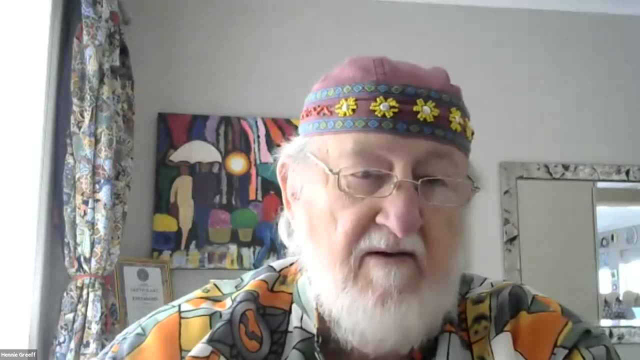 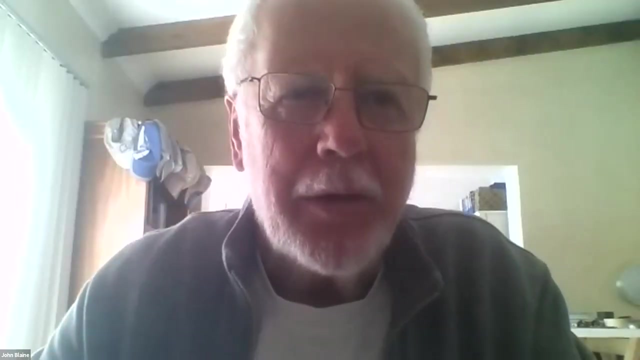 I am looking for volunteers to put together for us some kind of paper that we can forward. You guys are sitting there at home. Please think of something, John. you want to say something? Yeah, I think that maybe the one thing that you know. we all think of sand as sand, but 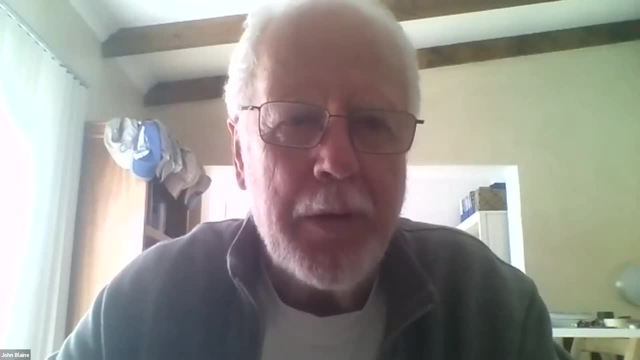 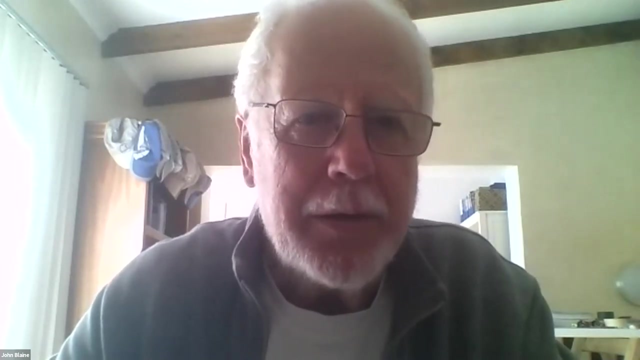 sand is not just sand. I mean, there's a big difference between river sand and beach sand, and it's not so much, you know, it's the granularity, but also the shape of the sand fragments. As I understand it, finely polished beach sand is generally not very useful for concrete. 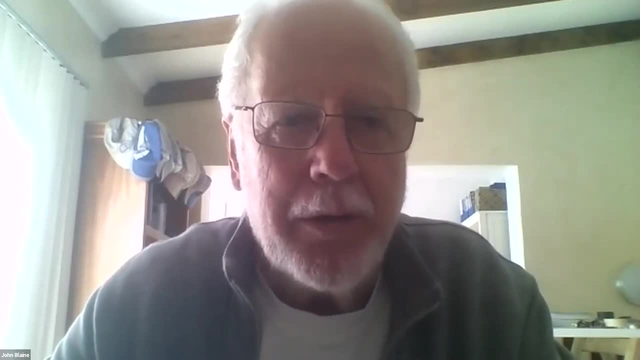 and cement, Maybe because it's got maybe a lot of limestone, other shell material and it's difficult to separate. But also windblown sands, I would imagine, are probably not very useful. Yeah, I would imagine are probably not as good as river sands. 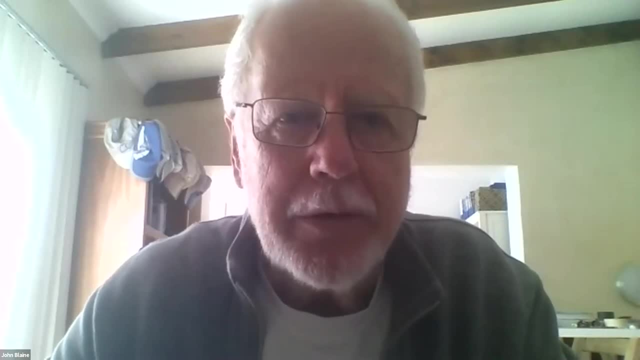 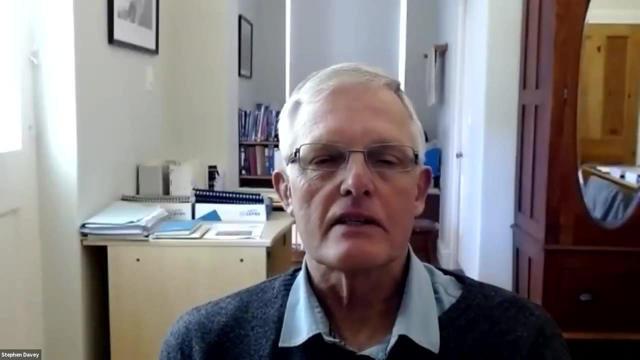 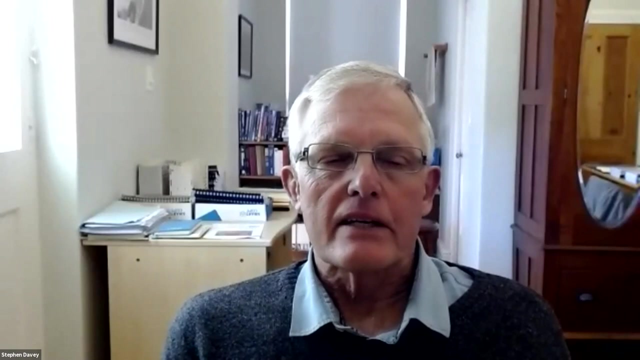 And so, Stephen, do those aspects come into it as well? Just the type of sand? how useful they are? Oh, definitely. There's a big difference between the different types of sand, And sometimes they even need to blend sand to make it comply with specifications as well. 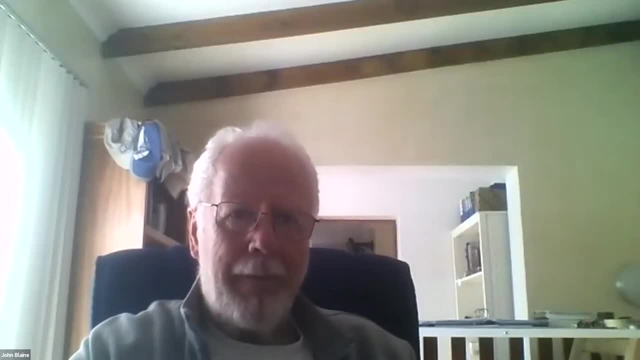 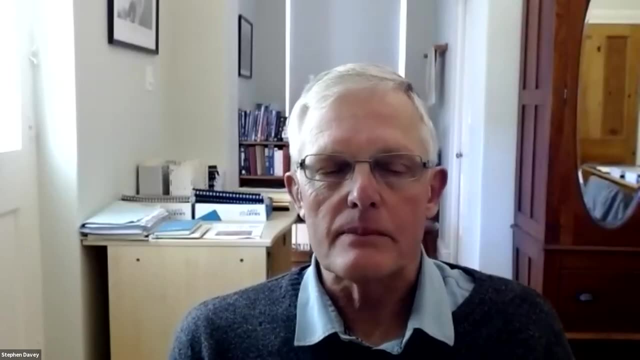 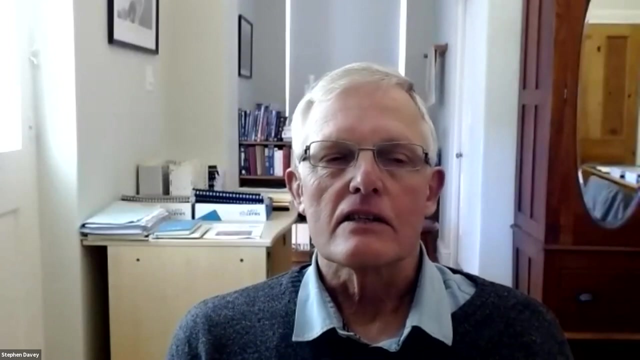 So you would find that the quality sand might be, you know, not as good. The sand might be not 100% suitable for concrete sand, but if you blend it with some of the Mammoth Beach type sand, then you can get a product that is really good for concrete. 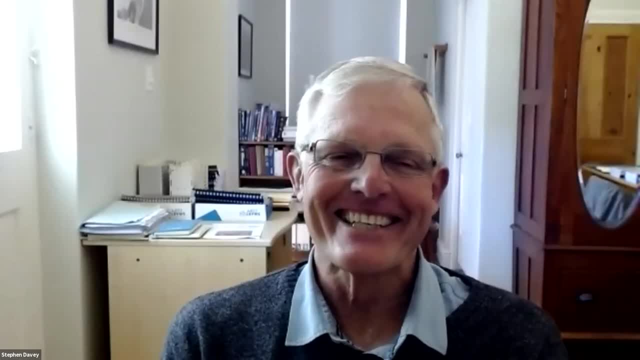 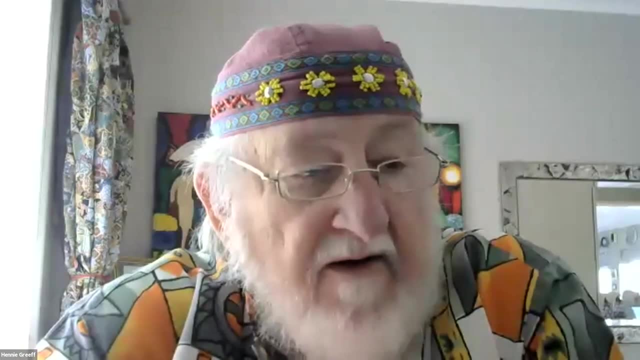 Thank you, No, no, no, Sand is not just sand. Yeah, Just for the layman amongst us. you know, the grading curve looks to try and obviate all the voids and minimize that to see the density of what you're going to produce at. 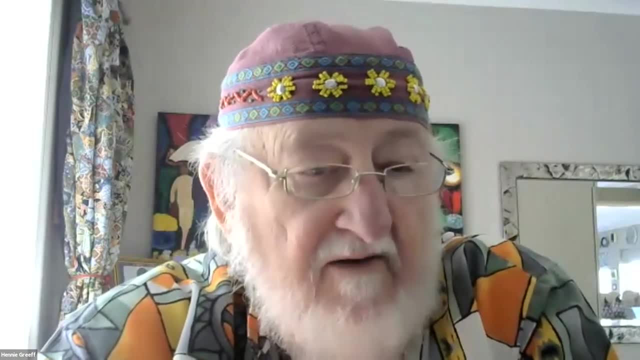 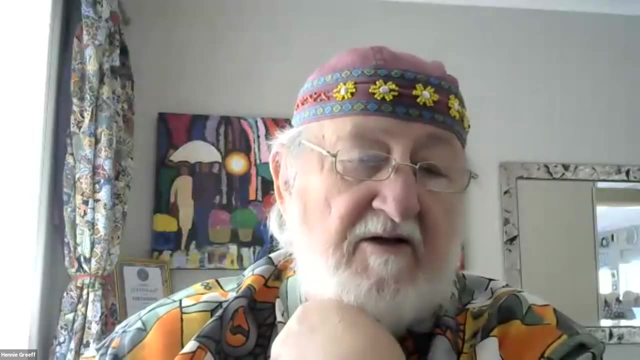 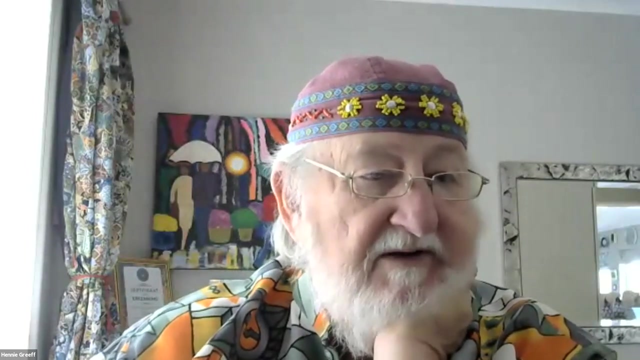 the end of it, And therefore some circular sands, leaves too much gap in the concrete. Therefore, you've got to design your ultimate strength. how long you're going to have the concrete Guys? any more questions at this point? John, your hand is still up, or is it the previous hand? 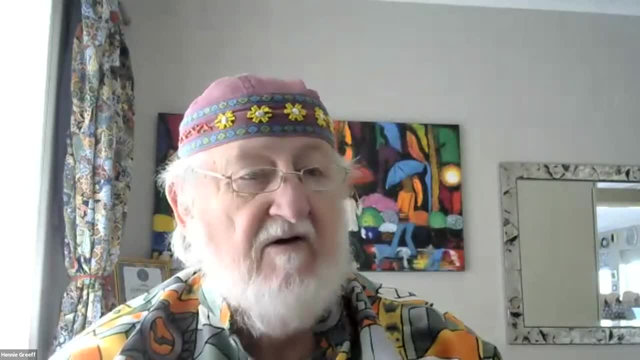 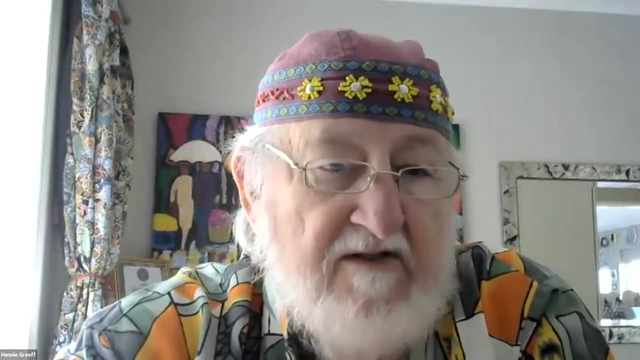 There we go. Thank you very much, guys. I think this was a very stimulating conversation, and it's not the end of it. We've certainly learned a lot of new things today. We've certainly learned a lot of new things. Thank you very much, Stephen, for doing this for us. 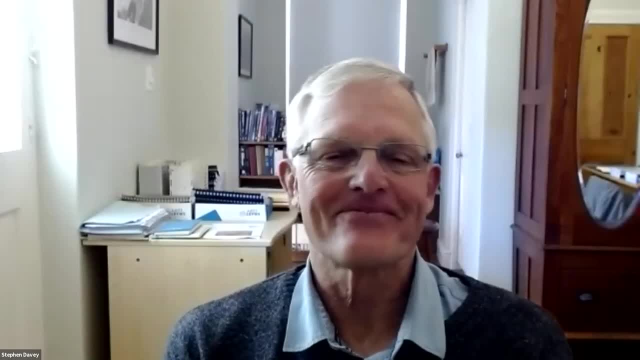 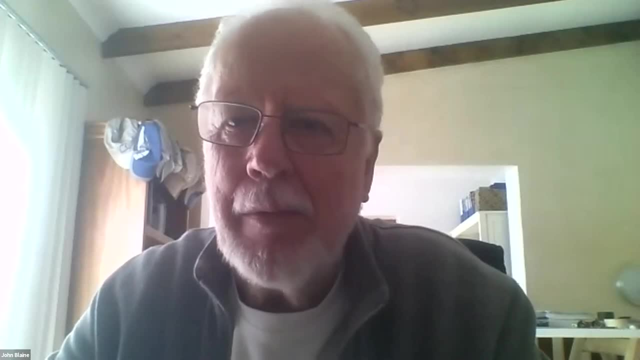 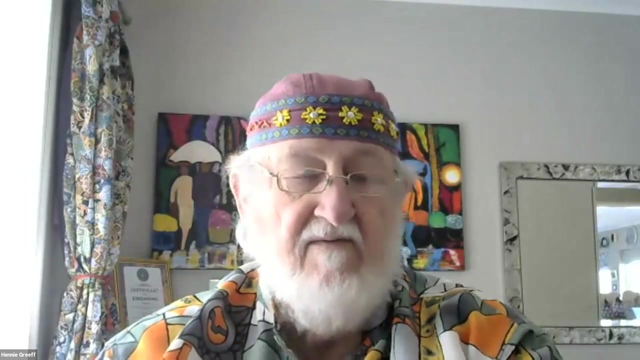 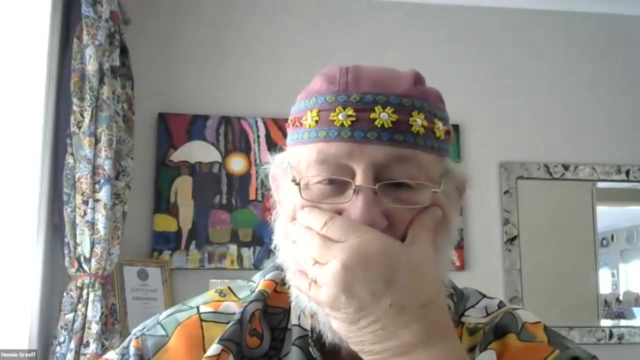 And guys, there's something that I can say. Yes, sorry, Can I talk Ferry Mark, sir John Carry on? Is it John or myself? Whoever speaks now? Okay, I just saw something there from Debbie. I suppose that is Debbie Abel from Durban. 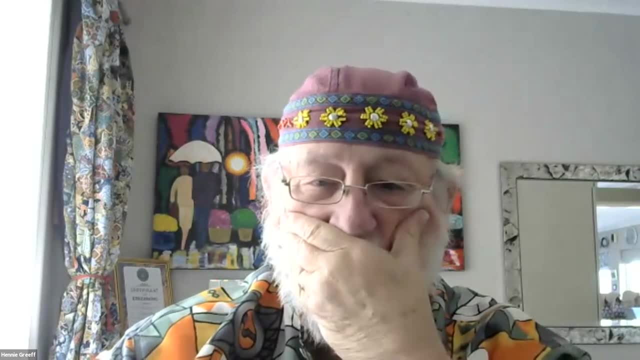 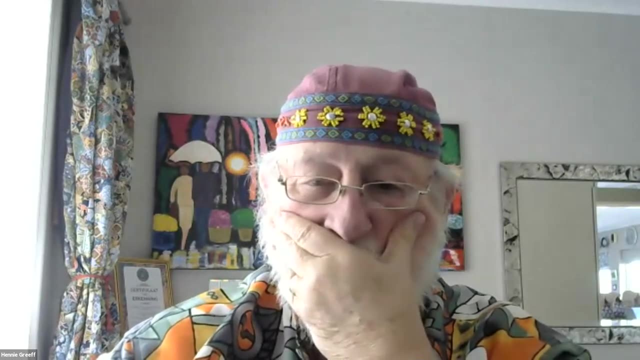 She just says that they've got an engineering geologist at the Queenie. That's quite correct. I mean, I know them all, starting from, I think, Tim Francis about 40 years ago, But that's about the only one that I know of and I don't know if they are appointed. 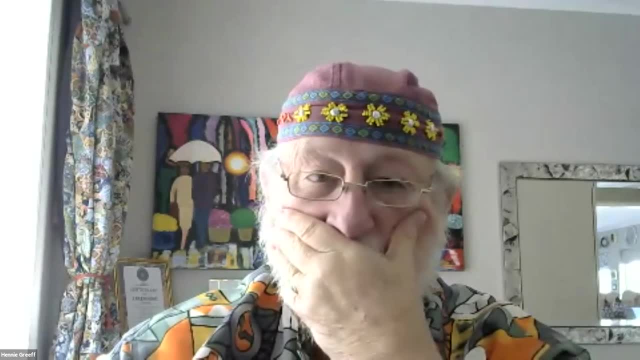 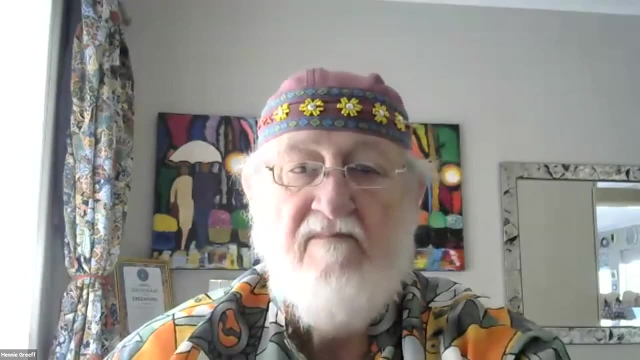 let's say according to the regulations of Council for Geoscience, because I would say that's about the only city that employs engineering geologists as such, And in Victoria, for example, or Tuani, we've got one there called Ashika Sudu. 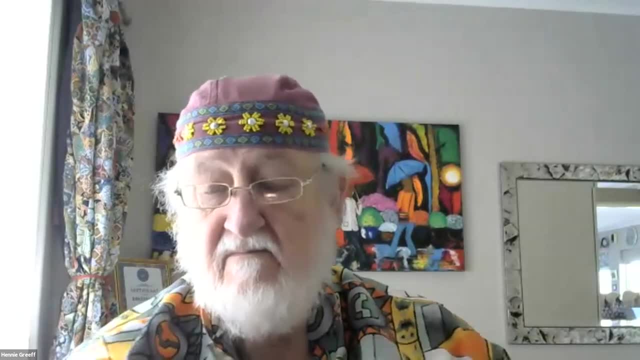 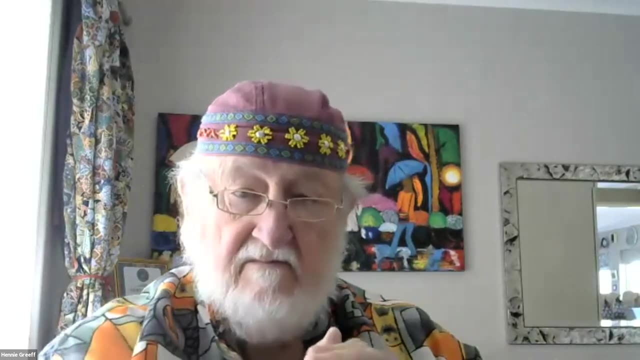 But I think Ashika Sudu is there under another sort of name, under, let's say, a geotechnical officer or something like that, not as a geologist, you know, per se. So yeah, so that's just the answer on, you know, on that one. 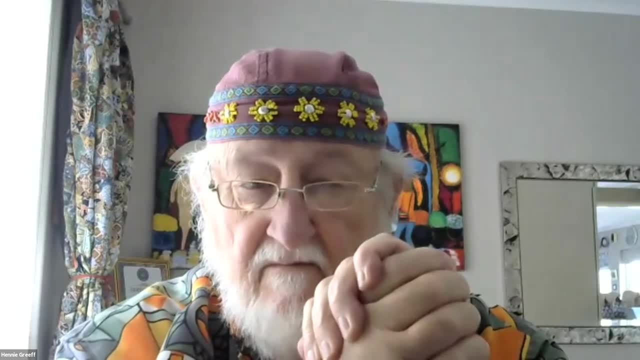 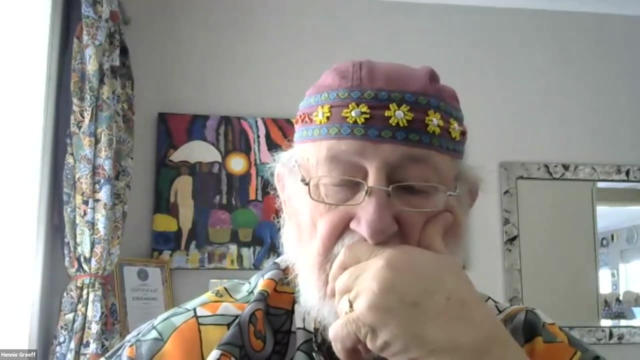 I think that's the other thing that I would like to ask Stephen, if possible, because I'm quite interested in that- is: what is the main source of crushed Yeah? Yeah, Also nice to see one guy that I know, Peter, but from previously from Water. 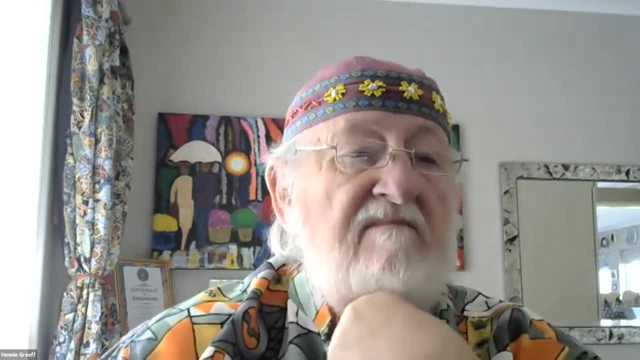 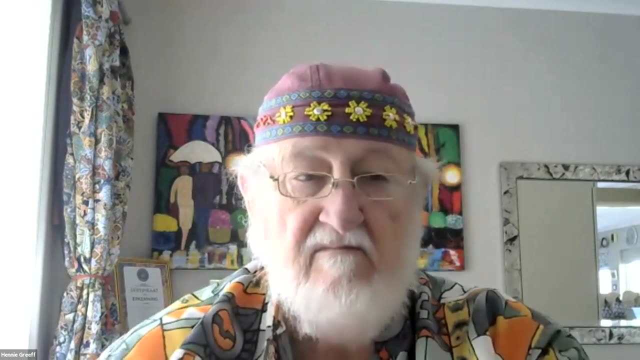 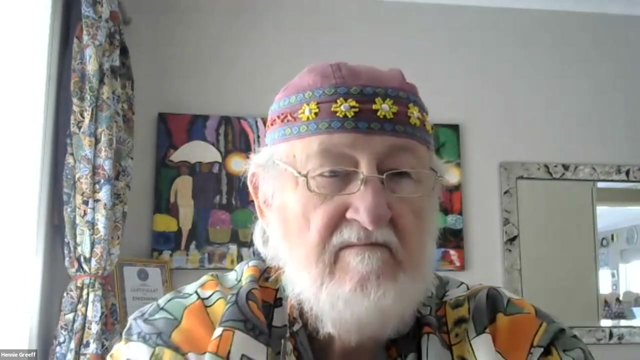 Affairs. But what is the main source of, let's say, crushed aggregate, coarse crushed aggregate, in the sort of Western Cape, Western Cape area? Is it Table Mountain sandstone, or is the Table Mountain sandstone generally too soft? or what have happened to the Malmesbury on-fells? or 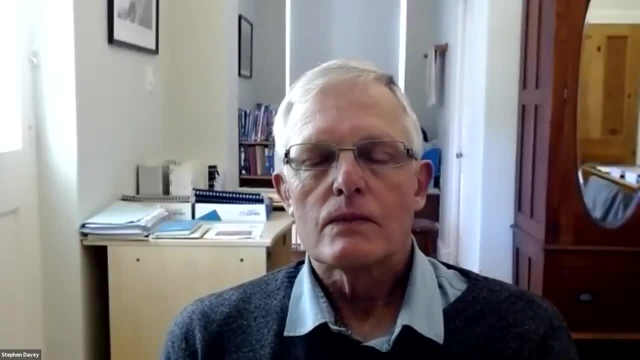 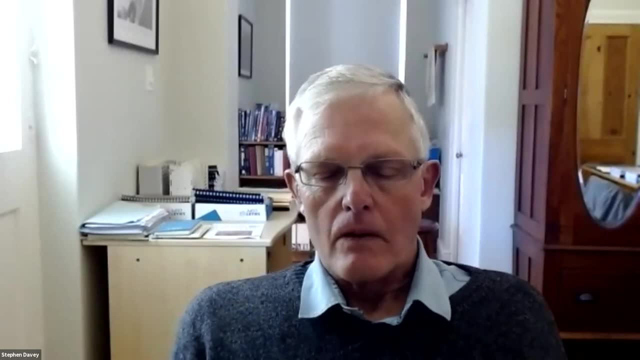 No, no, I don't think so, Because that used to have the problem with the alkali aggregate reaction. Just, perhaps if anyone knows something about that, you know, I'd be interested. Yeah, In Cape Town the main source is Malmesbury on-fells. 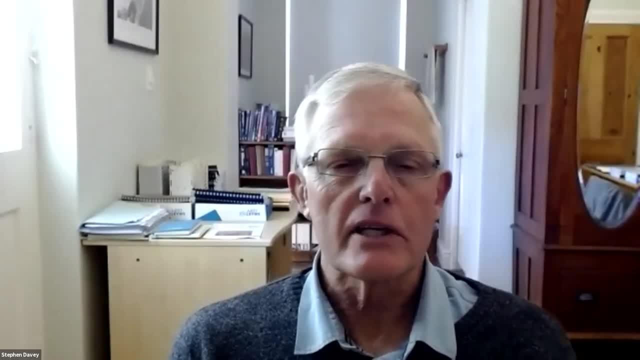 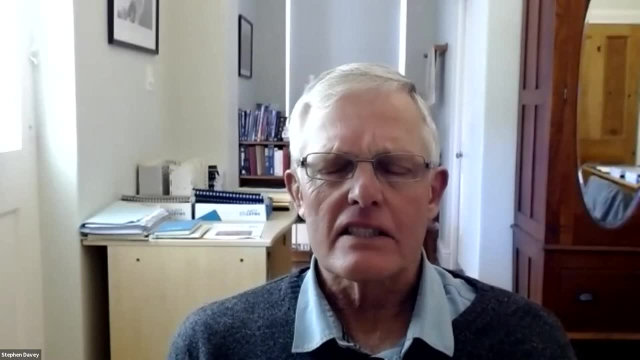 There's a whole series of quarries around the Tiger Big Hills and Ephraimette and Lafarge and private company Chirley Brothers. They're all around the Tiger Big Hills, tiger hills that those are, so that for cape town itself that is the main source going up to sodana. 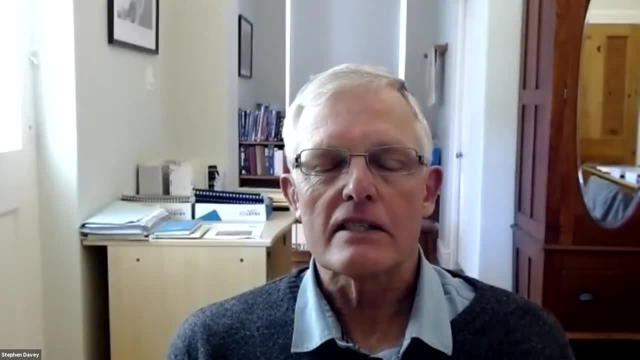 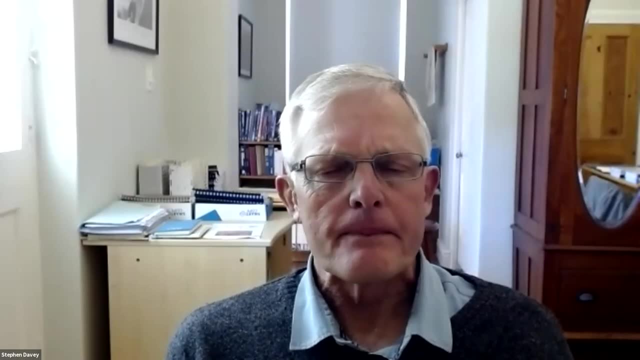 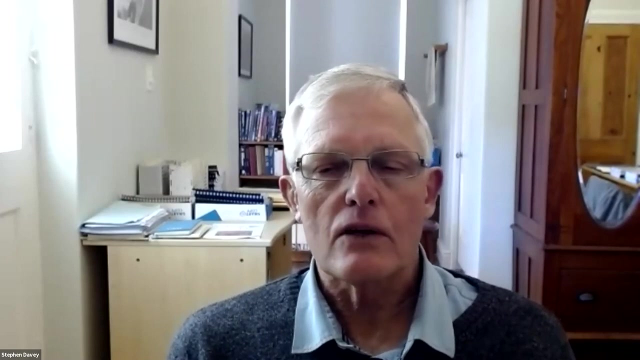 bay. it's small granite, cape granite, and then i think there's a table mounted sandstone quarry in grabo and um, going along the garden route, um table mountain sandstone in uh in flittenberg bay, and then there are quite a few quarries that are crushing uh enon conglomerate, um sort of like. 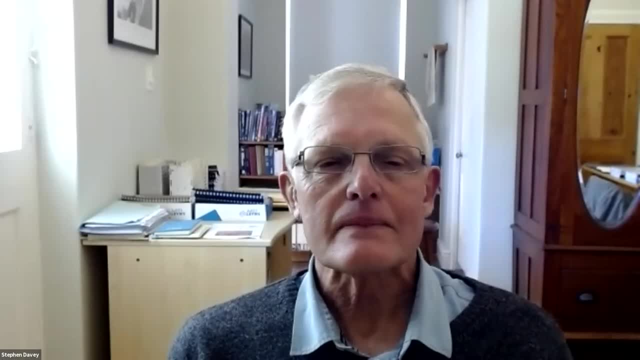 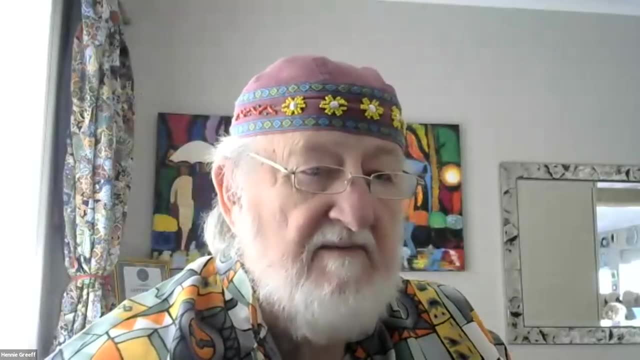 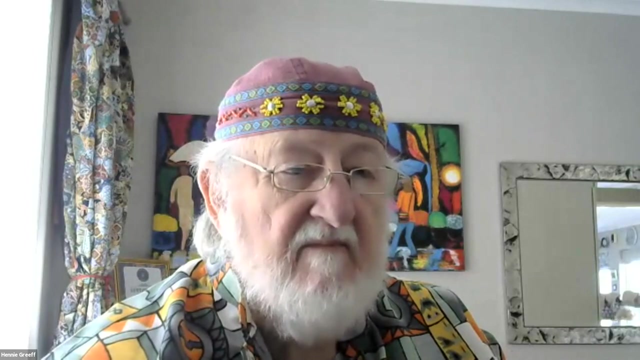 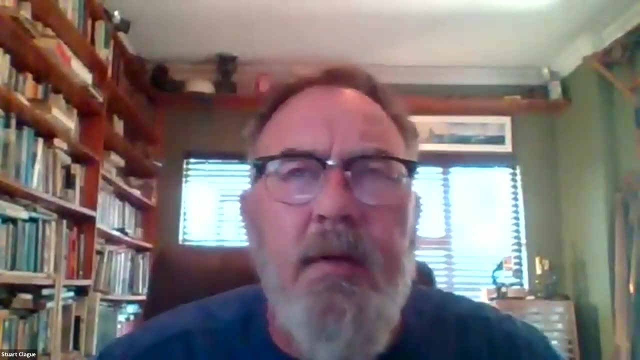 muscle by hartenbusch area. yeah uh, stuart clay, you can unmute yourself. stuart stuart, you got your hand up here i am. yeah, okay, here i am. um, yes, talking about quarries, i was wondering about the potential for ornamental stone with the cape granite. 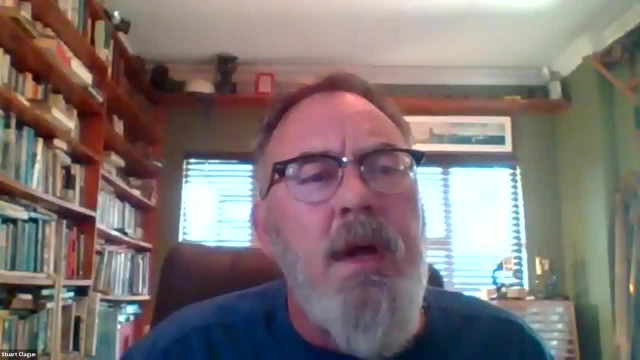 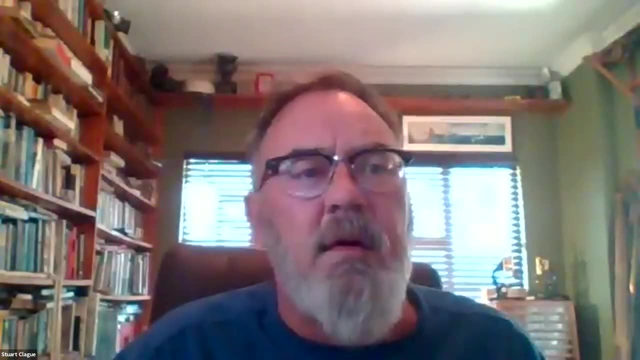 i can't think of any ornamental stone quarry or sales of cape granite, as all ornamental stone, most of the ornamental stone for kitchen tops and so on that we find is is imported or it's from the bush felt, the so-called rostenberg granite, which is gabbro on all right. 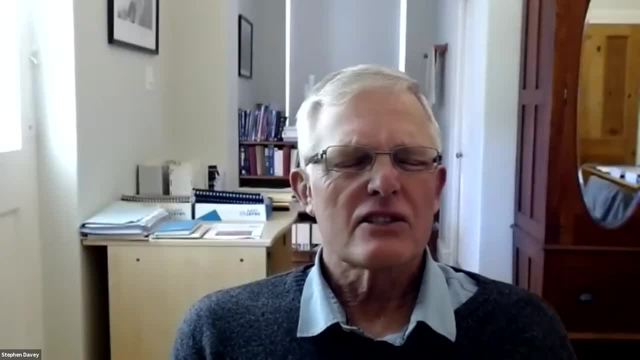 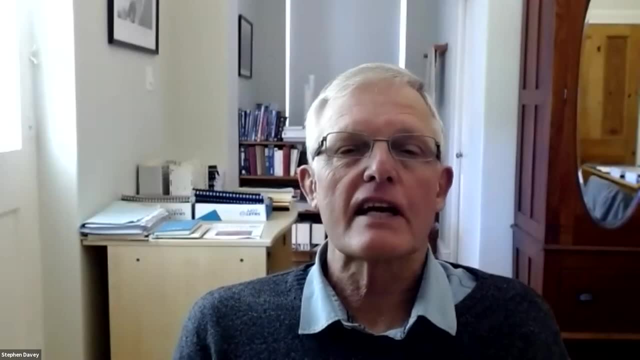 oh, there's, there's one on the power granite. i think it's called flip query or something like that. i can find the reference to it. and then there is also dimensions down that come from the northern cave. um, but yeah, i're not pretty much in the western. 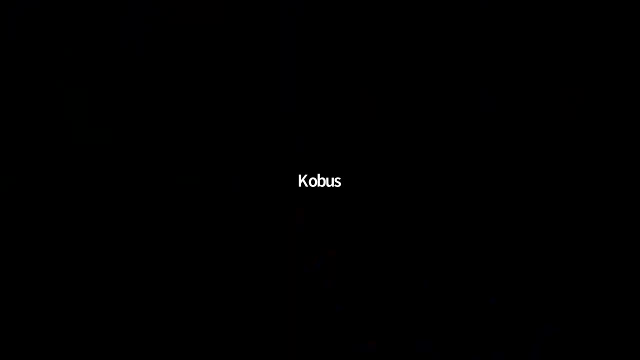 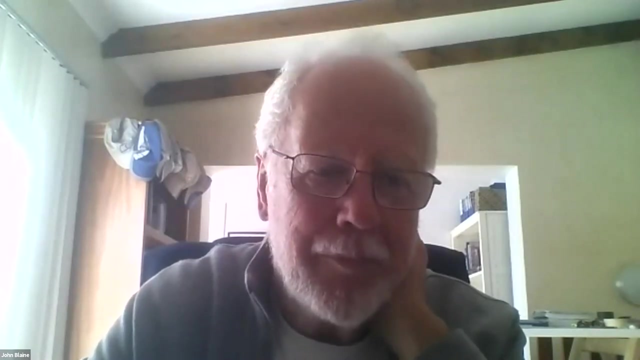 if i could just ask me something. uh, yeah, okay, what happened to that? uh, i used i actually went to school at financial up to standard six or what- now grade eight, and long after I left they opened apparently a marble quarry between Van Rensdorp and Vredendal. Is that for Dimension Stone or is that for some other purpose?